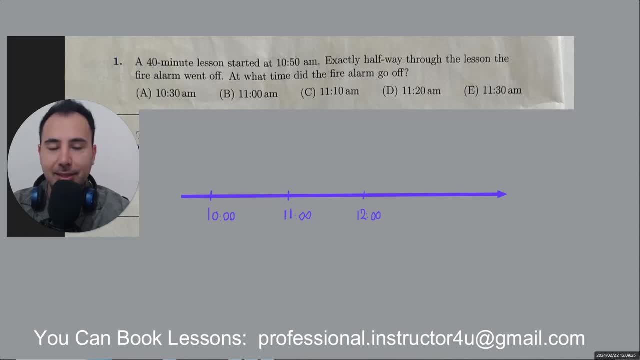 remember. you don't have to draw this in the test. I just want you to visualize this when you do a question like this. Probably this one is easy. You don't have to, but you just need to visualize something like this for all questions regarding time. So let's read this one: A 40 minute lesson. 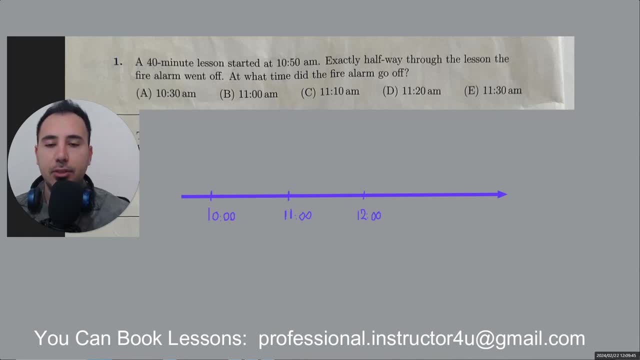 started at 10: 50 am. So this is the start. You have to visualize this. It's going to be just here. It's going to be 10: 50.. How many minutes before it becomes 11 o'clock? You have to answer that question. like 10 minutes later it's going to be 11.. Exactly halfway through. 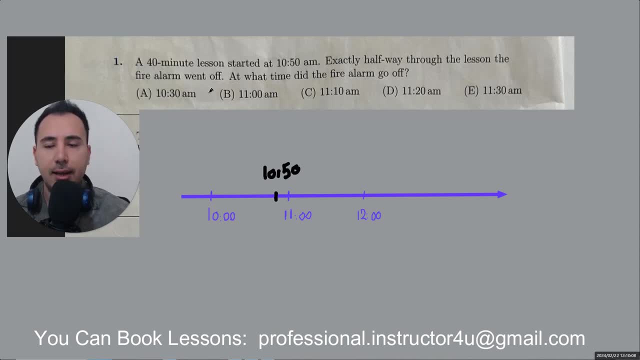 the lesson, the. oh, the fire alarm went off. So this is 40 minutes. Half of it is 20 minutes. So 20 minutes later, at what time did the fire alarm? okay, go off. So we're just visualizing this. 10 minutes later it's 11 o'clock, 10 minutes more 11: 10.. So it's going to be like this: okay, 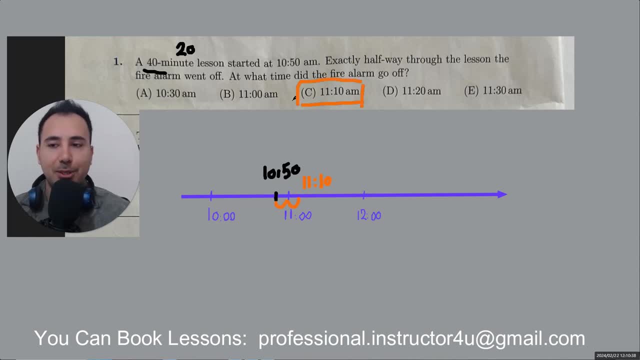 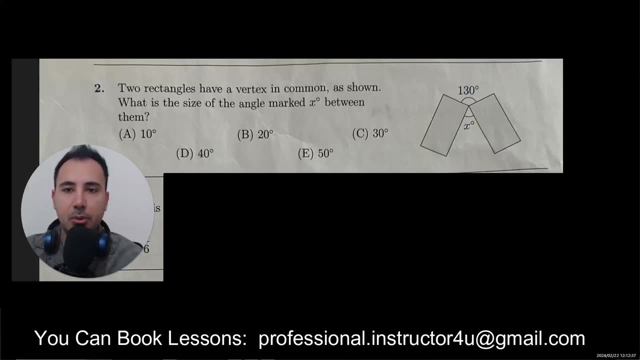 See this question. maybe you can answer it without visualizing it, but this will help, Okay. Okay, let's do a problem too. Two rectangles have a vertex in common. Okay, We know that vertex means a point, So it's going to be this point. These two rectangles have this point in. 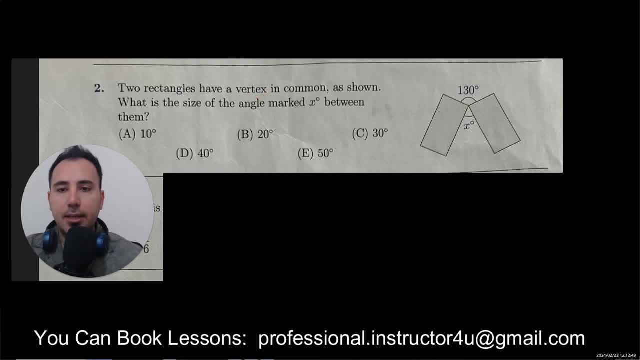 common as shown. What is the size of the angle marked x between them? Okay, So I think it's important to answer the question by just looking, But let me explain. See, when we go a full circle from here all the way and come back to the point I began, Okay, What is the angle? I traveled The 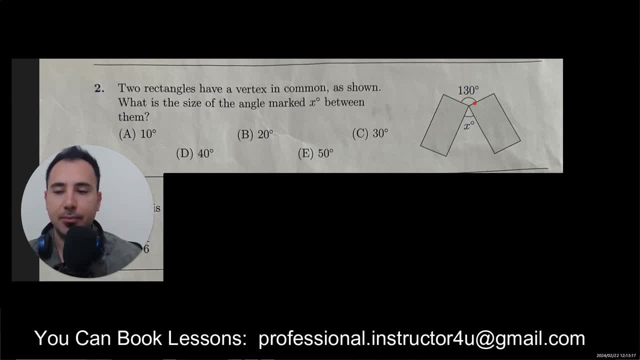 angle of a circle of full round is 360 degrees, Right, So let's go. This is a 90 degree angle, So I'm going to write it here: 90 degree angle, And then I go a 130 degree angle. 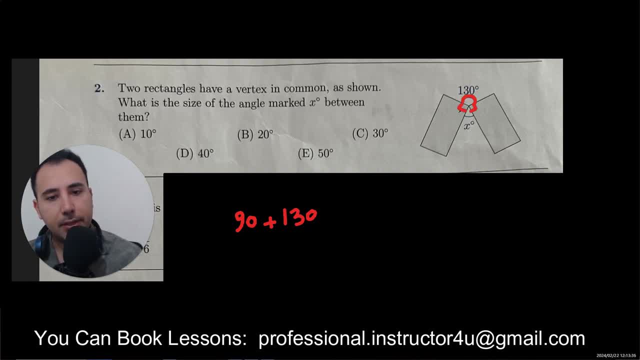 And then I go another 90 degree angle from here to here plus 90 degree angle And finally, Okay. So if I go this x degree, that's going to be a full circle. a full circle is 360 degrees. Okay. So if I go this x degree, that's going to be a full circle is 360 degrees. Okay So. 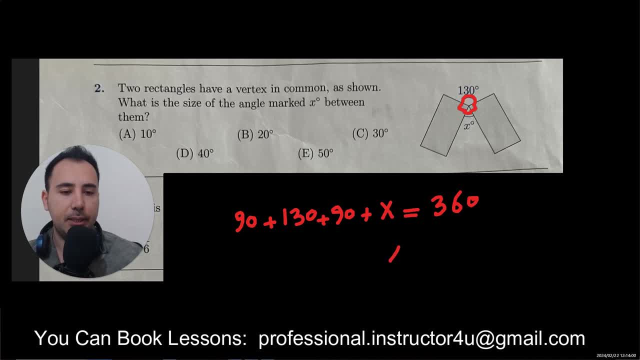 you simplify this. Okay, x will actually give b 50. Right? So if you want to be fast, you're going to be like this: 1990- 180. So 360 minus 180 is 180.. So 130 plus x is 180.. So that's how I know. 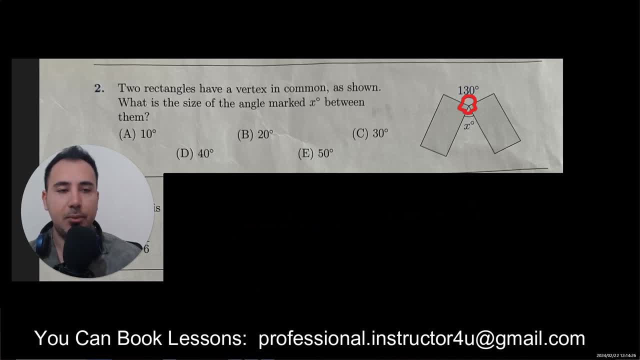 Okay. So, even in the picture, See, I will be like: Okay. So even in the picture, See, I will be like like okay, that's going to be a full circle. these two subtracted from a full circle, 180 degrees remaining 130 plus which number is 180, it gives me 50. i could do this two seconds, three seconds. 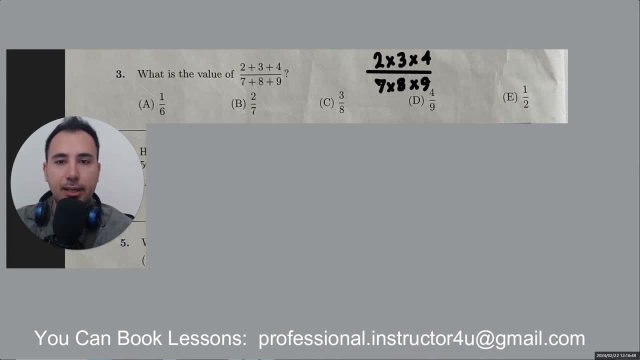 the only way somebody can get problem three wrong is, uh, confusing these two expressions, right? so see, when i have these two and i'm multiplying them, i can simplify them. so i could go. this tree cancels by this: okay, this 4 becomes 1. this 8 becomes 2. okay, and this 2 again. 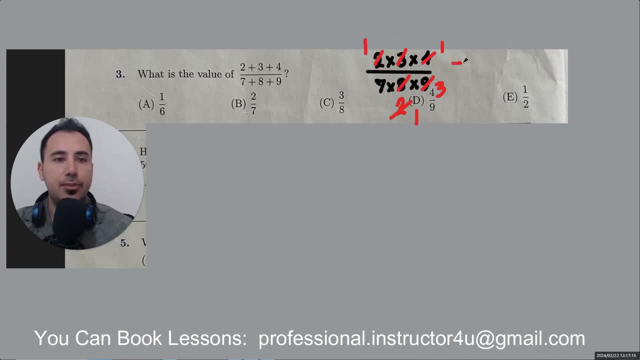 cancels with this 2, so the answer to this will become 1 over 21.. i get the cancel and simplify, but can I do this when I'm adding the numbers? can I go 3 and 9? you can't do that right. so when we are multiplying, we can simplify. when we 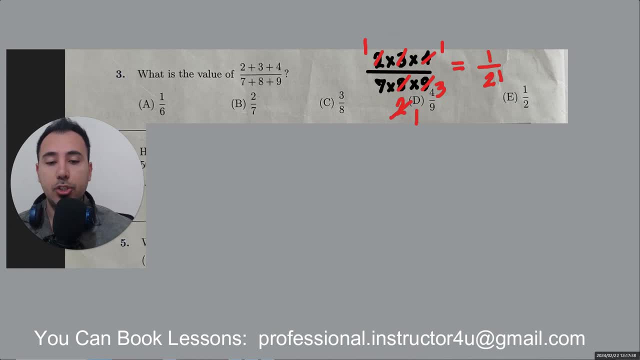 are adding them no way, so you just have to add them first and then divide. so let's go here: 2 plus 3 plus 4 is 9. ok, so 7 and 8, 15 plus 9, 24. do we have this number here? no, why not not simplify? both of these could be. 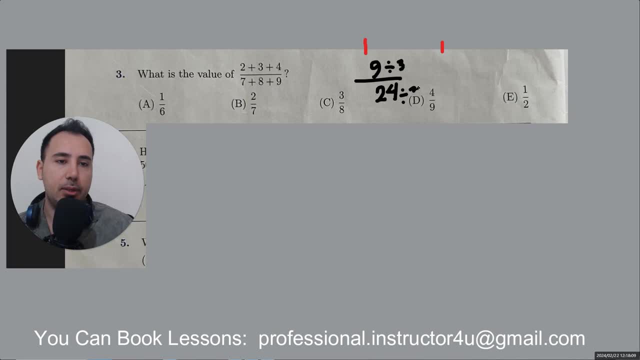 simplified by 3, and so let's go and do that. it's gonna be 3 over 8. so let's go and do that. it's gonna be 3 over 8. so let's go and do that. it's gonna be 3 over 8. 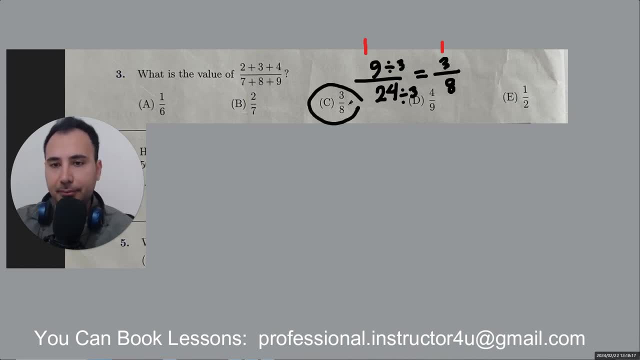 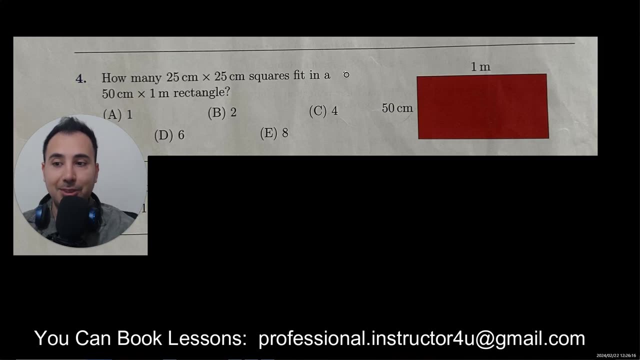 so C is the right choice. problem four is really important because if you do it the right way, it's gonna take a few seconds. if you do it the wrong way, maybe it's gonna take two or three minutes of your time, and you can make a mistake too. 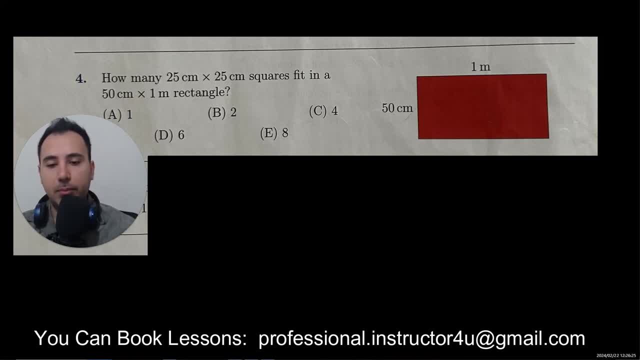 so the wrong way would be to find the total area of this, okay, and then find the total area of that, and then you would go: okay, this big area divided by this will give me the number of squares that's gonna fit. that's really bad, let me see. 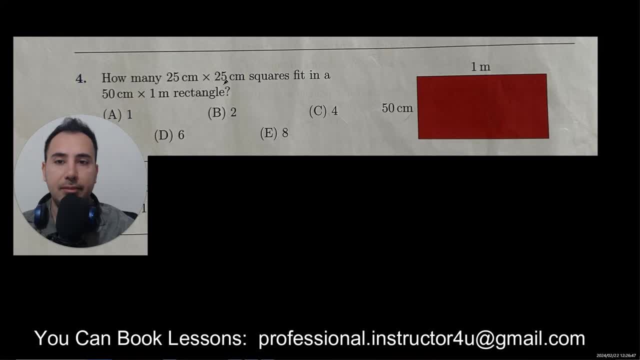 let me tell you why. how many 25 by 25 centimeters square fit in a this rectangle. see, you just need to draw one of these. first right: 50 is 225, so I'm going to draw one of these. first right: 50 is 225, so I'm going to draw one of. 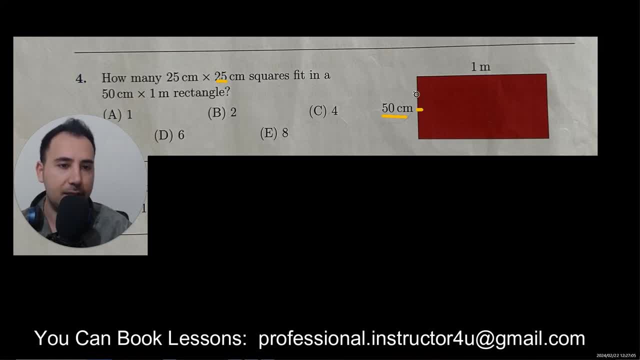 So I'm going to draw one of these. first right, 50 is 225, so I'm going to draw divided into half. see, this is now 25, this is 25, this is 25 and a 25 by 25. it looks something like this: now you have to tell me one meter is how many 25. 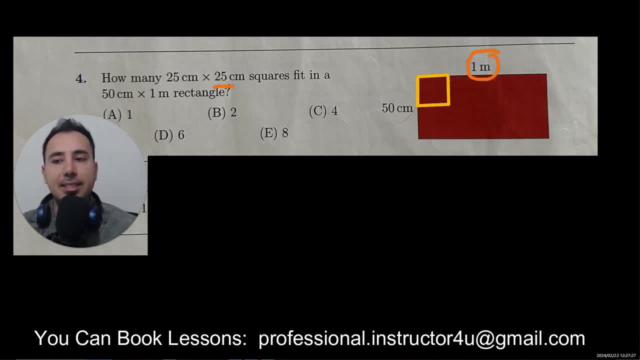 centimeters. one meter is a hundred centimeters, 25 centimeters, so centimeters. so 25 centimeters. one meter is a hundred centimeters, so 25 centimeters. one meter is a hundred centimeters, so 25 centimeters. one meter is a hundred centimeters, so 25 becomes 100 meters. so 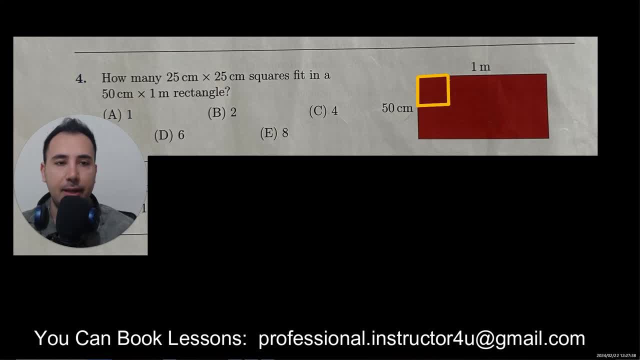 25 becomes 100 meters. so 25 becomes 100 meters. so the question is over. you don't even have to. the question is over. you don't even have to. the question is over. you don't even have to draw it. so if this is, if this is 25. 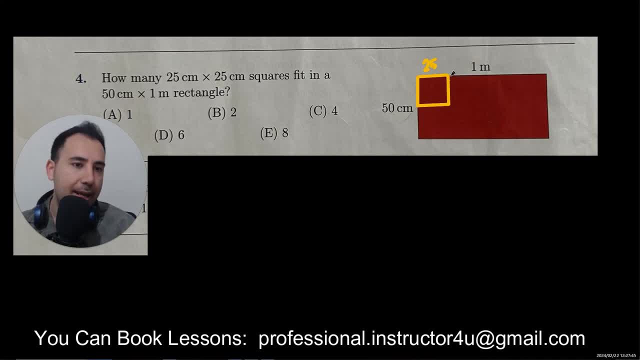 draw it. so if this is, if this is 25, draw it. so if this is, if this is 25 centimeter as well, since this is square centimeter as well, since this is square centimeter as well, since this is square, and then you will have another 25. 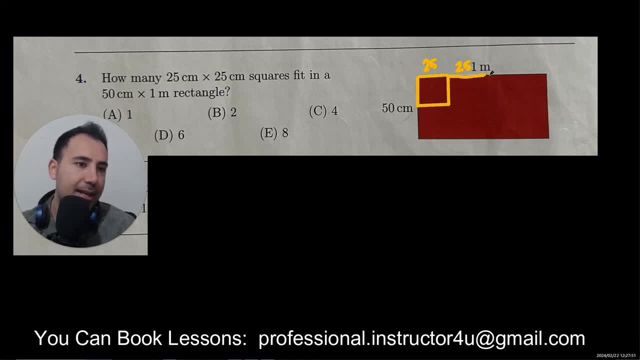 and then you will have another 25, and then you will have another 25 centimeters it's gonna be half, and then centimeters it's gonna be half, and then centimeters it's gonna be half, and then again another 25, and then another 25 do. 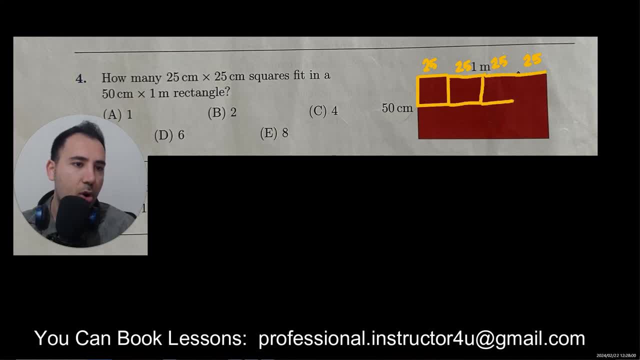 again another 25, and then another 25. do you have to draw it all in the test? no, I'm just drawing it to show you. okay, so this is four, and they're gonna be four here as well, so it's just gonna be eight. you do it like this, you see it. you could even do it like in three or four or five. 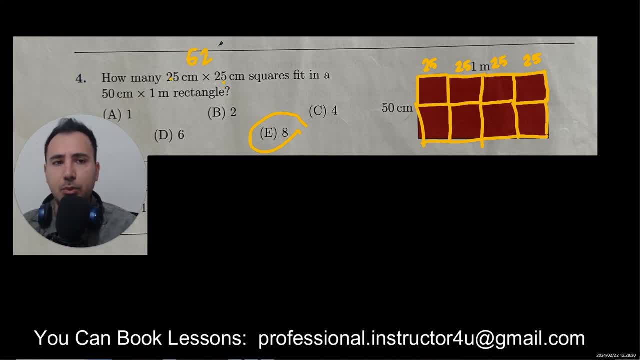 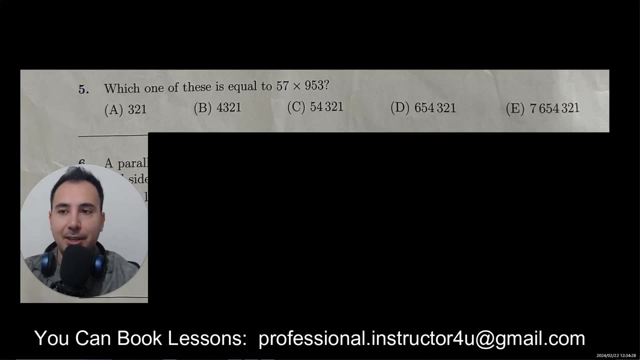 seconds. you multiply this. this is gonna be 625, and then you multiply this. ooh right, you don't want to do that for problem five. I have had some of my best students, smartest students, doing problem five the wrong way. they would go okay. so I have to multiply these two numbers and then one of them is the answer. is that a? 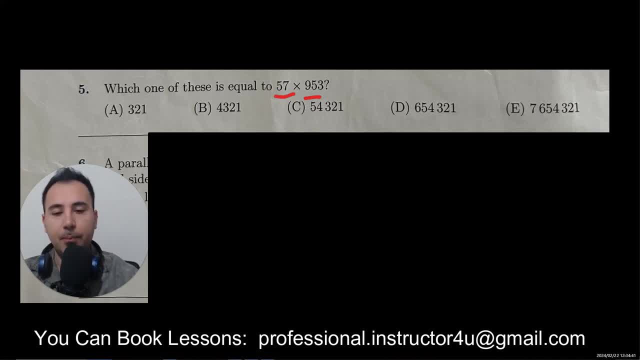 good idea. no, that's horrible because it's gonna take a little time, right. so you see that this is a problem. approximately seven to eight million. this is six hundred thousand. okay, sixty hundred six thousand six hundred, right. so the differences are huge. so then we could just do an approximation. 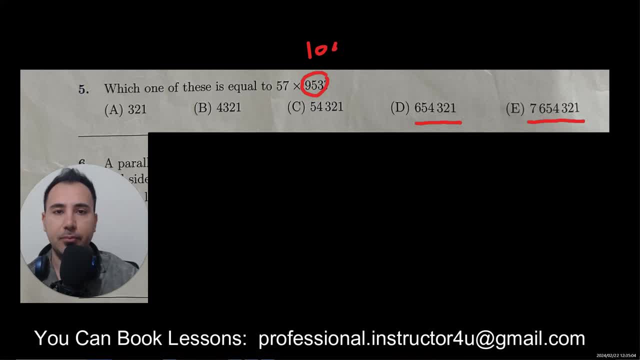 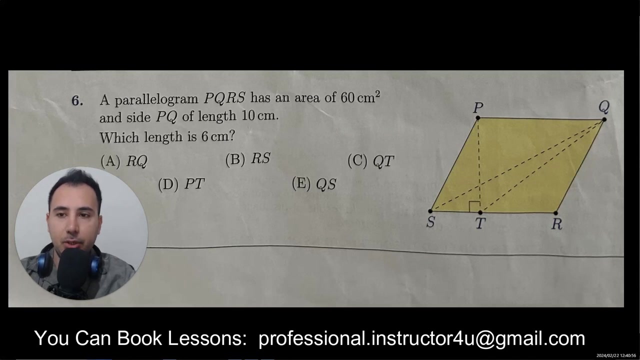 this is close to a thousand, this is close to sixty, so we multiply them, it's going to be a six with four zeros. six and four zeros looks like this one right, so C is the right choice. don't waste time again. if you know how to find the area of a parallelogram, maybe you could answer this. 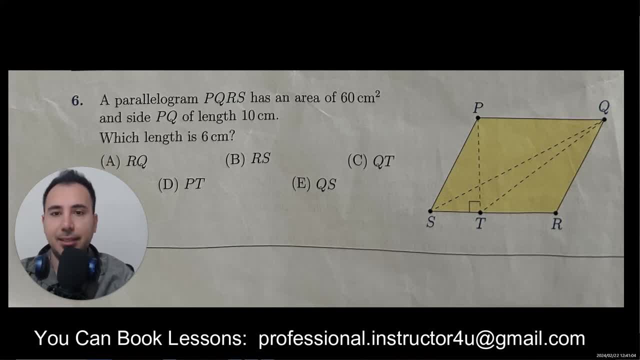 question just by looking, maybe ten seconds is enough. let's read the question. a parallelogram: PQ RS has an area of 60 centimeters and the PQ of length 10. they have given you this is 10. okay, which length is six. so basically do. 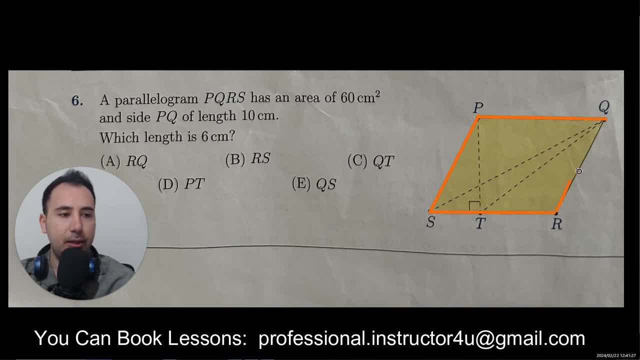 you know how to find the area of this parallelogram, do you see? all you have to do is just cut this piece, the blue piece, and add it here. so then the parallelogram turns into a rectangle. so the area of a parallelogram and the corresponding 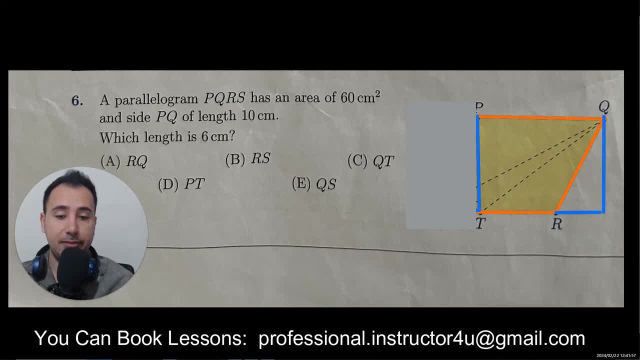 rectangle are equal, so how do you find the area of this rectangle? PQ is 10, the area is 60, so the blue side is. well, this is how large is this actually? 6, okay, but we know that this area of rectangle and the area of this 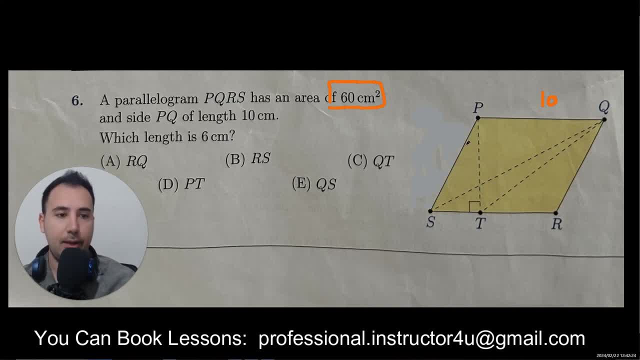 parallelogram or equal. so that means to find the area of the parallelogram you just have to multiply 10 by 6, so parallelogram is 60. obviously this is 10, so this is 6. so where is PT? PT is here. D is the right choice if you can't do. 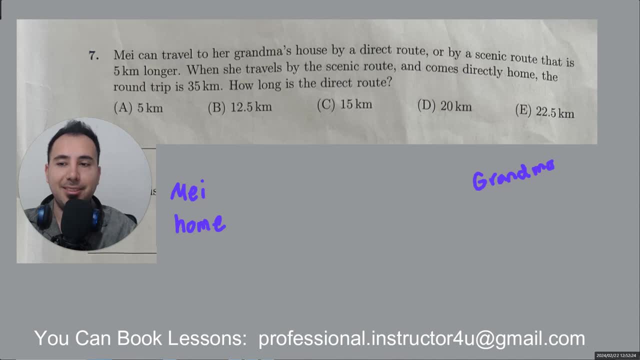 problem 7. you're overthinking the problem. there is no other explanation. so let's see. and again, I'm going to draw a diagram, but you don't have to draw it in the test, you just have to visualize this. right, this is your mental image. may can. 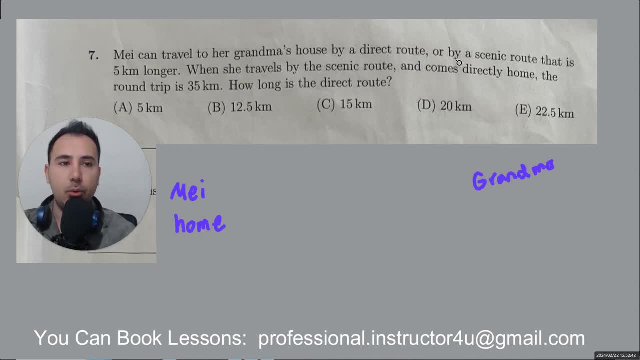 travel to hand grandma's house by a direct route or by a scenic route that is five kilometers of longer. so there are two routes. if you go directly, it's shorter. you could also go a little longer. okay, when she travels by the scenic route and comes. okay, a scenic route that is five kilometers longer. 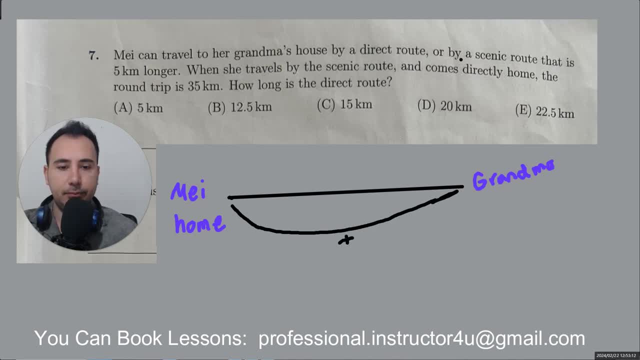 okay, when she travels by the scenic route and comes. okay, a scenic route, that is. so this one gets up plus five. okay. so when she travels by the scenic route and comes directly home, the round trip is 35 kilometers. how long is the direct route? okay, so she's gonna travel from here to here and then come back directly and the 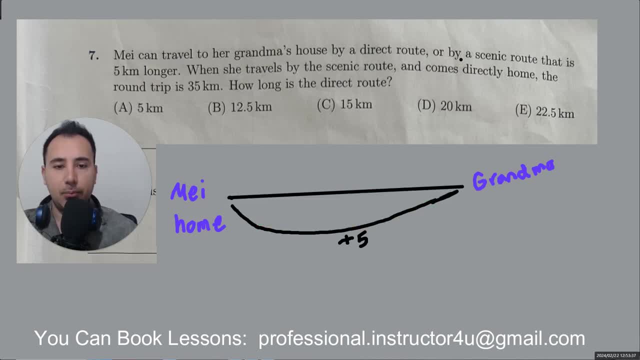 total is 35. okay, so here no equation is nothing. so you just pick a direct route. so for example, which one? I'm gonna pick? 20. if 20 is my direct route, then my longer route will be 25. so if I go from here to here, I go to grandma, 25 and I come back 20, that's gonna be 45, but we 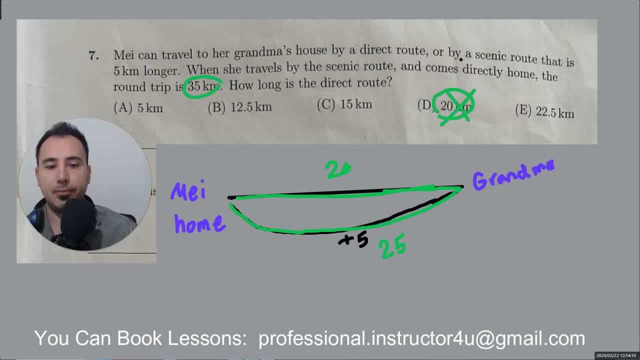 want the answer to be 35, so this is out right. so that's it. see, you could- even i- i'm pretty sure a lot of you already figured out the answer, so let's just try it with 15. if the direct route is 15, the scenic route is 20. so again, we're gonna go with scenic route 20 and come back 15. it's gonna. 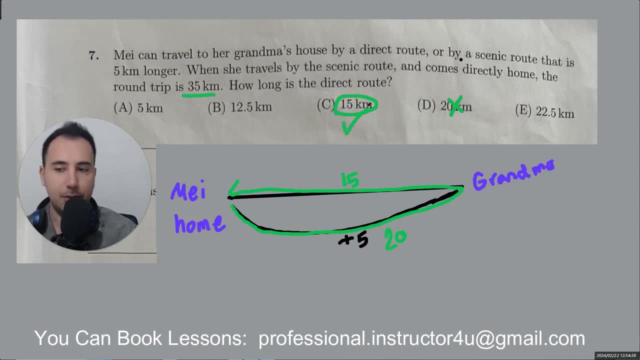 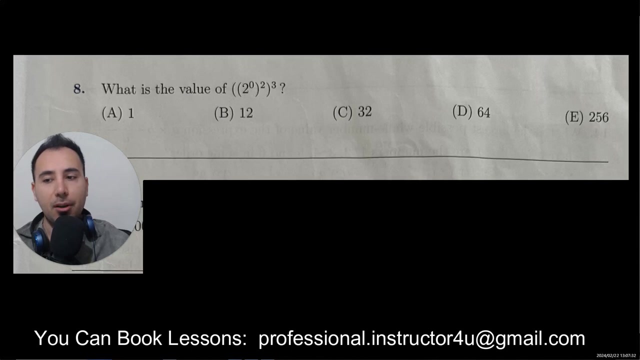 be 35, which is this one. so this is the right choice. i told you, if you can't answer this, you're overthinking the problem. okay, there are two ways to get problem eight wrong. okay, so if you get this wrong, probably most likely you're getting the either one of these things wrong. so what is two? 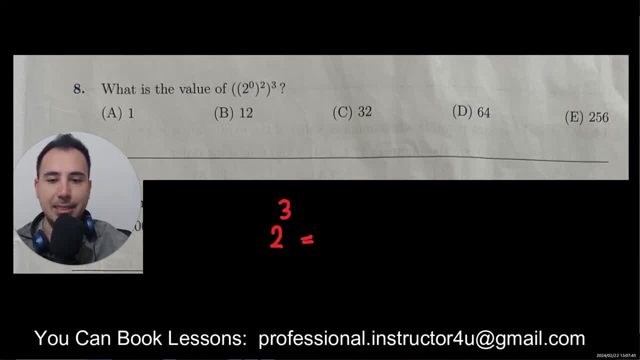 to power of three. are you going to tell me it's six or it's actually eight? see, if you think it's six, or sometimes you confuse these with multiply. that could be one reason that you could get similar questions or this one wrong. so two to power of three is two times two times two, which is eight. okay, 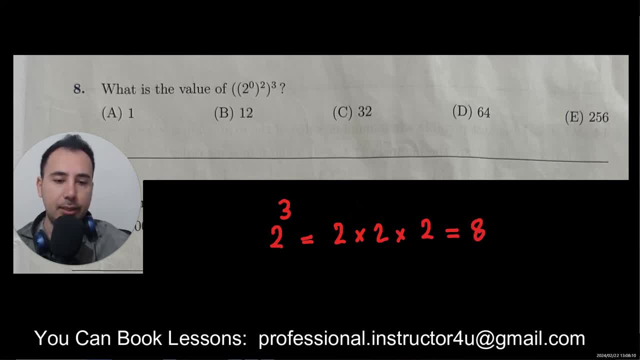 and one other thing is two to power of any number. so two to power of zero is actually one. one to power of zero is actually one. a million to power of zero, blah, blah, blah, blah, blah. to power of zero is one. and guess what? zero to power of zero. 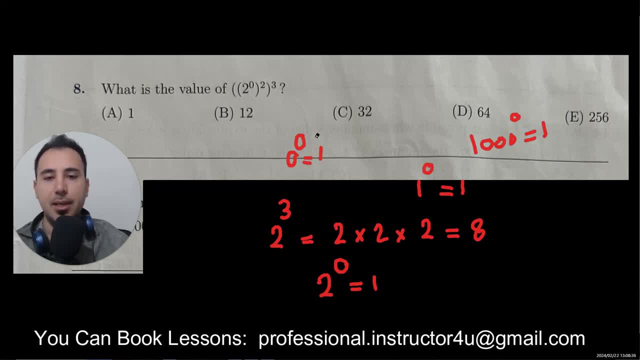 is actually one. this one is a little weird, okay, so let's go here. okay, so if you know these things, you shouldn't get this one wrong, so let's just start from inside. so what is two to power of zero? one? so let's do the question again: one to power of two and again to power of three. 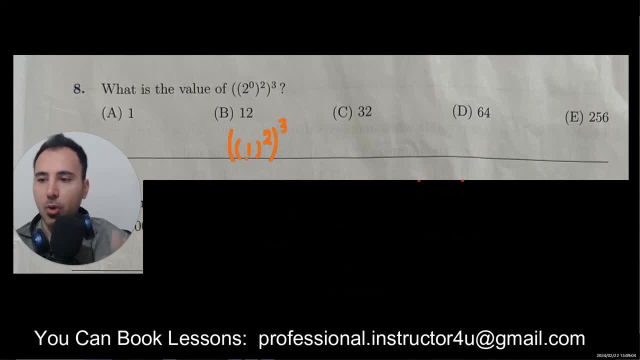 again from inside: one two power of two: one times one is one. you don't write one times two, no, this one one is equal to one times one, so it's actually one again. so the inside value here is actually one. so one more thing is going to be: one to power of three. one to power of three is one times one. 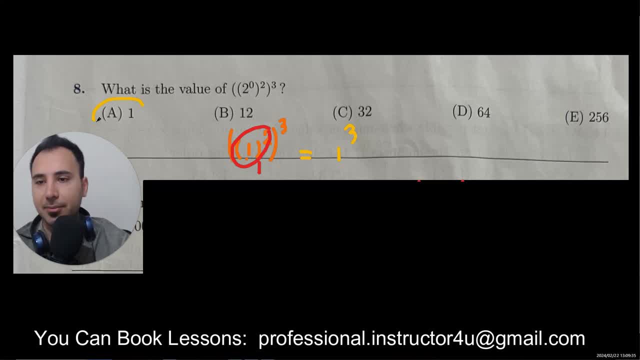 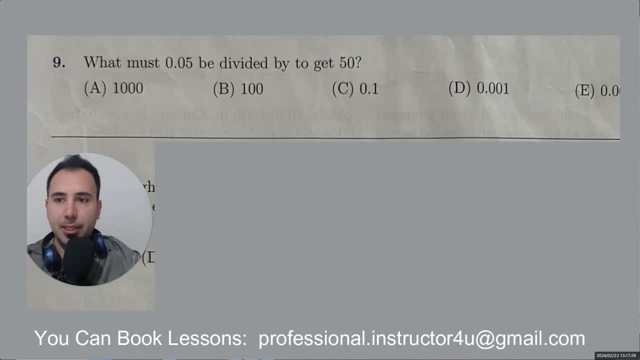 times one, which is one. so a is the right choice. if problems like question nine confuse you, i think the best way you could do is something like this: what must this divided by this b? let's just write it as a fraction. first, zero five over fifty, right, okay? so i wrote this. 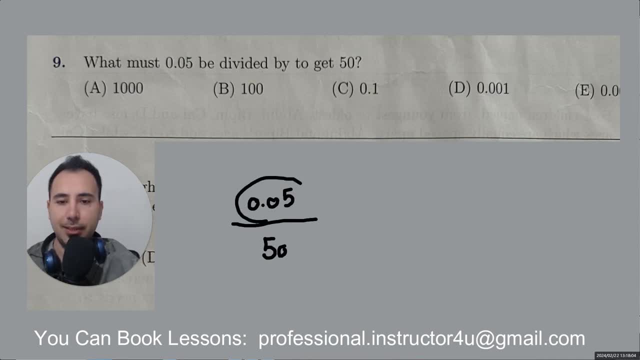 division as a fraction, then i want to get rid of the decimal value. so if i multiply this by a hundred and this one by a hundred, then i could get rid of the decimal. now we'll have a normal fraction. five hundreds times hundred obviously is five, so this one is going to be a five and three. 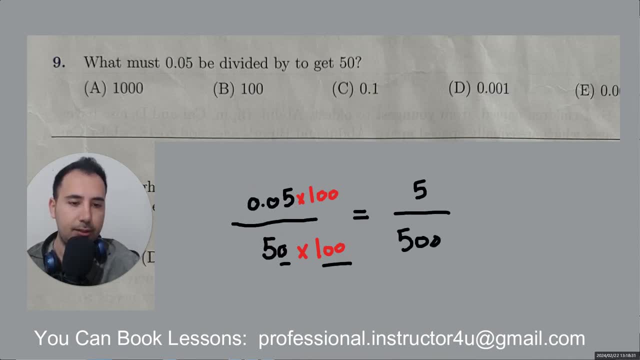 zeros. good, now, it's a normal fraction, that you know. let's simplify both of these by five, so it's going to be one. the first one. five thousand divided by five is a thousand. so i have one of options here. you can see them. so it's going to be one thousand. 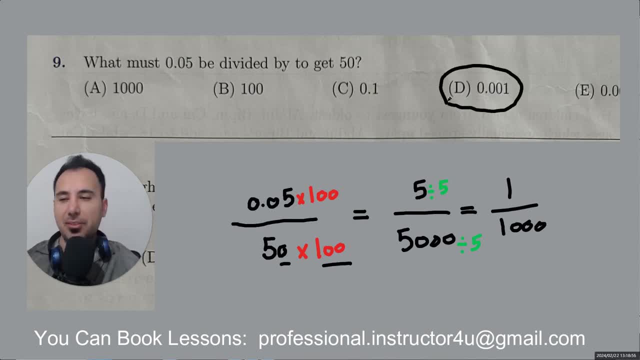 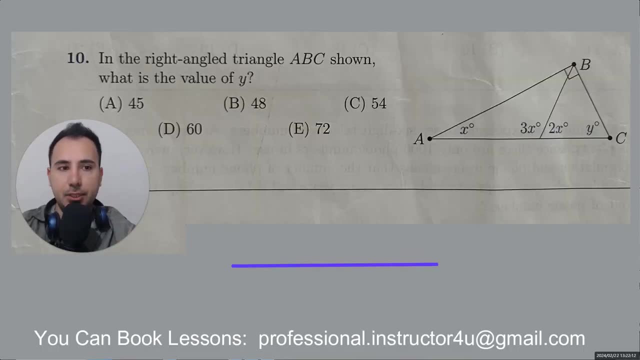 so it's going to be d the right choice this way. i think it's very simple. okay, there are two fundamental concepts. if you know these concepts, then you must be able to solve this problem. let's just review these two concepts. imagine- i pick like a point here- if i go through a circle and come back here to the beginning. 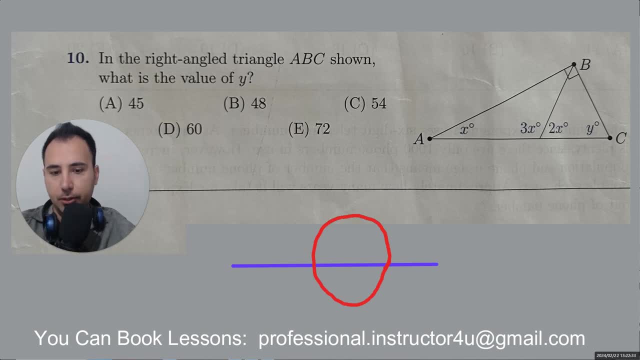 how many degrees is? that is 360 degrees, but if i go halfway and stop at this position here, this is half of 360 and it's going to be 180 degrees. so let's just do that. if i just do a half a circle, a semicircle, like that, it's going to be 180 degrees. 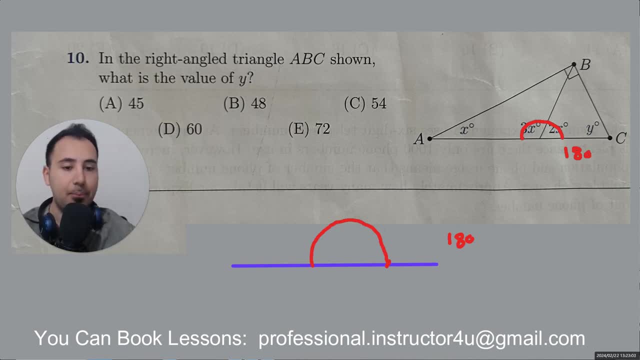 okay, that's the first concept. you need to know, okay, that here in a line we have 180 degrees when we go like this. the second concept is that the sum of the angles of any triangle is 180 degrees. so if i draw the weirdest triangle that i could do, this is i'm gonna go really weird. 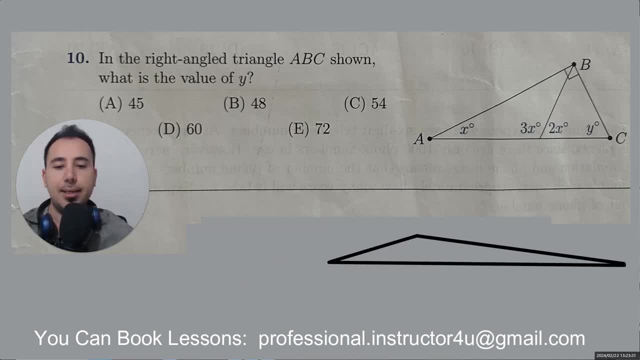 okay. so, for example, what is the sum of the angles? this angle plus this angle plus this angle is always 180 degrees. so if you knew these two things, okay, if you know them now, go give this a try. you must be able to, uh, answer the question now. okay, so here we have a 2x plus 3x. we said that's 180 degrees, so let's. 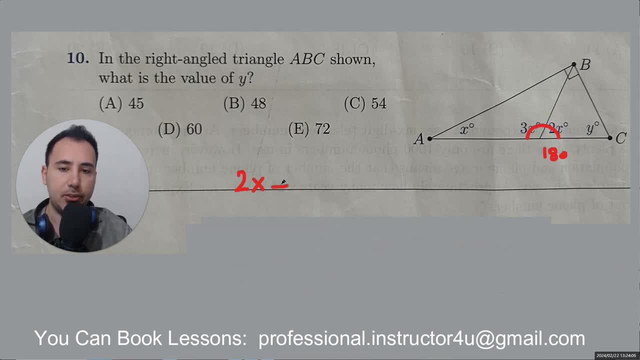 go from here. 2x plus 3x is 180 degree. so what is the value of x? we're going to have? 5x is equal to 180 degrees. so what's the value of x we're going to have? 5x is equal to 180 degrees. so what's the? 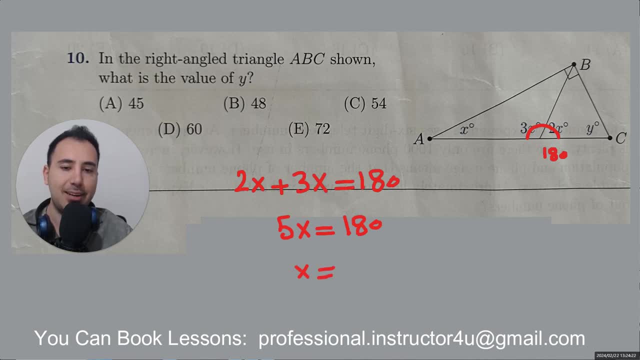 that X is 180, divided by 5 is 36. so this value over here is 36 and I set the sum of the angles of any triangle is actually 180 degrees again. so that means 36 plus this 90 degrees, okay, plus this Y value is going to be again a 180. 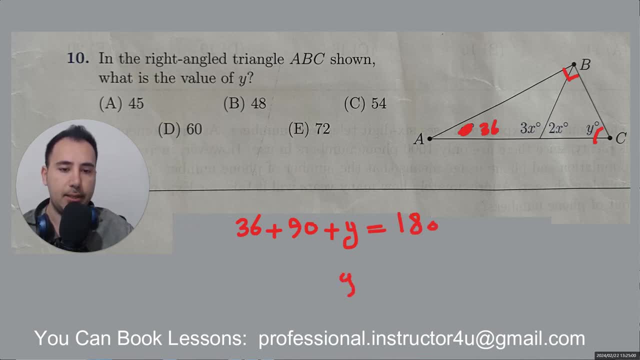 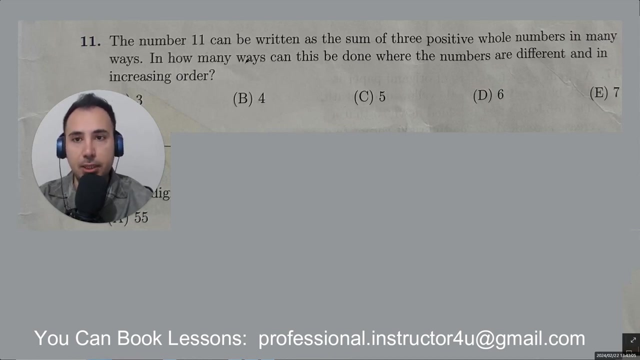 degrees. so Y becomes 180 degree, 90 minus 36, 54. so C is the right choice. you okay for problem 11. it's a counting question, it's not really that difficult. but I want to just talk about if you have a good habit or you have a bad. 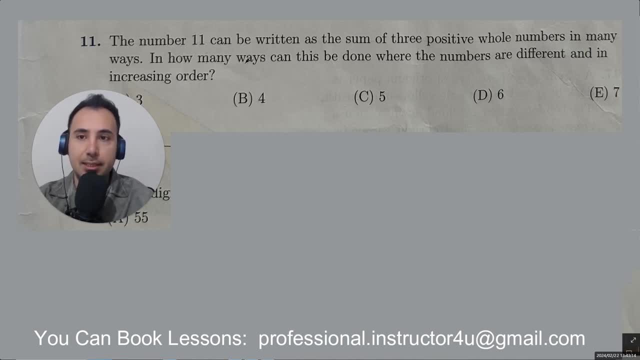 habit when you deal with a question like this. the number 11 can be written as the sum of three positive whole numbers. in many ways, okay, obviously it could be 1 plus 1 plus 9. that would be 1. in how many ways can this be done where the numbers are different and in increasing order? 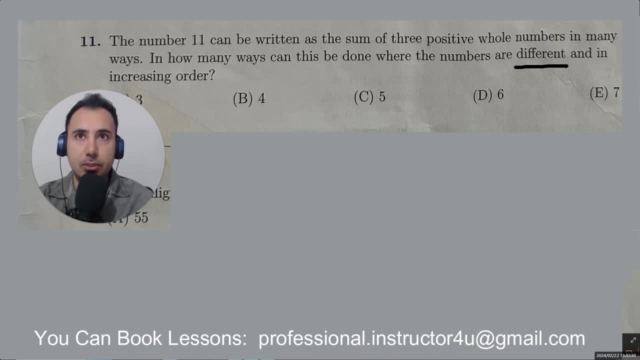 okay. so, for example, I see students writing them like this: they would go: okay, 2, 3, 5 is 1. and then they think about they would go: okay, 1, 4, 6 is 1. are you that person that it's just like: come up with anything that comes in your mind. 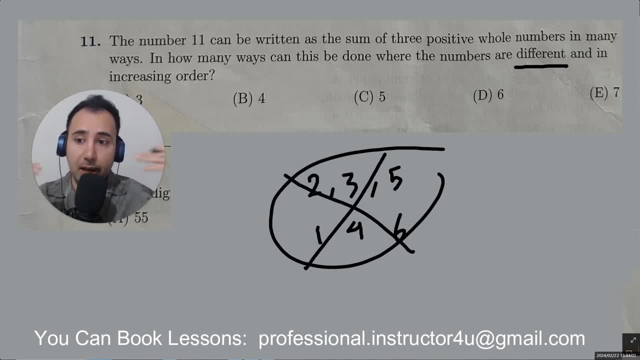 that just like come up with anything that comes in your mind. This is a really bad habit. You don't have organization, Maybe you can't think of one right, So maybe there are. for example, seven is the right answer. You do it like that you could only count six. 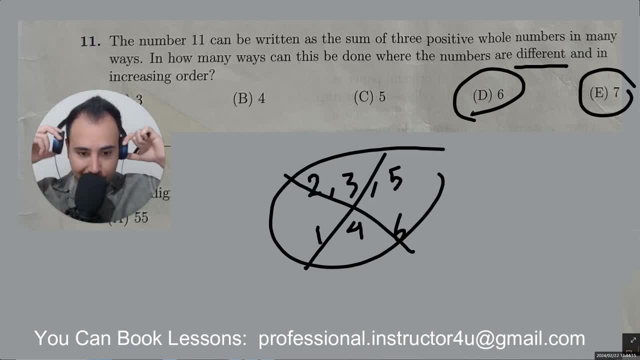 How do you know if you got it all? So what you need to do. you need to have some organization, Like what? So I say the first number has to be one, okay, Okay. and what is the next number? Just one, more than one. it has to be increasing. 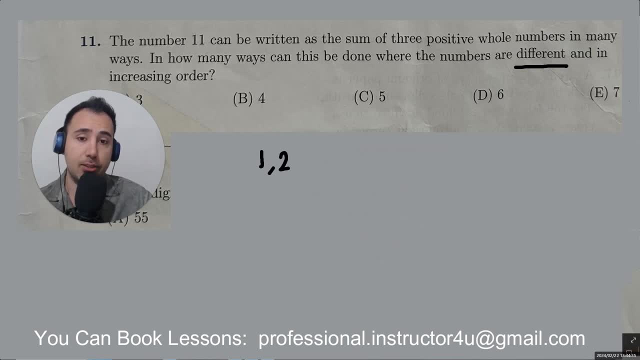 and it has to be different. So if this is one, this is two. One plus two plus eight is 11.. That's the first one, okay, And then you keep this one here. just repeat it here. What is the next number? 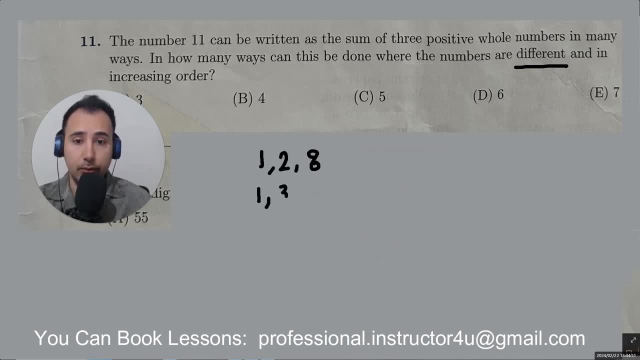 You increase that by one, That's gonna be one, three, seven. I add this two, I add one, two plus one, Then this one has to be eight minus one, seven. okay, So one more, Then it's going to be one, four, that's five. 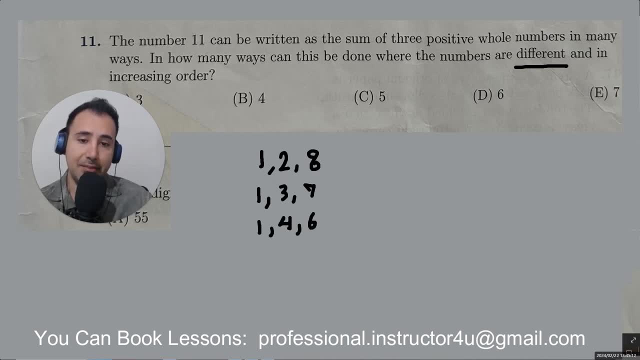 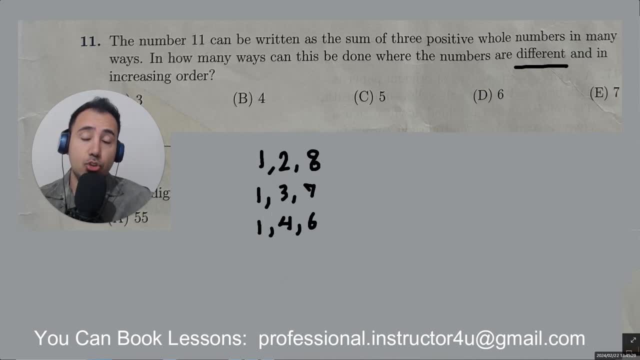 I did all. I did all because I did it and I choose all off of them. that involved one right, So I move on. two, two, So what is only one? after two, three, And then this will be six. 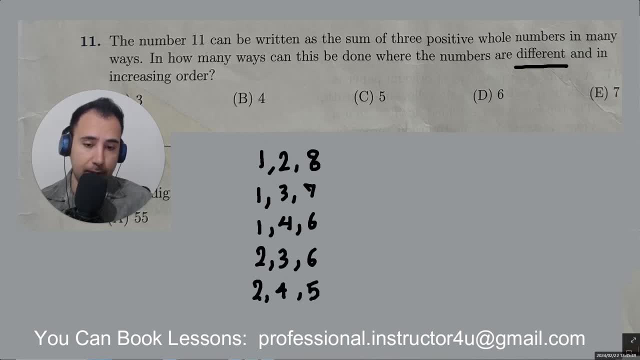 What if I have two after three is four, Two, four is six. This will be five. okay, So let's go one more: 5, 7, and then it's gonna be 4 again. okay, so we already have this and this is not. 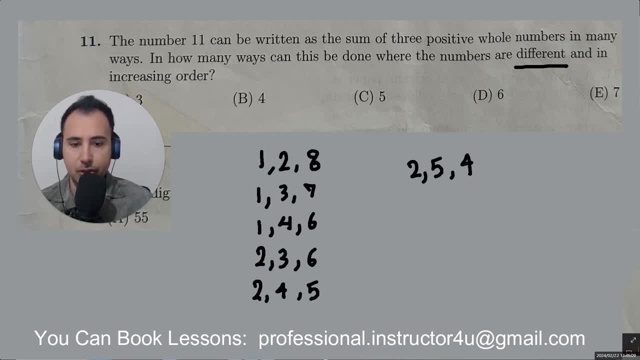 an increasing order. so with 2, we're done, let's just try 3. okay, if I go 3, then the next number increasing will be 4, 3 plus 4, 7. we need another 4 to become 11. is this possible? this one is also no, okay. so that's all. see, when you start with a, 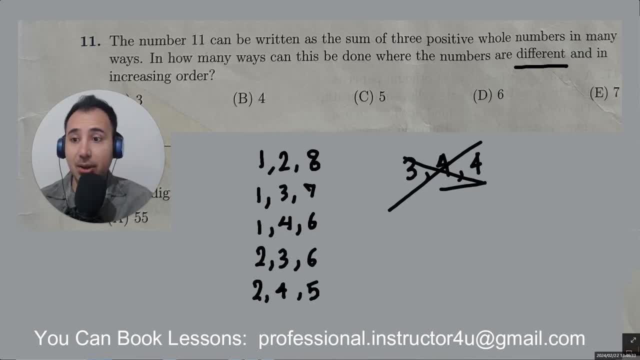 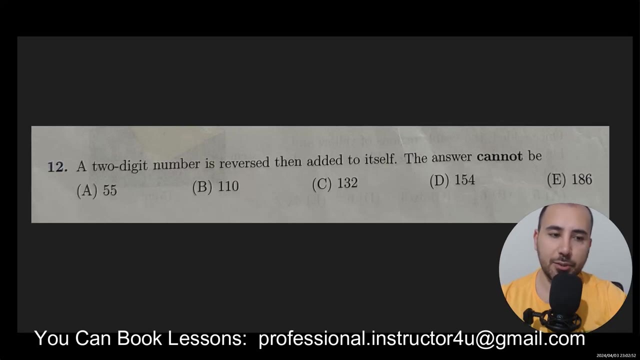 pattern from a smallest to biggest. then you have it all. so one, two, three, four, five and that's it. okay, let's do problem twelve together, and we're gonna do this in two different ways, and number one way we're going to do is: we're gonna do it in two different ways and number one way we're going to. 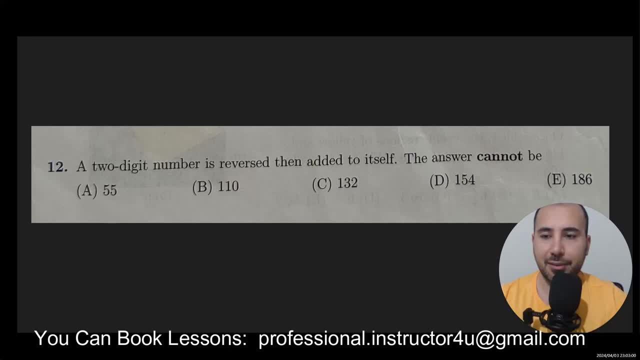 even if you are terrible at math, still you could answer it right. it requires no knowledge, right? you could still answer the question how? let me read it first: a two digit number is reversed, then added to itself. the answer cannot be okay, so right, probably the best way to do the problem is first. 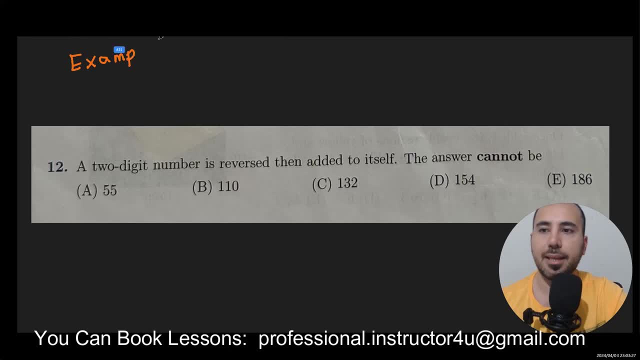 coming up with examples, and then you observe the examples. right, you just come up with a two-digit number. I'm gonna go with 32. okay, what is the reverse of this number? two and three are reversed, so it's going to be plus 23. when I add them, I'm gonna get 55. ah, it says this number cannot be. 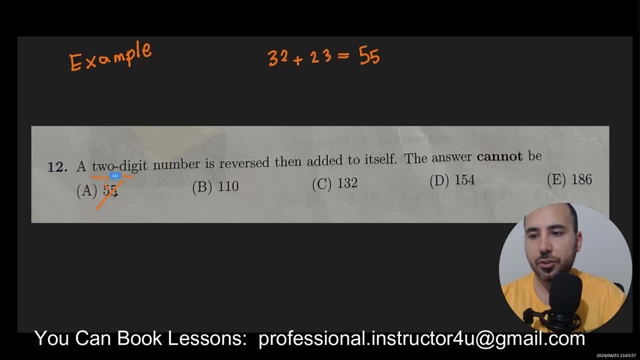 okay, so it can be 55. so out right, we just let's just get with different numbers. I'm gonna go with something larger. I'm gonna go with 74, and then plus 47, it's going to be 121. okay, and let me make go with something a small like 12, and then a reverse of that, and then I'm going to go with. 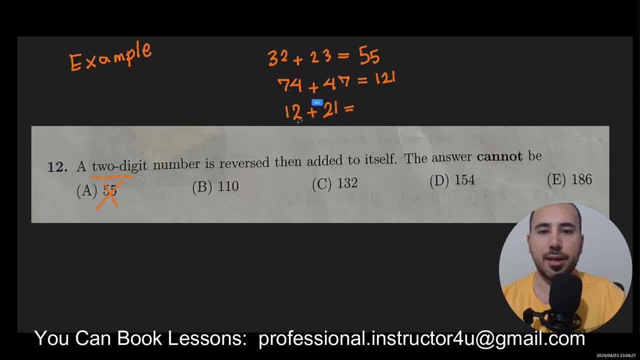 the reverse of that is 21. okay, when I add these, I'm gonna get 33, right? so once you come up with enough example, see, do you observe a similarity between these numbers? all of these numbers are a multiple of 11, right? in other words, I could divide all these numbers by 11.. this one is: 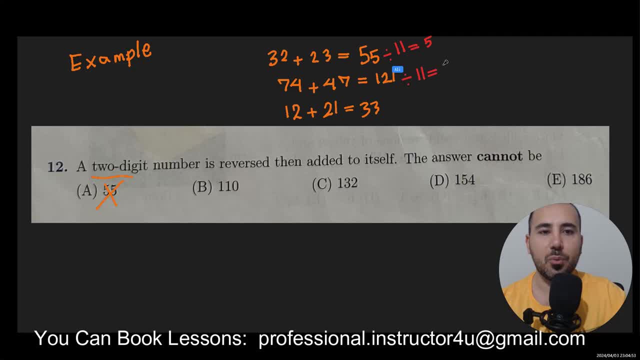 when I divide this by 11, I get 11.. when I divide 33 by 11, I get three. so all these numbers are divisible by 11, and it figured out the problem. so this one is divisible by 11.. when I divide it by 11, I get 10. so out: I divide this by: uh, 11 I. 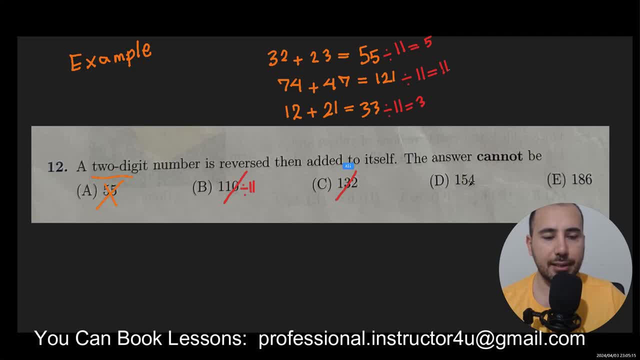 get, I think, 13.. and this one is again divisible by 11.. but this one we see 100. uh, let's see here, 6 is not divisible by 11. right, let's just go here one. let's see here it's going to be 11, 76.. you see, 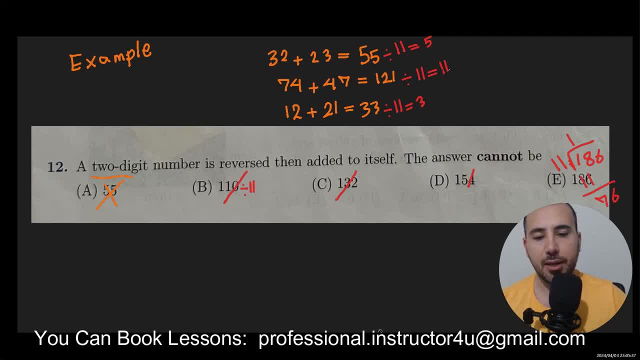 that this number is not divisible by 11.. so the right answer to the problem will be 186.. that was approach one. it requires, like, no math knowledge. right, you could answer the problem. uh, the number two way we could do is going to be a little more systematic. okay, and uh, probably this is a more advanced way. 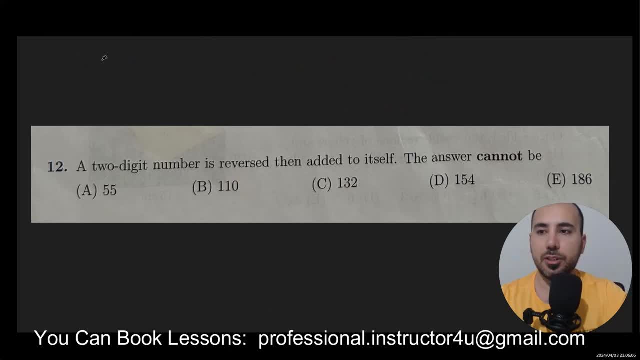 equally a really good way. so a two-digit number. we're gonna write it as a- b. so, for example, let's go back to our example of 32.. when you write 32, this tree is just three times 10, right plus two. so I'm going to apply this to a- b, so I could write a b as whatever a is: 10, a plus b, the. 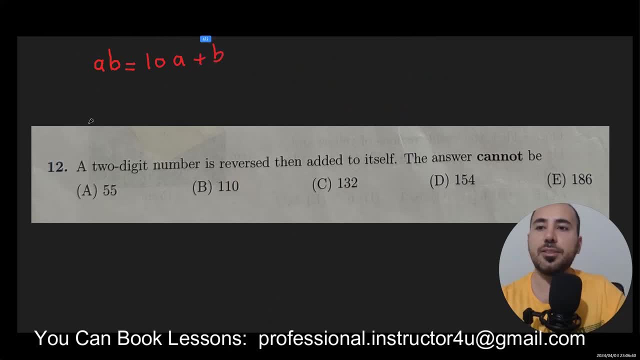 same way as I wrote 32.. and what is the reverse of this value? ba, right, and this is equal to 10 b plus a. and the question is saying: okay, we want to add them to together. so what is a b plus b a? it's going to be this part plus this part. so okay, if I add them all together, it's going to be 11 a. 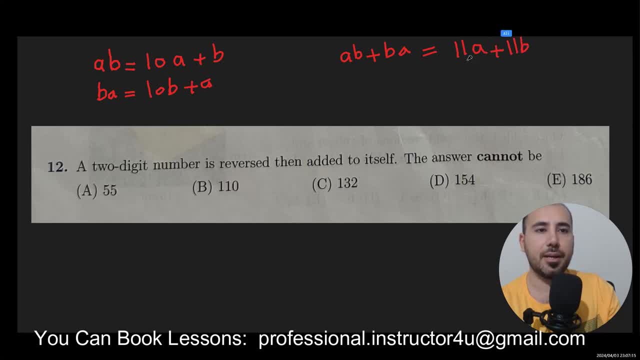 plus 11 b. okay, so a 11 is common. I could factor it so it's going to be 11 a plus b. so what does that mean? that's kind of like the proof that the sum of the numbers, like you two-digit number, you reverse it. 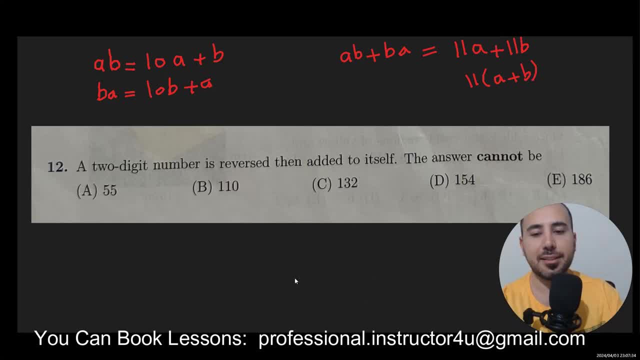 you add them together is always divisible by 11.. so you just have to go through the options, as we did, and find which one cannot be divided by 11, and it's going to be this one. so that's why we choose e. okay, problem 13.: 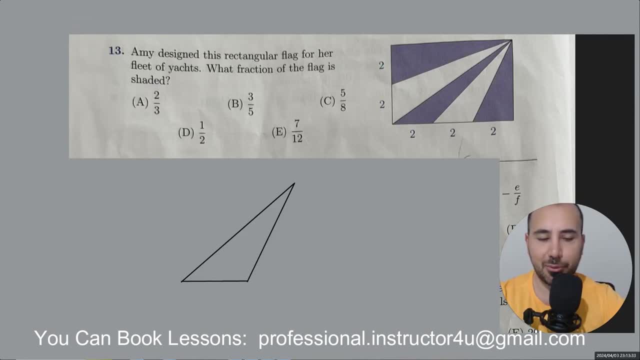 even though I think this question is not very difficult. but I'm pretty sure that a lot of you will have problems with this problem and I think a lot of you have problems figuring out the area of this triangle. and again, you have that because you don't know where the height actually is. 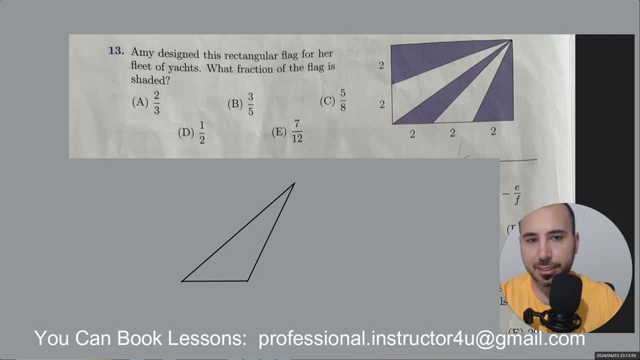 see, if you can't do the problem, it's because, for example, if this is the base, where is the height? see, I see some of my students will go, okay, where is the height? they'll just try to go like this: is this the height? is this the height? where is the height? 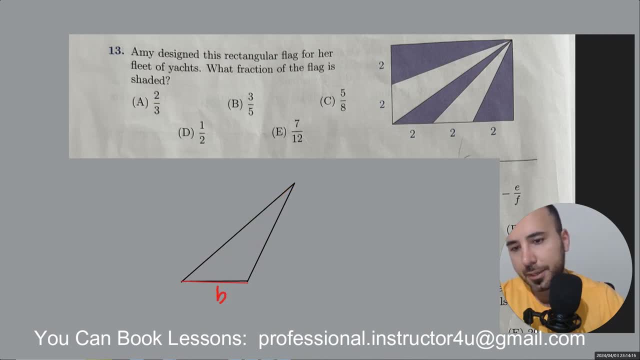 the height, okay, has to go from this vertices, which is opposite the base, right, and it has to go 90 degrees perpendicular, and now none of them are perpendicular. so in this case you will make, you would extend the base both sides right, and then you would say: 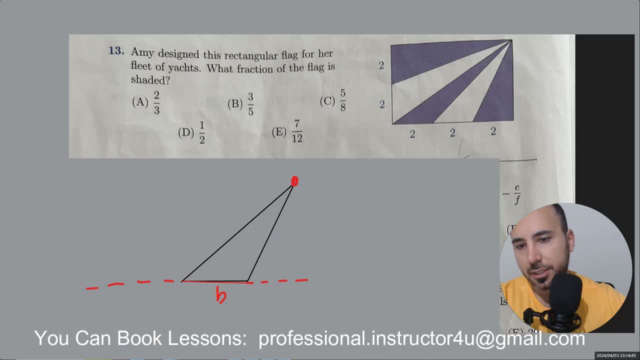 okay, I could draw this from here to here. now, this is your 90 degree and this becomes your age. this is your height, this is your base, and the of a triangle, we know, is just h times base divided by two. right, this is the missing point. you didn't know this. now you could answer the problem. okay, let's see how. let's just do it. 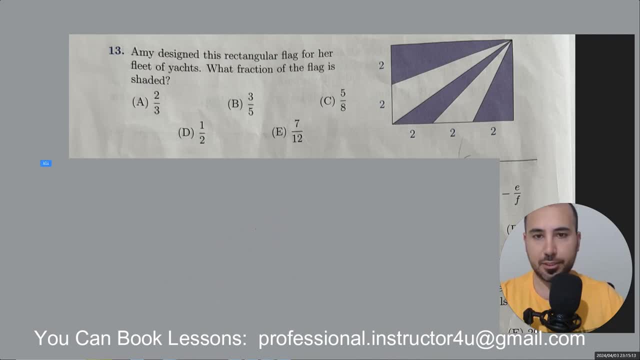 together. now let's just start with the easy one. this is two and this is 90 degrees, since the question says it's a rectangle. okay, my picture, my diagram, is not the best, but this is two. how large is the largest side is two plus two plus two, so the largest side is six. this is two, two. 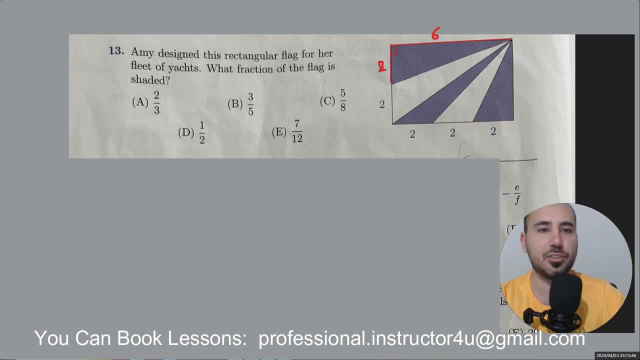 times six, twelve divided by two, sixth. so all of this area is six. so all this area is six. let's go with the other one, that is easier. this is two. this one is two plus two. right, this is two plus two is four, because this is equal to this. it's a rectangle. 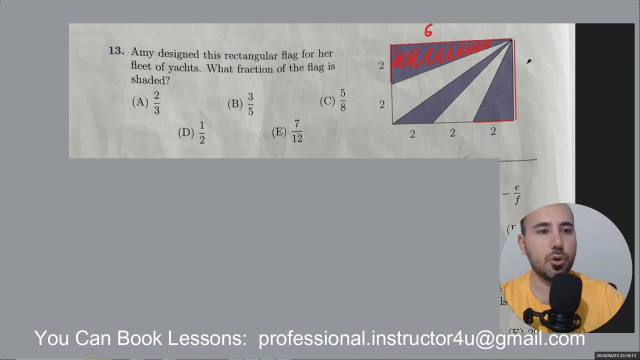 right. so two times four divided by two, eight divided by two is four. so there you go we. we're already done with this, so let's go with the other one. almost done so. this one is four times two divided by two. this one is four. now the only one remaining. 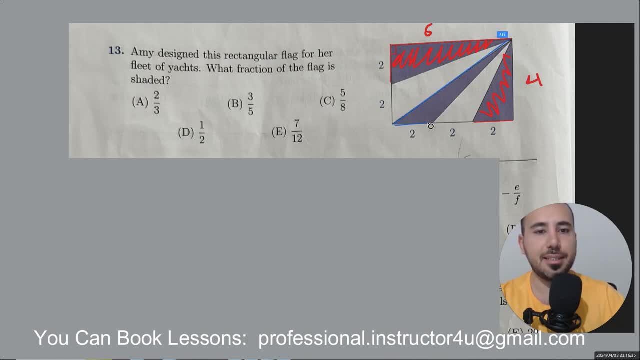 probably the one you couldn't get, is this one right over here. the base is two and where is the height? so this is two. i'm gonna write two times the height of this, as i just showed you. is this one again. so this is 90 degrees. 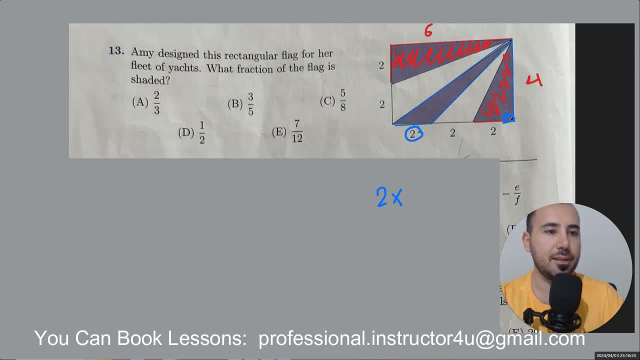 three to the base. okay, so the blue triangle is going to be two times four. divided by two is going to be four, so the blue one is also four. okay, so the total area is six plus four plus four is 14.. okay. what fraction of the flag is shaded? 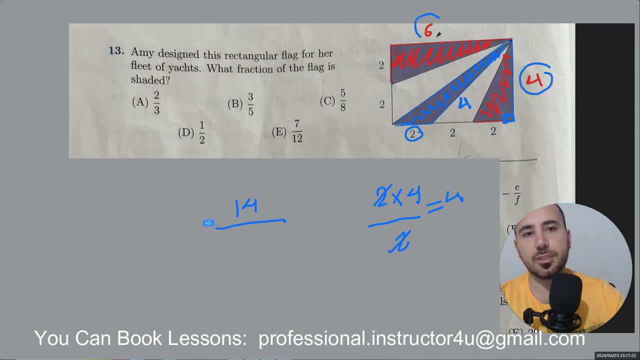 what is the area of the rectangle? four times six, twenty four, both of them are divisible by two, so seven over twelve, e is the right choice. okay, before we move on to the next question, something interesting now is that i want you to take a moment and see that. 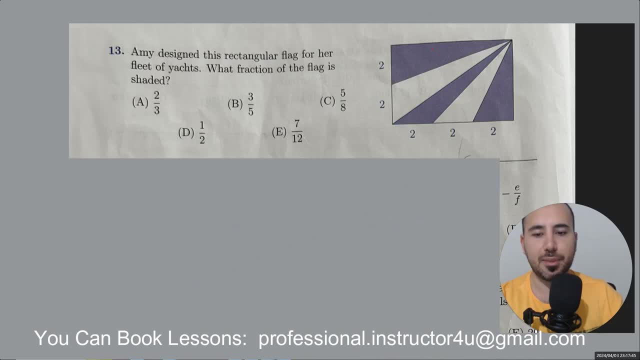 the area of both of these were formed, so they do have equal area. this triangle is actually equal to this. both of them are four. why do they look the same? i don't know. maybe they look the same to you, but i'm not sure until i just do the calculation. both of them have this is two. 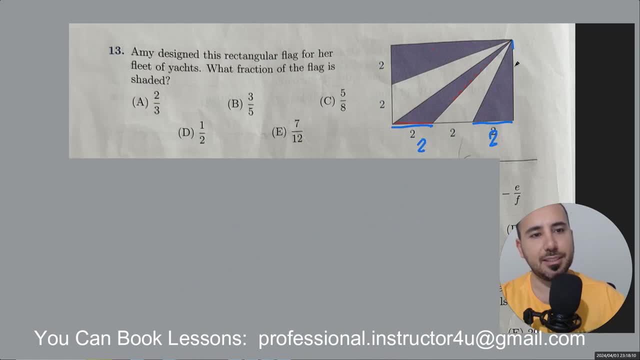 this is two. both of them have the same basis. this is the height for this one. guess what? the same thing is the height for this triangle. so bases are the same, heights or heights are the same. so absolutely, they have to be equal. okay, let's move on to the next. 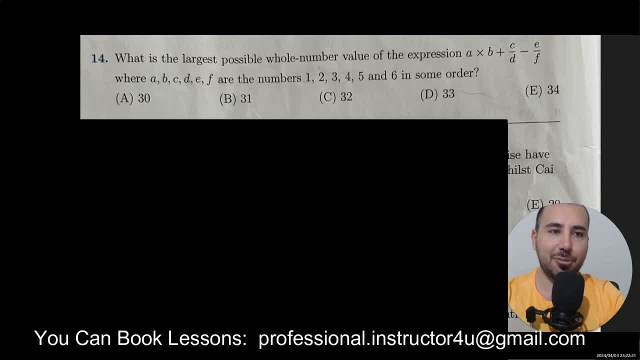 well, problem 14 is extremely easy for some students and extremely challenging for some others, right? usually my students are in two groups, right? so some students they are instruction based. they say once they read the question, they expect to know everything and then they start dealing with the question. right, and there is the. 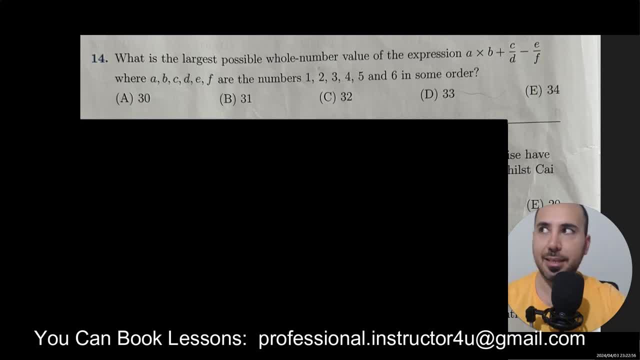 second group that when they see a question like this, they say, okay, I don't know how I'm gonna answer the question, but let's just start. okay, let's just put some of these numbers like plug in these values, in these variables and see what happens. I will figure it out and they will figure it out. you need to be in the 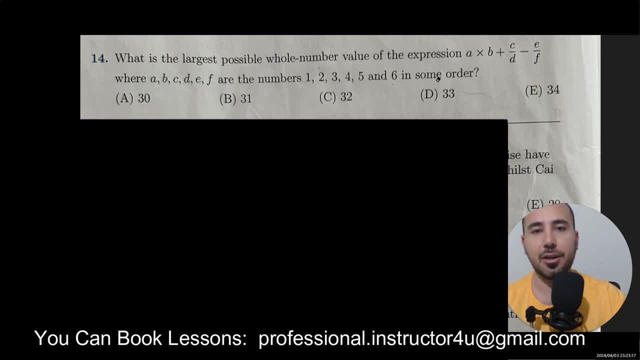 second group. this problem is actually a lot easier than you think. what is the largest possible sum, whole number, value of expressions, where a, B, C, D, F are the numbers? okay, in some order. now let's see what you want to maximize this value, right? so what do you think I should put? my six. so should I put, for example, my 6? 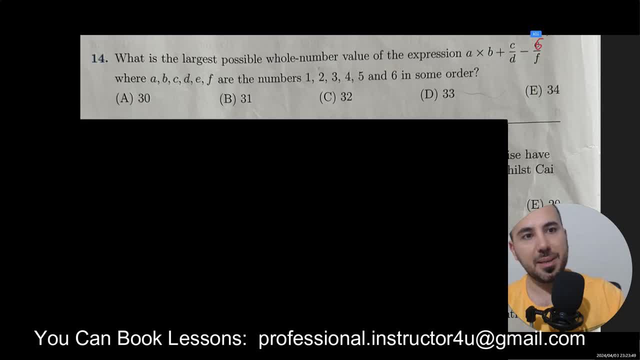 in the negative part. should I make this part that is negative a small or large? that's the first thing. these are the questions we need to ask. we want to make this one a small, as a small as possible, as at least as possible, and we want to maximize these two. you really want them to be great, but 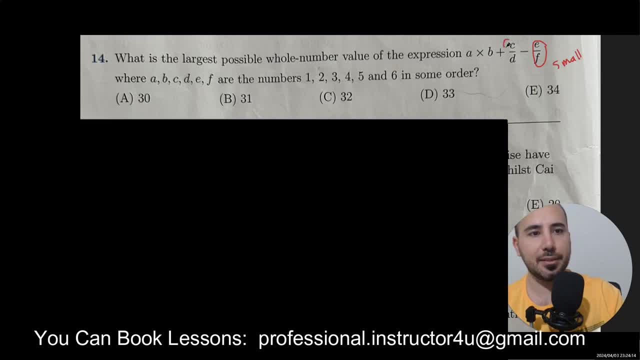 where should we, where should I put, for example, my six here? if I put six here, and then what is the smallest thing I could put here is what you should I put six over one or should I put my six over here? so if I put my six, 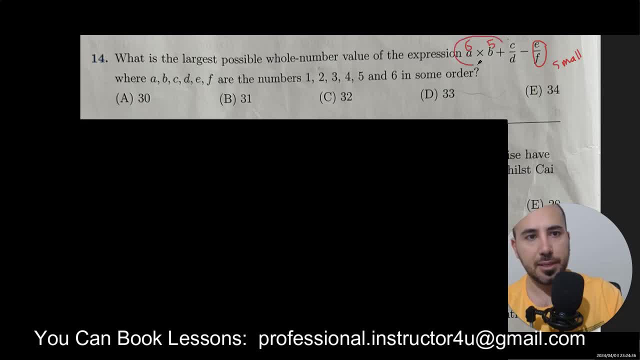 here and my five here. see, I already made something great, but if I put six and five in any other places here, okay, then it's a waste, right? we don't want to do that. so the first two numbers okay, because we want to maximize this. I'm 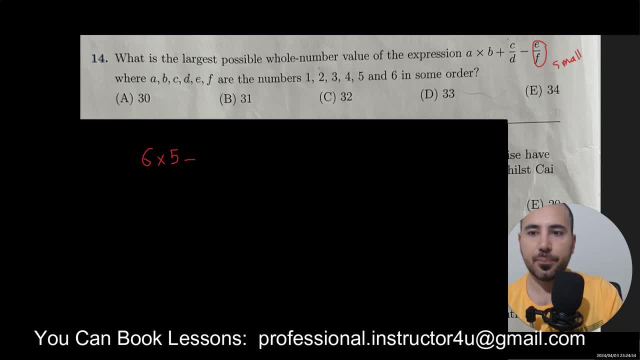 gonna write it like this: six times: five plus C over T. now these are gone and we want to maximize this right, so probably let's just try this, for I put it on top. below is one, because four is really large, and for the minus part, minus because should I put three over two or two over three? which one is smaller? 2 over 3 is 3. 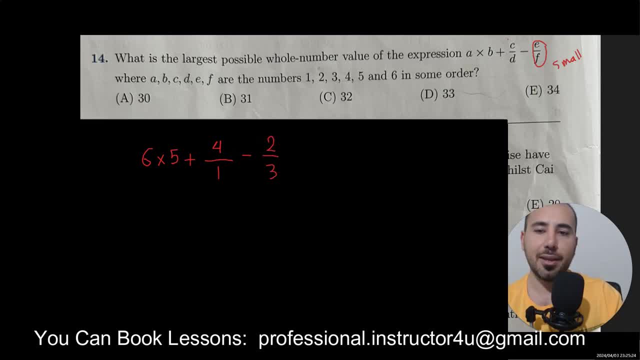 is smaller, but there is a problem now. the problem is that this is not an integer value, but the question said we want the answer to be a whole number. now this is actually 34.6666. blah, blah, blah. right, it's not an integer value. i actually made something higher, but it's not integer. so 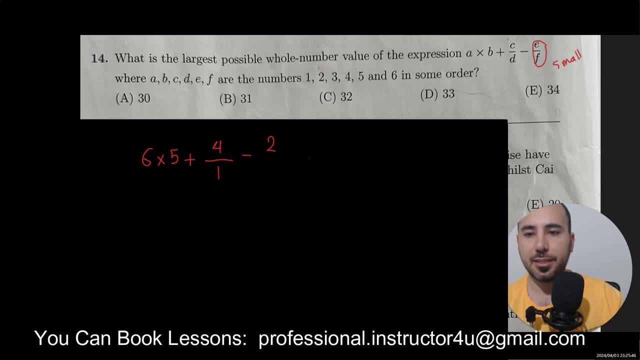 unacceptable. okay, so that means we need to. instead of that, maybe i could go with a four over two. okay, i could go like that. and then minus one over three is not possible. minus three over one, that's one way to do that. okay, now it's gonna be 32. minus three is 29. 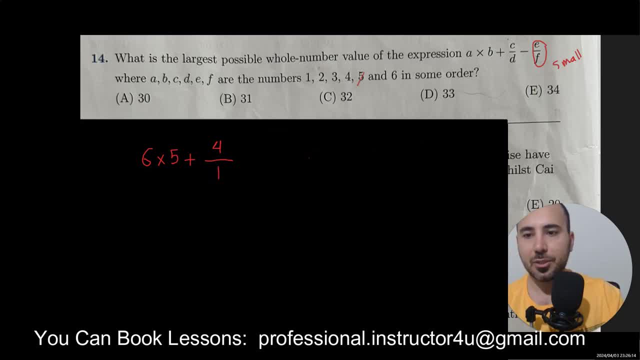 it's not in the options, okay, Okay. so the other option that I have here is: let's see here: Maybe I could use 3 and 1 here to get myself a plus 3, and this one minus 4 over 2.. 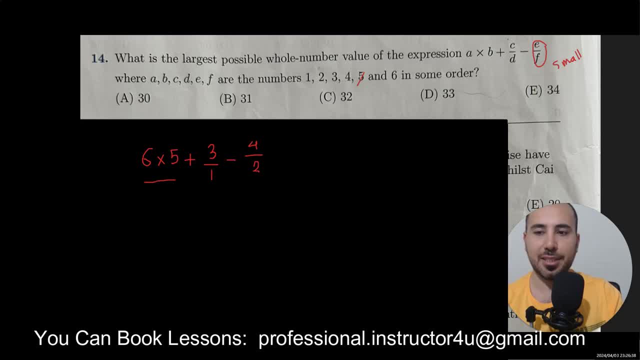 All right, this is going to make it even larger. So this will get me 30,. this will get me a 3, and a minus 2.. Okay, and it's going to be 33 minus 2, 31.. 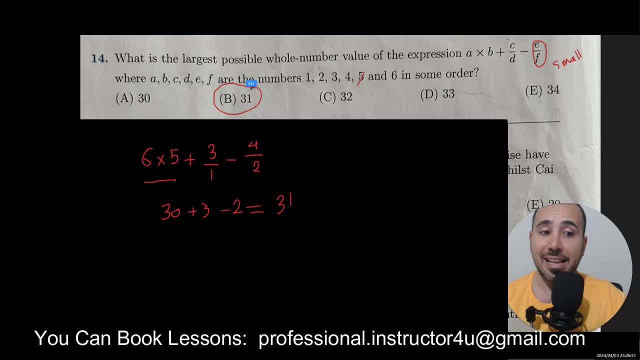 So B is the right choice. Who can't answer the question? People who are saying: wow, a lot of variables, this looks difficult, I can't do it. Who can't do it? Just start trying out different options and just see which one is. 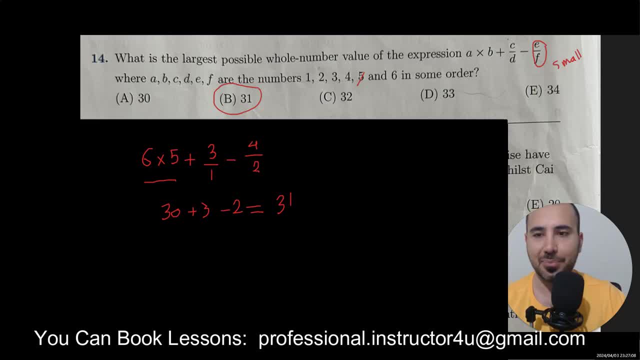 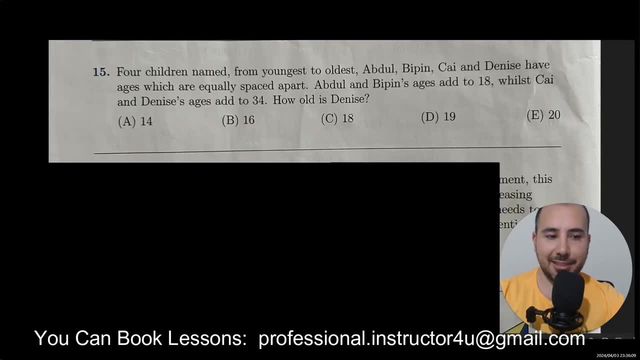 of the maximum, which one is the highest number? Okay, not difficult. Okay, problem 15.. If you can't answer this problem, I think you are overthinking the problem, right? So probably you're just writing equations and all of that and say, ah, I can't do it. 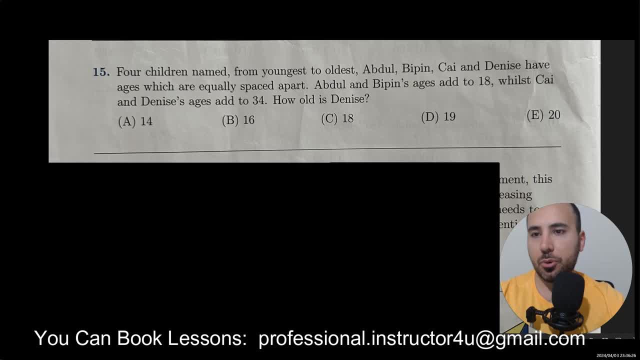 So it's way easier than you think. Four children named from youngest two. So A is the youngest. Let me make this larger: A is the youngest and then B is the next one, C is the next one, D is the next one. 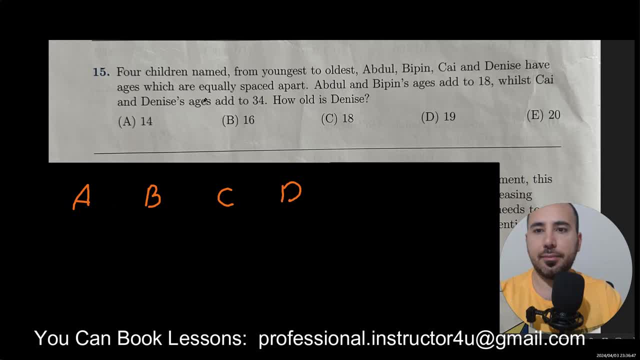 Now they have ages which are equally spaced apart. What does that mean? So, for example, if D is three years older, then C is, for example, three years. So if A is three years older than B, B should be three years older than A. 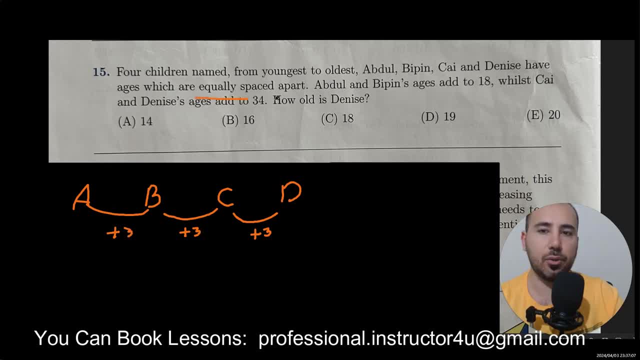 It has to be the same, That's equally spaced apart. This is what it means. And then A and B, their ages, add up to 18.. And C and D added together are 34.. How old is the last one? D? 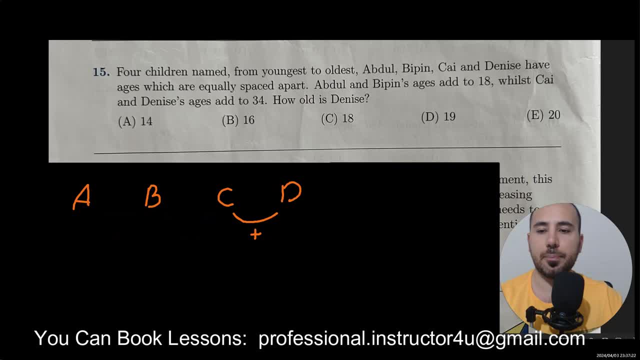 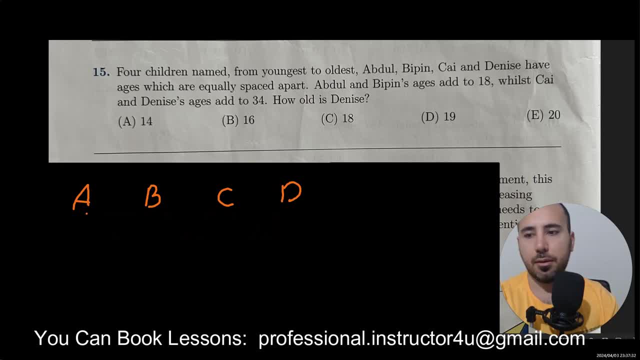 they get 18.. One way would be nine and nine. Is that possible? No, because B should be older. Then the next number to try is 10 and eight. So the difference here is two years. So the next person, if that's true, will going to be 12.. 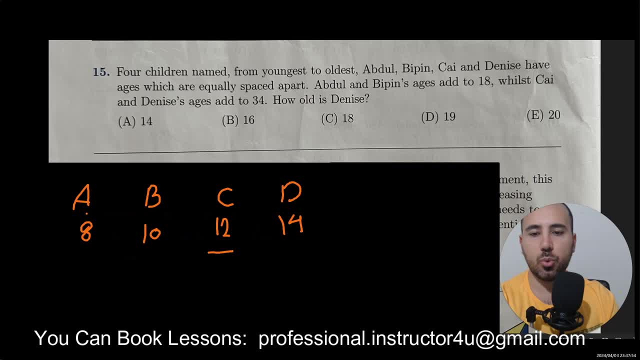 The next person is going to be 14.. What is 12 plus 14? 26.. The question was 36.. The question was 32.. So the difference between them- 10 and eight- was not good. Let's try the other one. 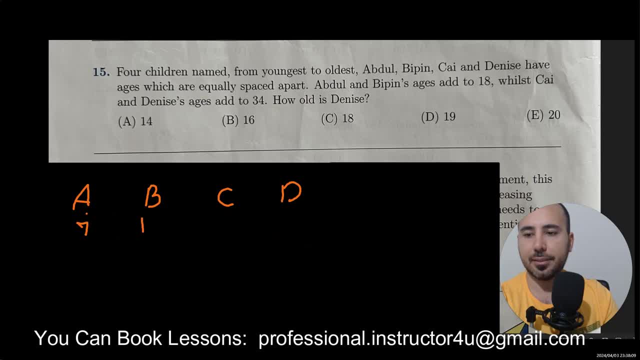 Let's try seven and 11,, the difference of four. Okay, let's continue that: Seven plus four, 11, plus four, 15, plus four. So what is 15 plus 19?? 34.. So how old is D? 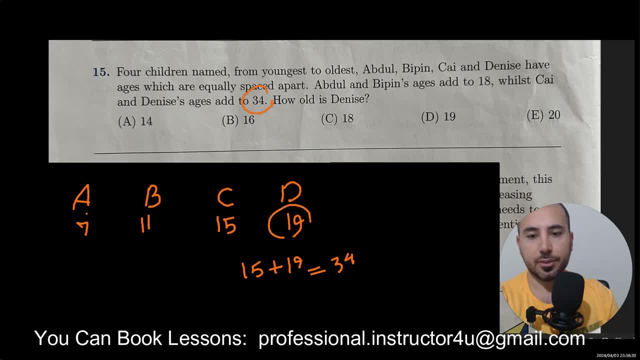 19. 19. 19. 19. 19. 19.. So easy, right? If you just have the right approach, it's so easy. If you want to write equations, oh, you could write equations. See, I would never advice writing equations for this type of problem, right? 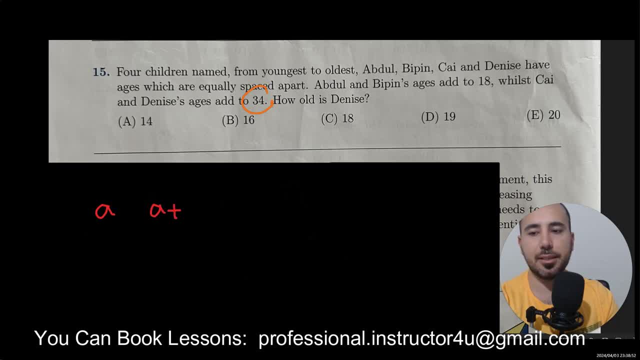 The first person will be A. The next person, B, would be A plus D. The next person will be A plus 2D will be a plus 3d. ooh, that's a lot of time wasted if you just want to go with. 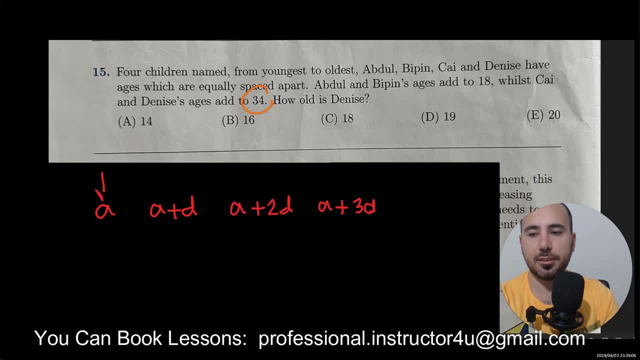 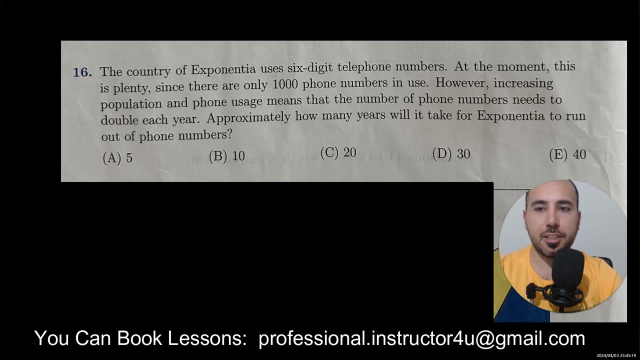 this, okay. a is like the age of the first person, D is the. how many, how much is added each time? okay, then you can write equations. never advise it for this type of questions. okay, I'm gonna give you some tips for this problem. that makes it a lot easier. the country of exponential. so it's just telling us. the problem is: 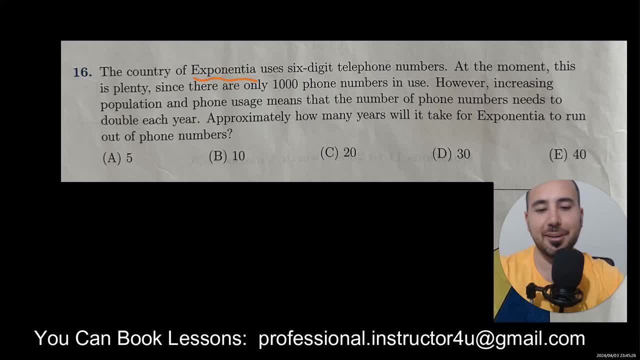 exponential. this is the first hint of the problem. using uses six digit telephone numbers at the moment. this is plenty, since there are only a thousand phone numbers in use. however, increasing population and phone use is a lot of time wasted if you just want to go with this type of question. 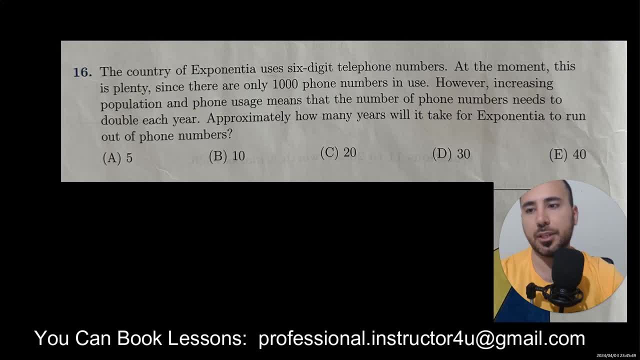 is that the number of phone numbers needs to double each year. approximately how many years will it take for the exponential to run out of phone numbers? okay, so when you see this number, okay, the good habit is to just check out the options. see, are the options right? for example, five, six, seven, eight. I are they. 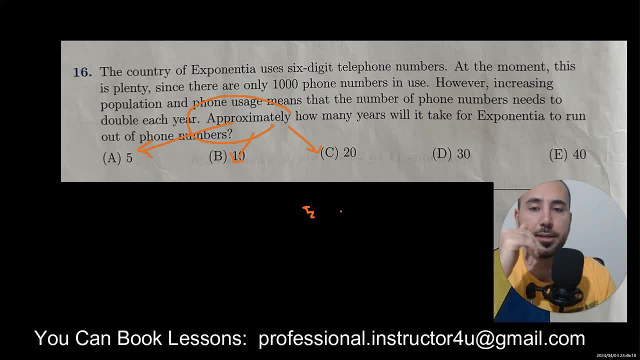 really close or they're so different, right. so that's the thing, see, you would see immediately that the options are too far. okay, and that's a good thing, because we could round these numbers right. so right now we have 1,000 numbers. next year is going. 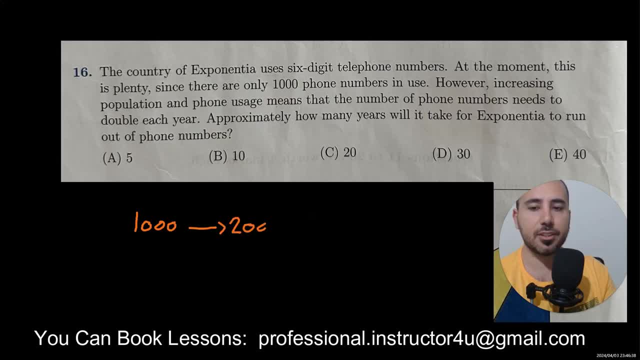 to be 2,000, next year is going to be 4,000 and it's going to exceed them, so that's really the best YOUよう attempt to run out of phone numbers for when you're in food. future related to yourbe care. 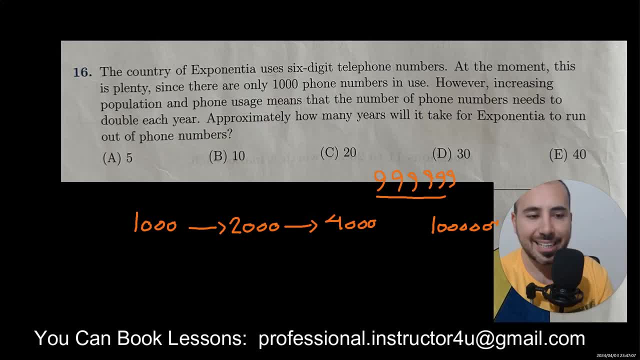 that I'm warning you guys. I know this is gonna be a hell of a unlikely outcome, because there's people like it, okay. so, depending on the time you have the chance, the best way of calculating this number it's really like this: you shouldn't multiply this. 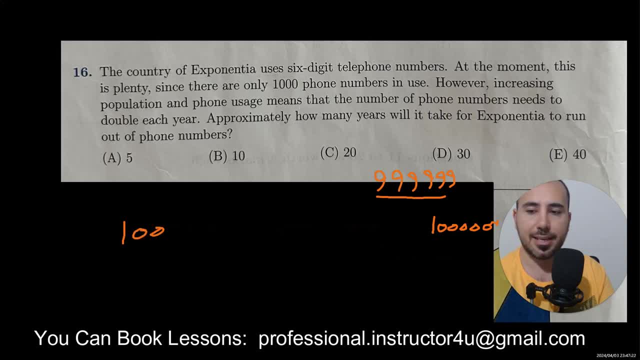 number. you should tell yourself this: a thousand multiplied by two, two, two multiplied by two, multiplied by how many twos will be greater than a million. the number of twos here will give you the answer. so you could also write this exponentially. that would be a more professional. 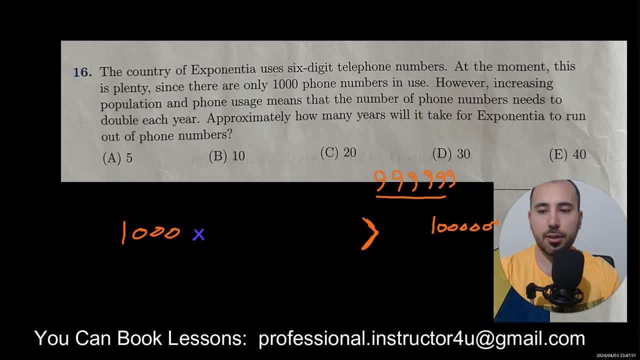 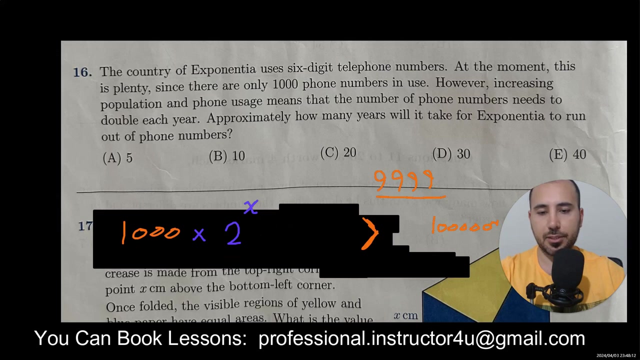 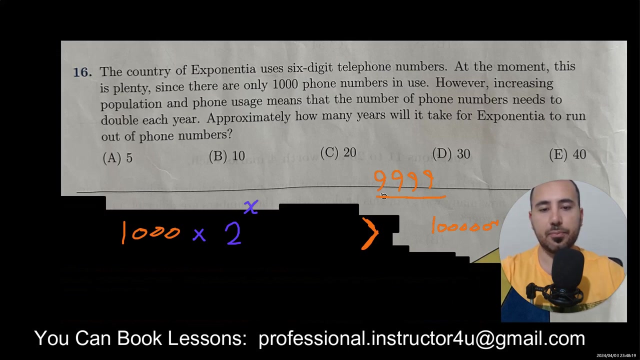 way of writing it. so how many? two should be multiplied and then multiplied by a thousand so that they become more than a million. okay, so if you turn it into an in groups, if you turn this into an inequality- wow. so let me correct this a little bit. if we turn this into an equality like this, let me clear this. 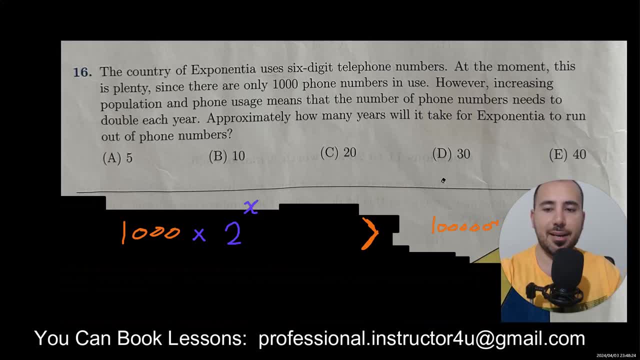 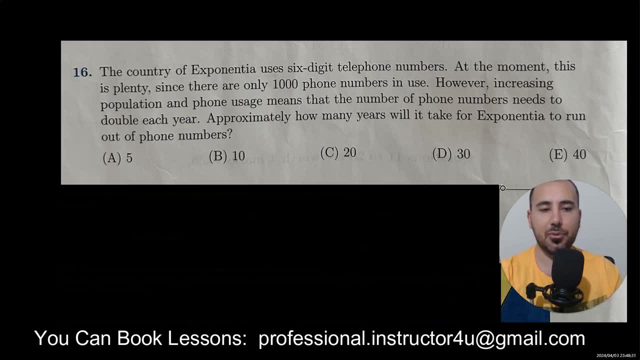 then it would be easier. you have a thousand multiplied to raise the power of x greater than a million. right, let me rewrite it and you think about how you can answer this quickly. a thousand multiplied by two to power of x should be larger than a million. can I divide both sides of any inequality by any number any? 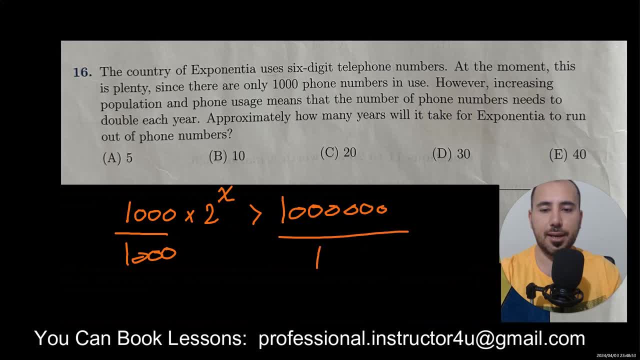 positive number, is it okay? yes, let's do that. so these two numbers are, by pen, a thousand. so a million divided by uh, it's again a thousand. so see, I'm writing this to explain, but when I used to do this question myself, or you're good at this question, you don't even need to use this, you. 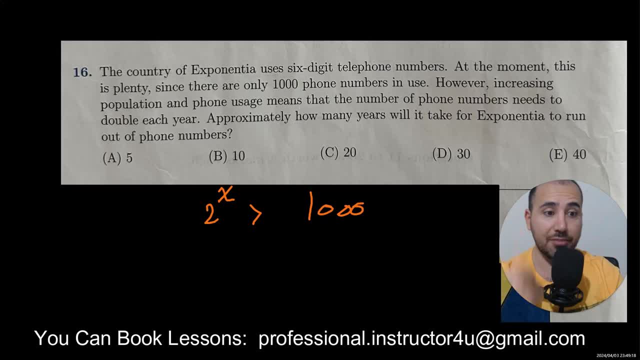 would go: one million, what divided by a thousand is one thousand. two to power of what number is greater than a thousand? the answer I hope you know is 10.. because two to power of 10 is a thousand and 24 is greater than this. so, if you're good, 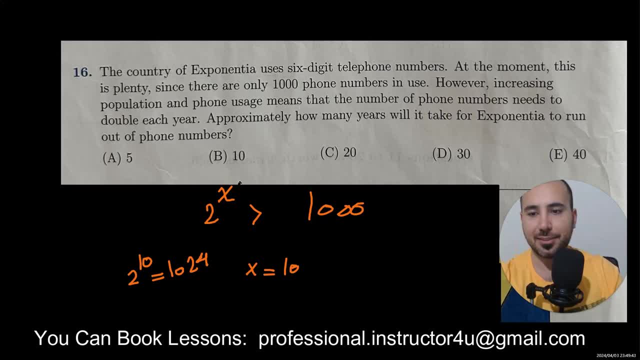 at this you could answer the question like under a minute. so this has to be 10.. but why did I turn the number into a million and this one was a thousand? because look at the differences- five years. so for example, after five years, how many phone numbers are being used? 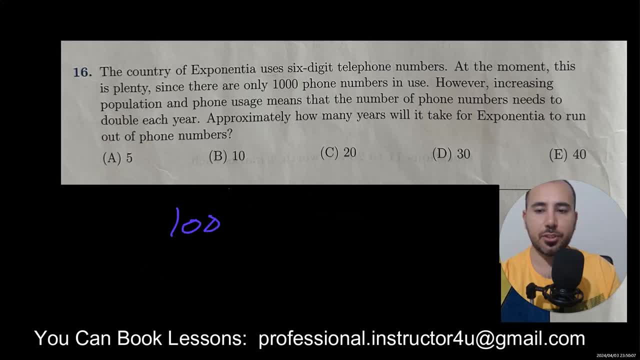 it's going to be like this: after five years you have you start with a thousand. after five years, multiply by 10 to the power of 5, this is 32. so after 5 years there's only 32,000 like phone numbers use. it needs to exceed 1 million by 10, like this: ooh and. 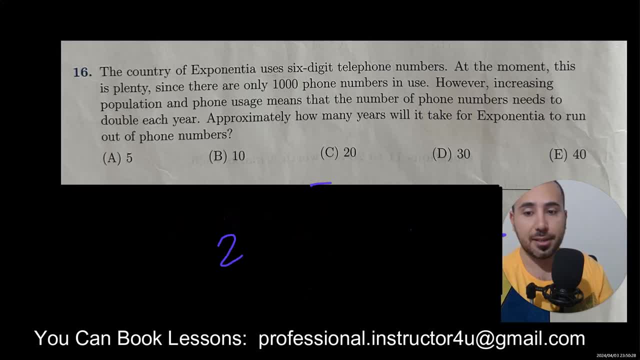 if you go to to power of 20, do you know how large it is? that's gonna be about 2 to the power of 10, multiplied by 2 to the power of 10. approximately, this is a million thousand multiplied by thousand. so we start by a thousand. so and then, 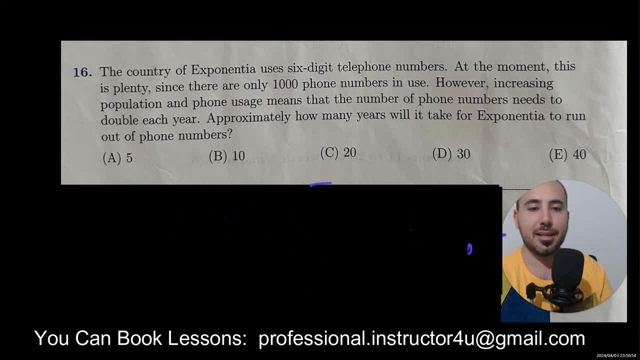 you multiply by a million, do you know what that means? that means after 20 years it would be a billion phone numbers. I tend to power of 9. right, this is like what the population of India right now, so this city, after 20 years, will reach. 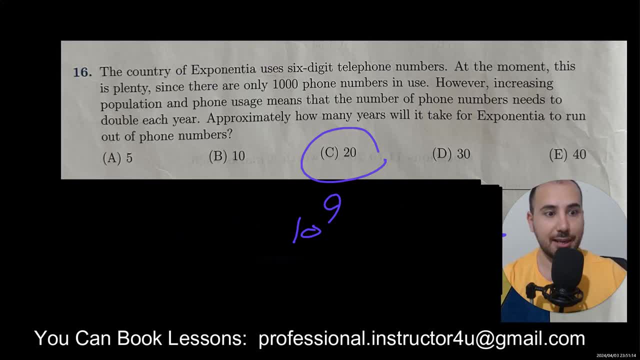 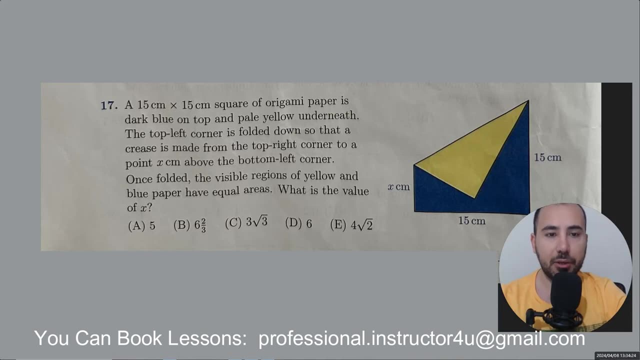 the population of India. okay, so you see how you should answer this type of questions. you know the right way. it makes it really easy. okay, I have some advice for you if you are a person who has problems with questions that require visualization. usually they take a lot of your time. so if you are that type of person, maybe the 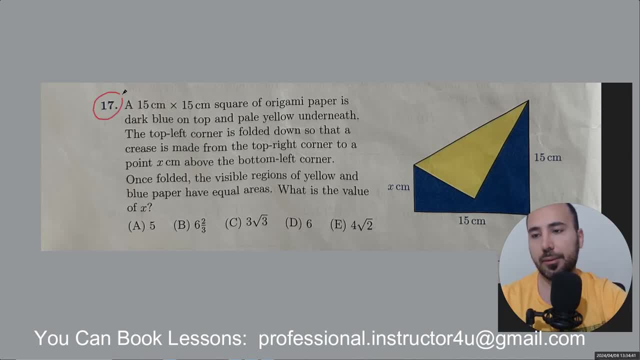 best idea is to skip these questions, like mark them, and just move on to the next questions. later, if you have extra time, you come back and just attack these questions, but usually this is the best strategy. I've had a student they say I did really well up to this question and then this problem wasted a lot of my time. 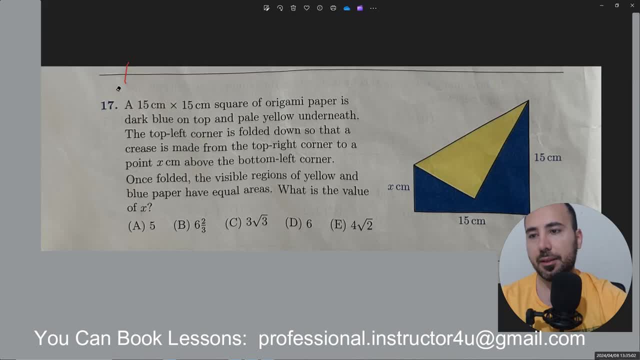 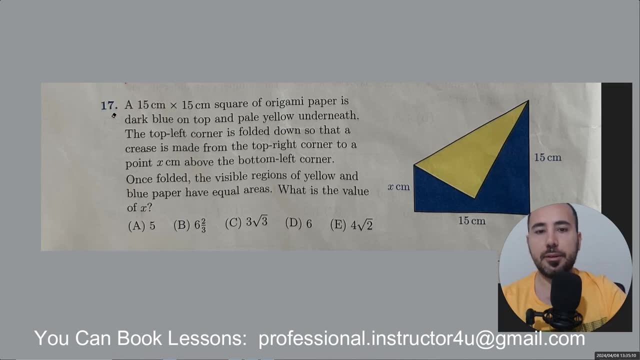 so It could also be used. so be careful. like the questions that require visualization, Let me also clean it here. Let's just read the problem. A 15 by 15 centimeter square of origami paper is dark blue on top and pale yellow underneath. 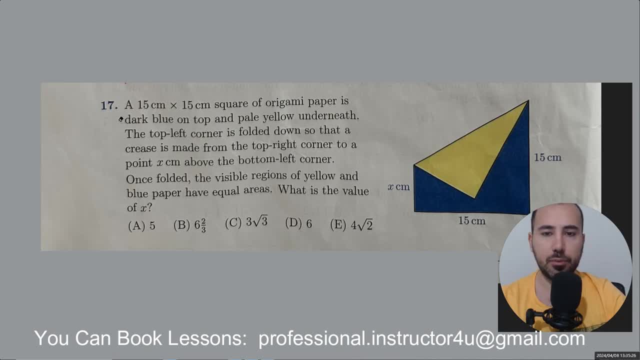 The top left corner is folded down so that the crease is made from the top right corner to a point X above. Basically, all this information is on the picture. Once folded, the visible regions of yellow and blue have equal areas. What is the value of X? 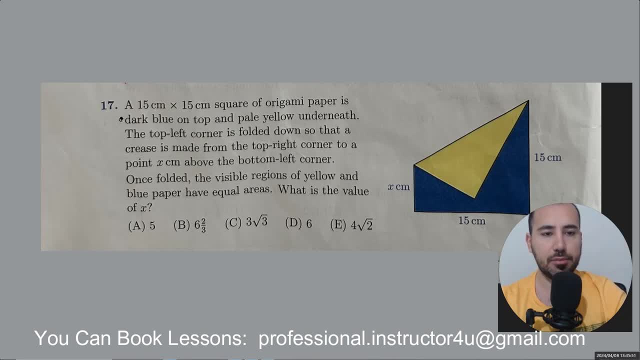 So we need to just focus on this folding part first, right Now, because it says: original was a square. let's just recreate the square. It makes sense, right? This is the first step. This is our square And if you see the yellow right. 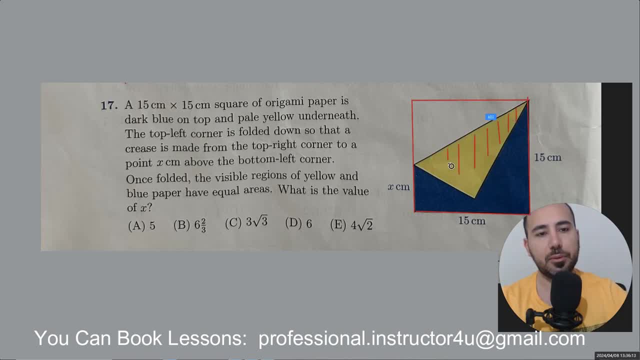 This yellow region. this is again another yellow region here, isn't it? So you fold it right, You take it here. This is the front, This is the back. They have equal areas. Okay, So it's going to have. so this is also going to be another yellow. 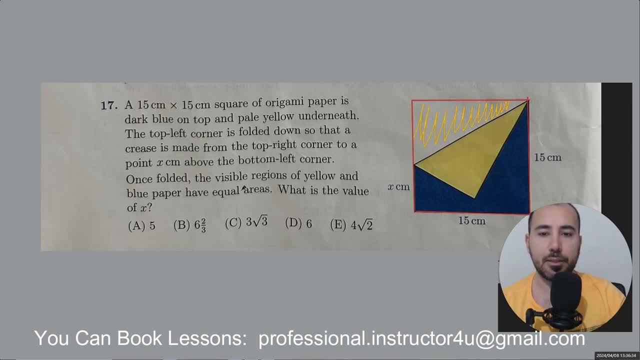 And the question says that the yellow and the blue have equal areas. So, for example, if the yellow is X, this yellow is also X, The blue is also another X. So that means we have the area of the blue part. So 3X. the total area is equal to the square, which is 15 by 15.. 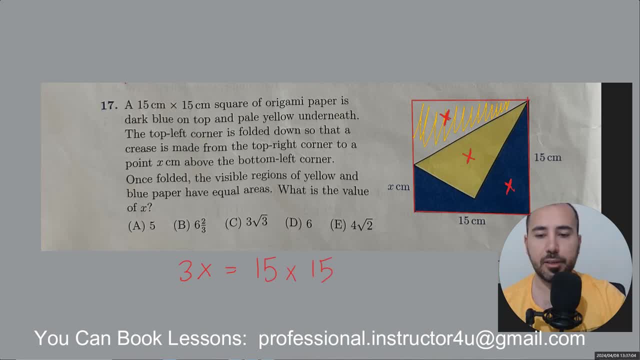 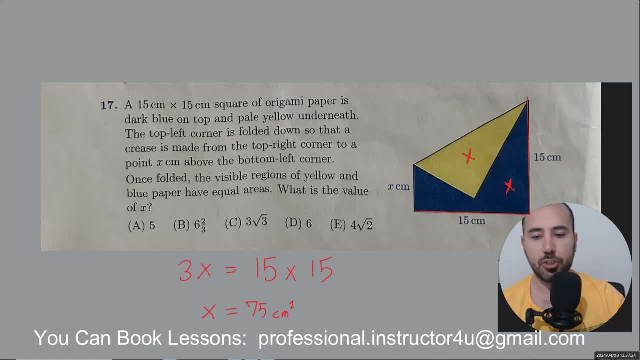 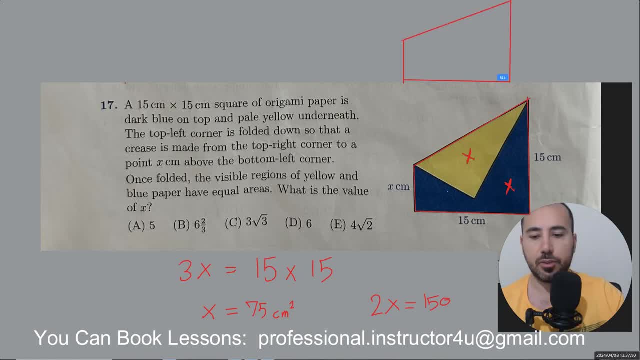 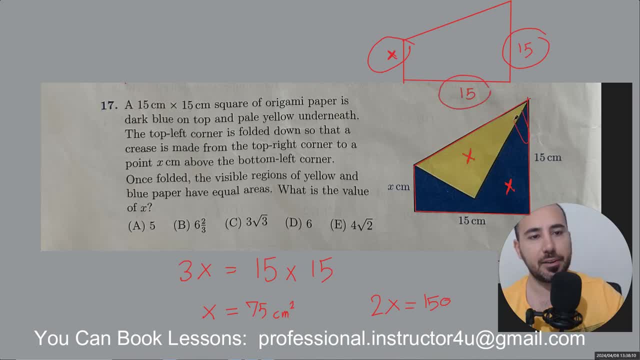 multiplied by 15, it's gonna be the area of this trapezoid, which is 150. so let's just do that: x plus 15 divided by 2- okay, multiplied by this height- we know if it's the height, because it's perpendicular to both of them- multiplied by 50 is equal to the area of the trapezoid which we have. 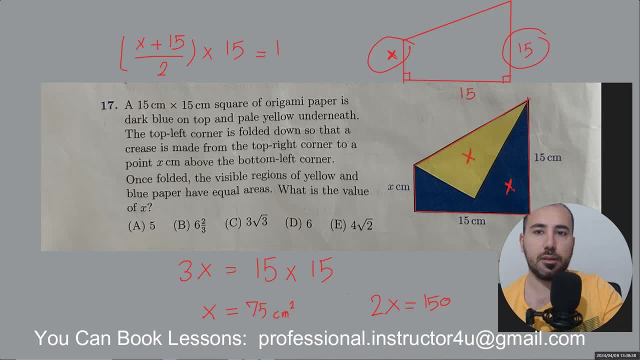 it here, 150. so how do we go about this? uh, it makes sense to divide both sides by the area of the trapezoid, which is 150. so let's just do that: x 15 and 15, a trapezoid by a 15, right? that's why we simplify them. so this one divided by 15, this one divided by 15. 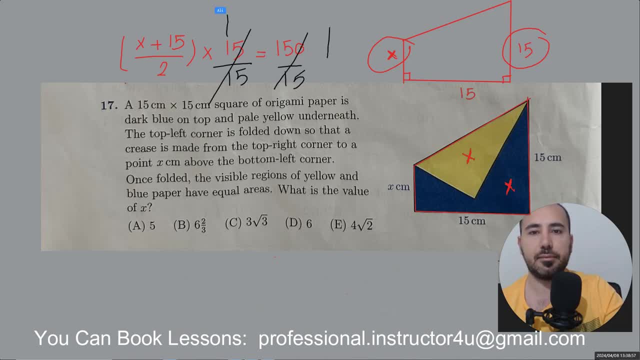 15 by 15 cancels. this is 10. okay, so let me go then. i'm going to clear this. this is going to be 10. so again we have this two. you could multiply. you may know the answer already if you don't multiply both sides by a two. 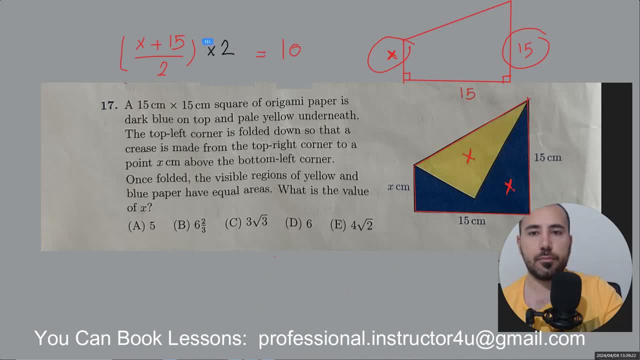 okay, this is going to be 20, of course, and the reason we multiply this by two because we could cross this. okay, then, because these are crossed, then i'm gonna clear them all. so we're gonna have: x plus 12 is equal to 20. so you already know the value of x, don't you? 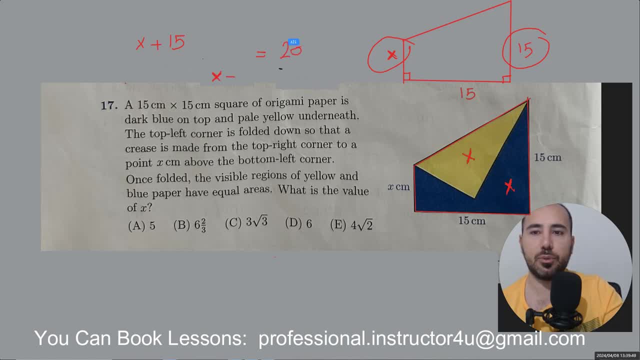 so from here we're going to have the. a value of x is equal to five. okay, so this is going to be the answer to the problem. not difficult generally, but consider this like usually, visualization questions could potentially take more of your time. well, i'm pretty sure a lot of you will have problems with. 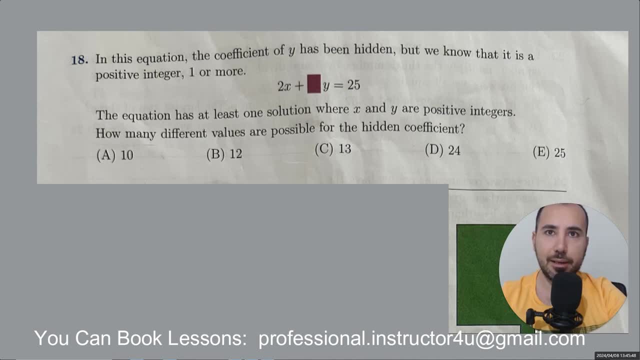 this type of questions and usually it's because when you read the question, you get confused and you get stuck. you think about it and then you leave right. let me tell you how you could break this question right and what do you do for this question. you could also apply it to other questions. 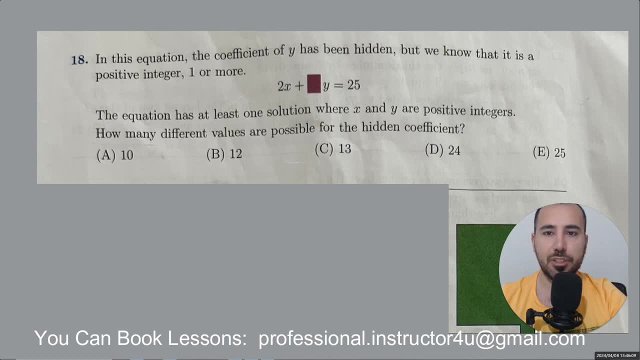 let's read the problem first. in this equation the coefficient of y has been hidden, but we know that it is a positive integer, one or more. so what does that part mean? y could be one, or it could be more, two, it could also be three, its integer. it could also be a thousand. right, okay, the equation has at least. 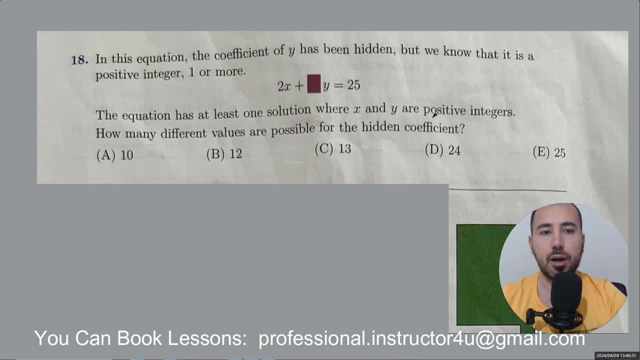 one solution where x and y are positive integers, how many different values are possible for the hidden coefficient? confused, right? what does that even mean? see, at this stage, don't just be afraid. it's so simple, you're gonna get it. you just try a few of these, then you understand what's going on. 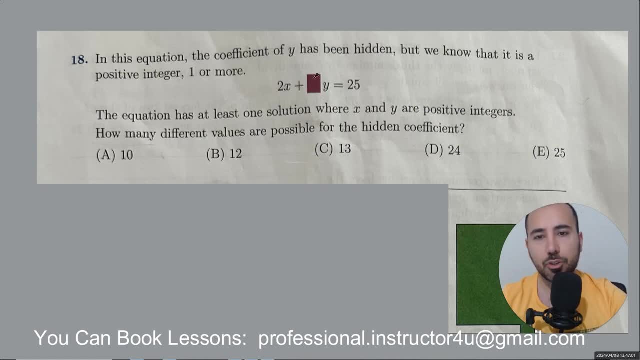 you try one, probably the smallest one, then you do two, then you do three, and then you see what happens. very easy, right? so now let's just go here. if x is y, this is the coefficient, right? the question says how many different values are possible for the hidden coefficient. is y possible? there's only. 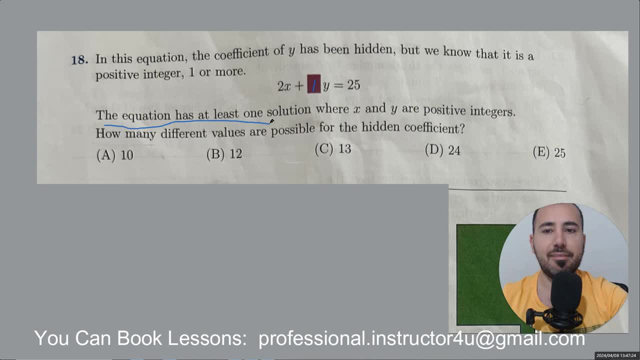 one condition here: that they need to have at least one solution where x and y are positive integers. now, for example, for here: if y is here, if x is 1, then y will be 23, right, if I give you this question here, how many solution does it have? 2x plus y is equal to 25. 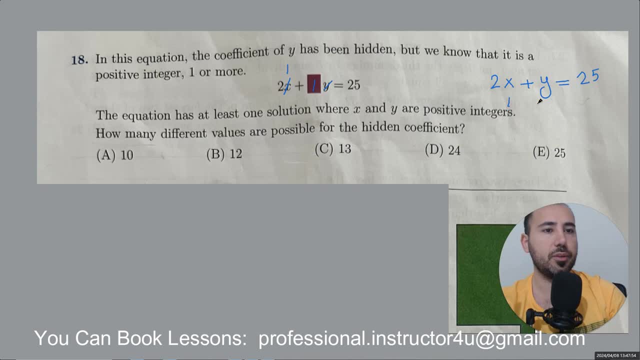 a lot of them, like: if x is 1, y is 23, if x is 2, it's going to be 21, right? so it has a lot of them. so the first answer is the. the value of 1 is good. so we we found one. well, the coefficient of y could be 1. 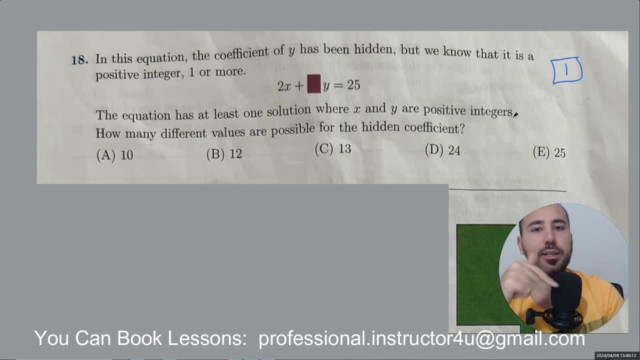 this box could be 1. so what is the next number? we need to try. can the box be the value be 2 here. if I put 2 here, and we know the y has to be a, an integer value, right? if I put here 1, then 2x, this has to be 23. 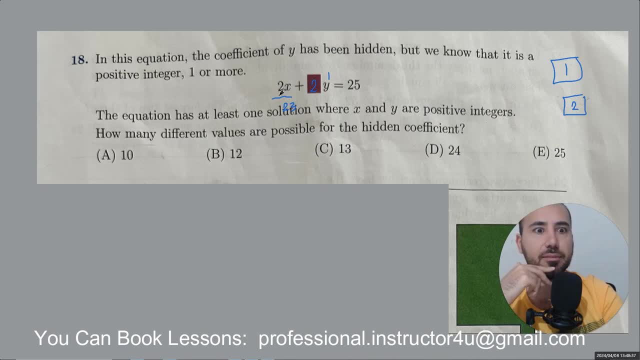 but 23 divided by 2 is 11.5, not an integer. let's try another one. so now, if y is like uh, 1, we try. let's go put a. 2, it's going to be 21. not going to work. let's try 3, this is going to be 6. 25 minus 6 is 19.. ah, so because I put here 2, this got even number. 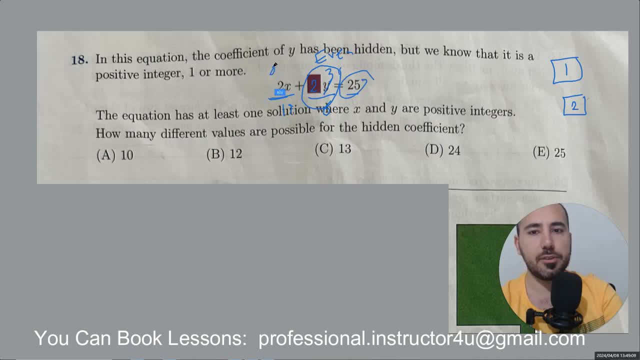 and this is 25, then this won't become odd. when we divide it by 2, it doesn't become an integer, so 2 is not going to work. so why the coefficient? 2 is impossible. one was okay, two was not okay, so let's go with three. okay, if I put three here? 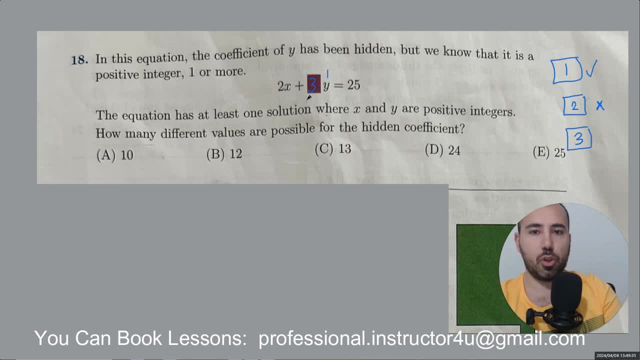 if y is one, very good, so all of this is three. this is 25, so this has to be 22.. so x is 11.. huh, it worked. so three is working. so now, what do you think about four? do you think the coefficient can? 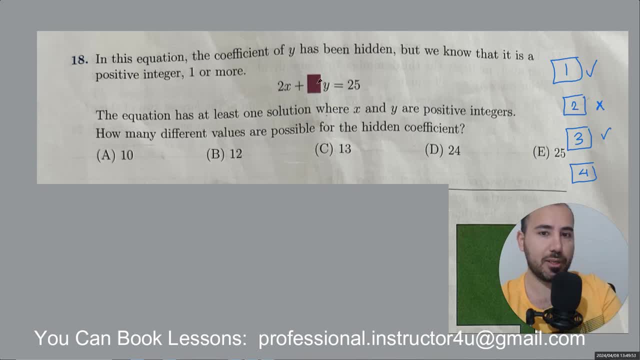 four here. no, it's going to be the same story as here. if this is four, this is one. then this is 21 divided by 210.5. okay, so now this is the time you understand the question. now this is like you can start counting. before this, you didn't even know what the question was. 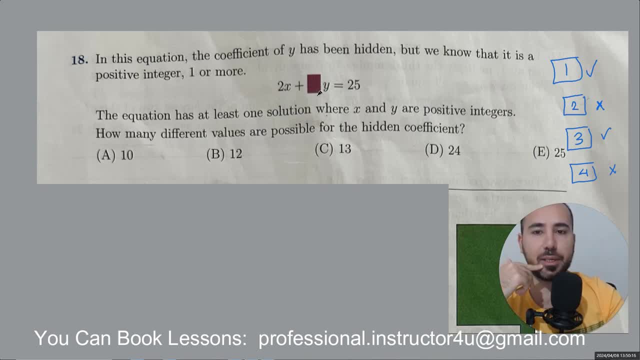 so what is the maximum value that we could get? so the maximum value, you could continue this. okay, i would say, can i put here 25, for example? let's try it. if i put 25 here and the smallest value of y is 1, then all of this becomes 25, then this will be. 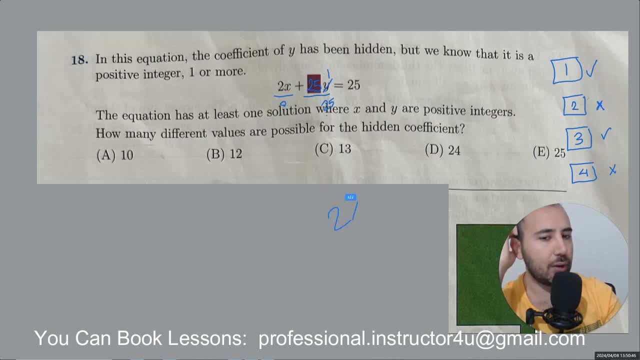 0, 0.. 2x is 0. So x is also 0.. Is that good? No, because we want the solutions to be positive. integers 0 is not positive, So 25 is not possible. So can it also be something more? 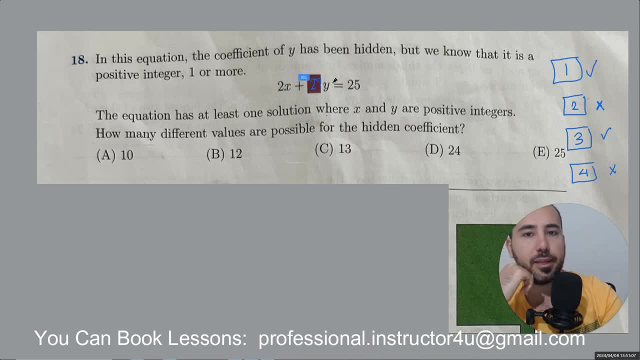 So like 27.. If y is 1,, then this will be negative 2.. Is that good? No, because it's got to be negative. So let's try 23.. Okay, if you put 23 here, y is 1.. This is 2.. x is 1. And it's going. 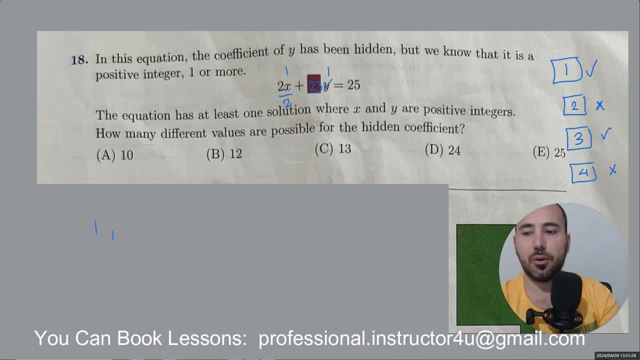 to work. So that's going to be the answer. The answer is going to be like all the odd numbers: 1,, 3,, 5,, 7.. Just write them all or just count all the way to 20.. Okay, 3.. So maybe you count them or? 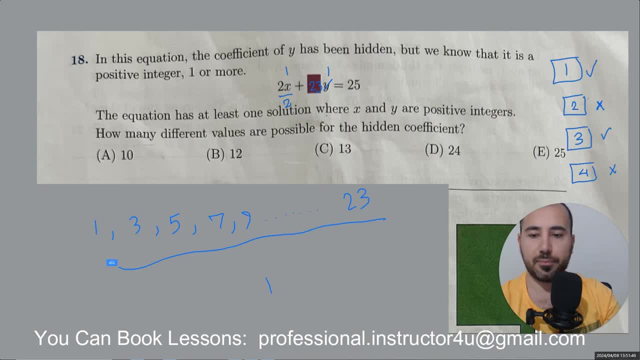 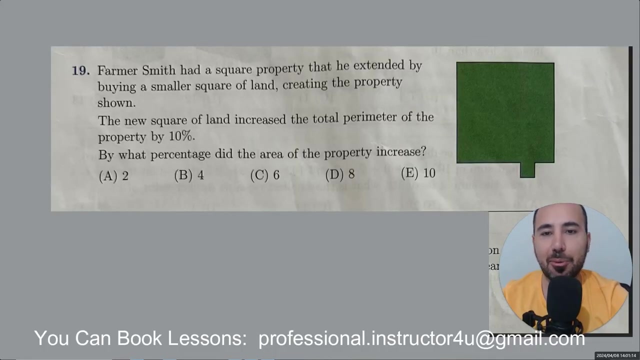 however, you know this is going to be 12 of them here. Okay, so the answer will be B. Such an easy question If you do it the right way. if you do it the wrong way, really difficult. so farmers mayor had a square property that he extended by buying a smaller square of. 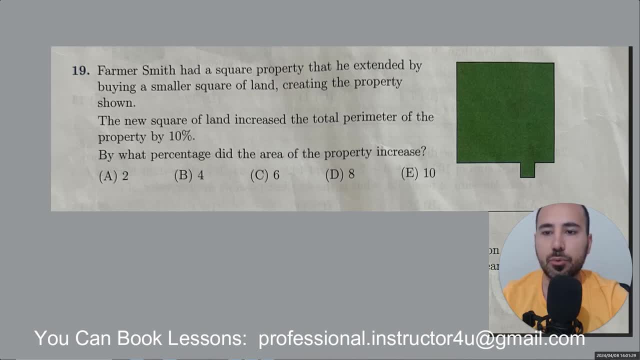 land creating the property show. the newest square of land increased the total perimeter of the property by 10, but what percentage did the area of the property property increased? so i have a question for you: how large is this side of the square? how large is it? so they didn't give it right. why do you think they didn't give the side of the square? 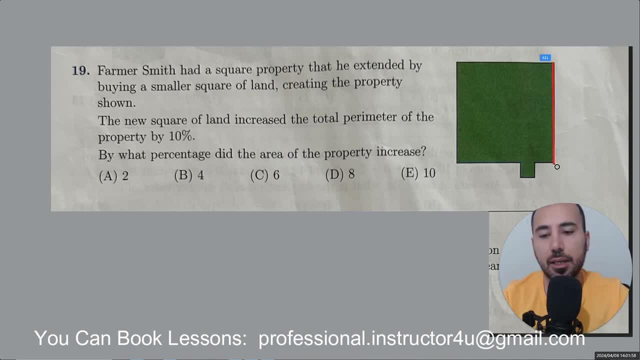 because it doesn't matter. so if the side here is one, the answer wouldn't change. if it's a thousand, it wouldn't change. if it's a square root of three plus infinity, divided by two, to power of n, and n is again, n is three, it's still, it wouldn't change. 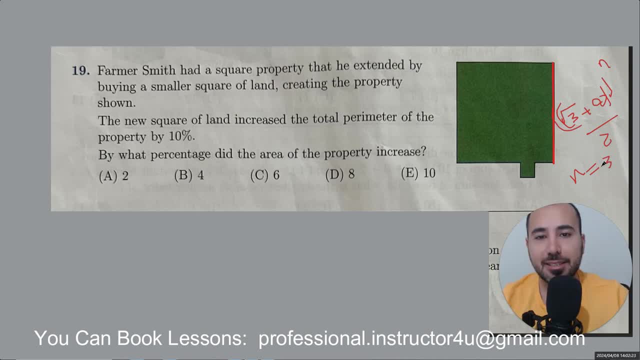 right. so what is the simplest value you could write? do it with that value. okay, i'm gonna choose 10. now, now one, i'm gonna choose 10. so if this one is, if this side is 10, then the original, the original perimeter was four times 10, 40.. 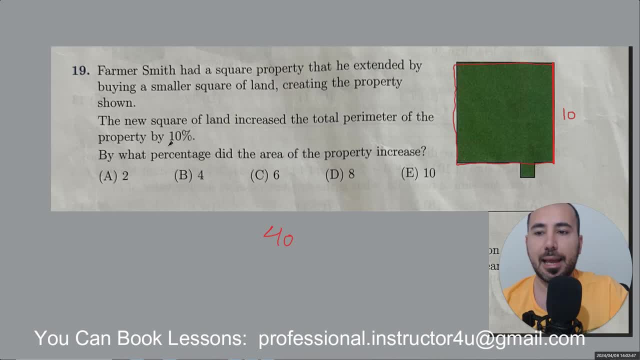 okay, and then it increased by 10. what is 10 of 40? 10 percent? you simplify it, that is 1 to 10, right? so what is one tenths of 40? you multiply it by one tenth, the answer is four. okay, so the perimeter was 40, now it is 44 after this part is added. so how large is this side? 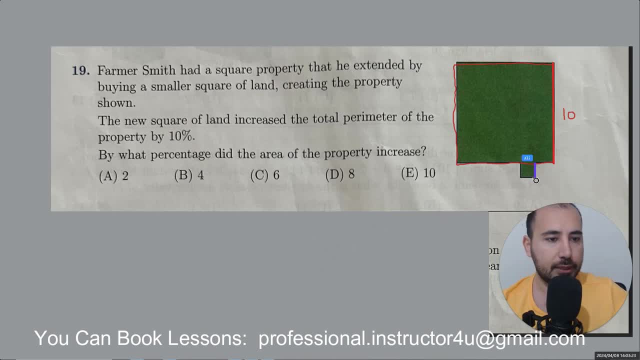 see, now, when we have these three sides added to it, the perimeter is 44. so that means this side over here, each side, should be two, two, two. so what is the perimeter now? okay, so what is the perimeter now? the perimeter is 44. now don't tell me it's gonna be okay 40, and then it's gonna be three, twos, it's. 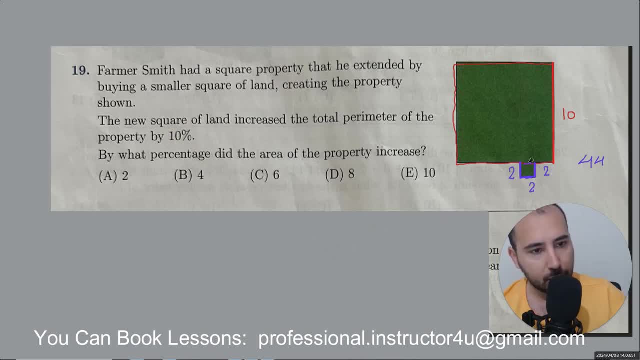 not. okay one. this one is equal to this one. we already had this. the ones that will be added are just this side and this side. so the new perimeter is 44. so if this is 10, each side over here is two. okay, so then by what percentage did the area change? so the previous area was 10 by 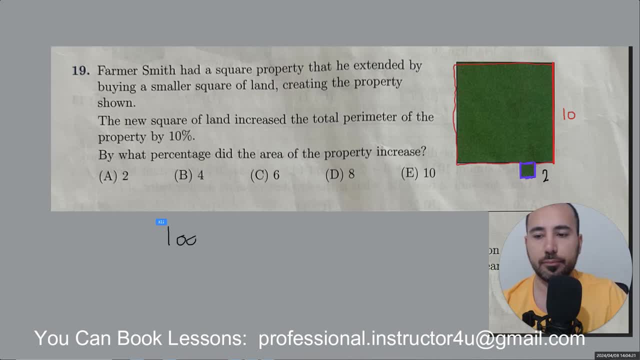 10.. so it was a hundred. now the new area is the same: 10 by 10, 100 plus the area of this little thing which is two by two, which is four. so what is the amount of information that we have right now? okay, what is the increase? 100 turned into 104.. so what is the increase? 4? 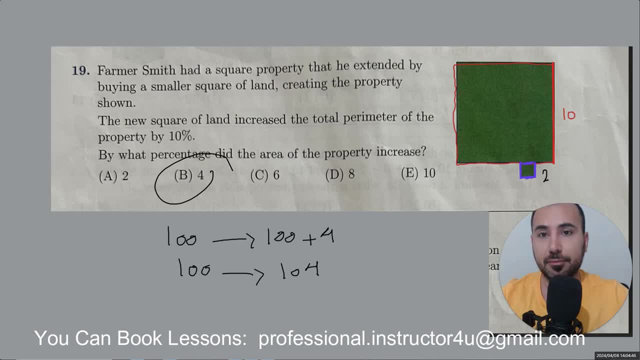 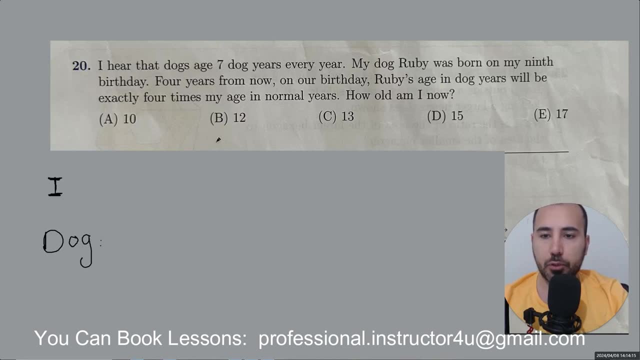 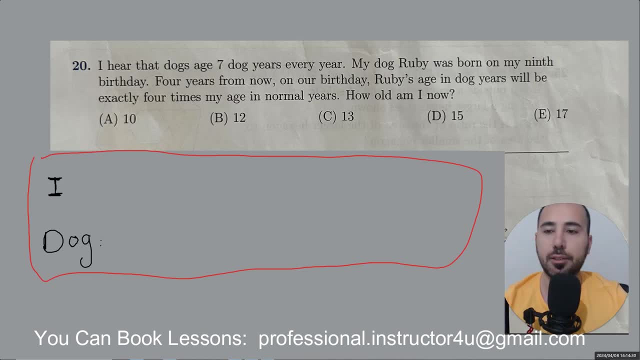 yet then i would suggest that you just make a chart instead of writing equations. so, for example, i hear that dogs age seven dog years every year. my dog, ruby, was born on my nine's birthday. so when i was nine years old, my dog was zero years old. okay, four years from now on. 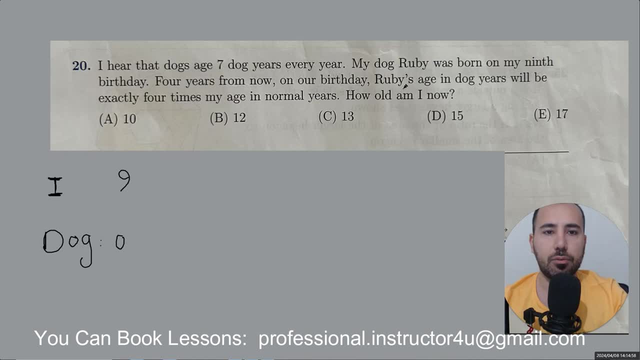 our birthday, ruby's aging dog years, will be exactly four times my age in normal years. how old am i now? okay, so let's just complete this diagram a little. one year later, i am ten, but my dog is seven when i'm 11. this one is 14.. this one is 12, then this one is 21.. see, it's already. 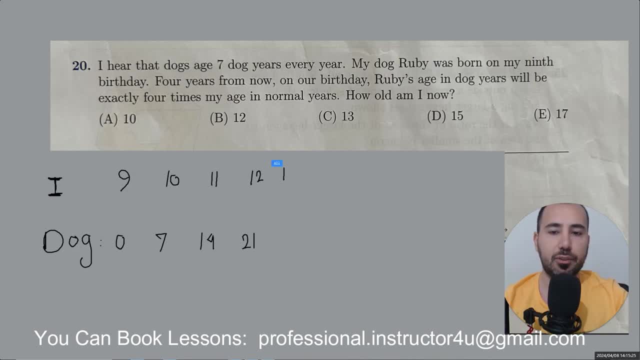 close to two times more the dog. so this one is six is 13, again 28, this is 14, this is a 35. so you could just continue this, okay, or you could just write an equation up to you. so here it could be 15, this one would be 42. you just should continue this. 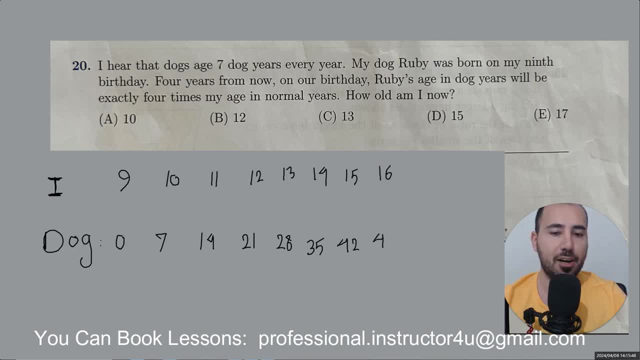 when this is 16, then this one is 49, almost three times, now a little longer. when this is 17, this is 56. when this is 18, then this is 63. when this is 19, okay, this is gonna be 70 when this one is, uh, 20. it's gonna be on my head, it's gonna be. can i write on my head? 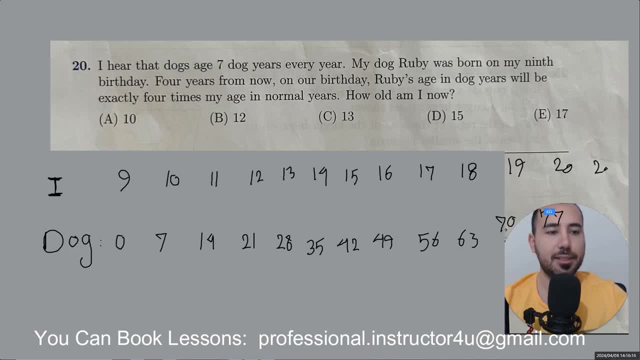 yes, i can. it's gonna be 77 when this is 21. okay, this is gonna be 84 and this is what happens. okay, this is the answer. okay, but here it says four, four years from now this will happen. okay, how old am i now? it's gonna be four, back one, two, three, four. so this person, i- is 17 years old. 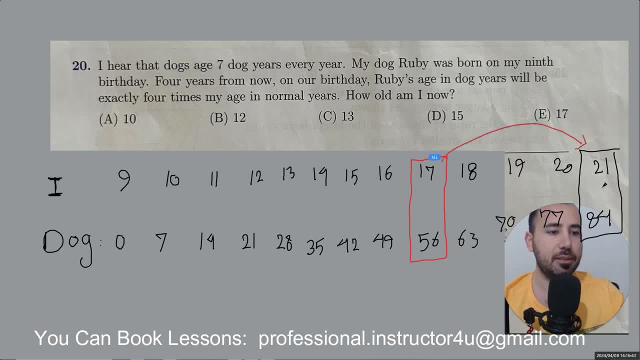 right now, four year later, it's gonna be four times. if you divide this one by this one, it's gonna be four years. okay, so basically, uh, this is a diagram, but if you can visualize this, you could also write like an equation. so so for us, for example, 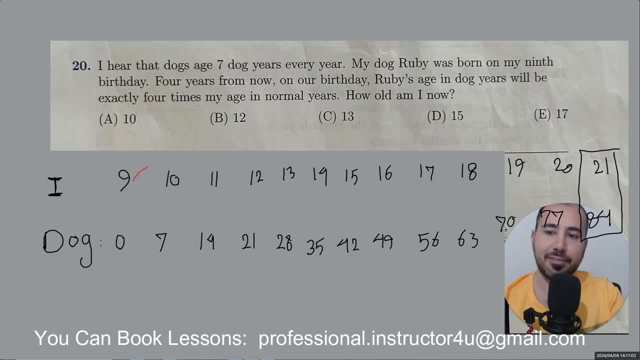 here. how many years is this? you would say. if this one is the, how many years later? so instead of a number, you could put a variable: how many years later? okay, but this one will go by seven. this one goes by one. this one goes by seven, so the amount of increase of the other one is actually. 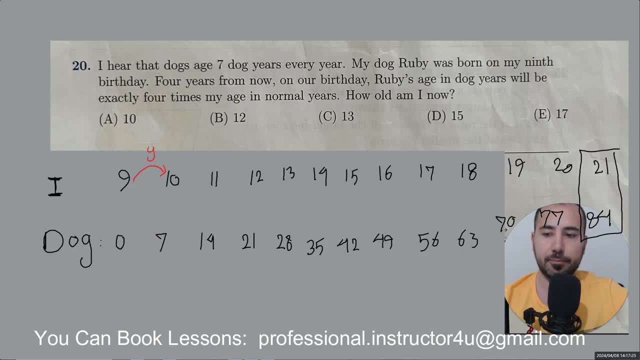 if this is y, this is seven y, so it's going to be seven y. so this is person: start from zero. the dog i starts from nine. let's just write an equation: nine is added by one each year. the dog starts from zero, but is adding by seven y. so that's the equation. 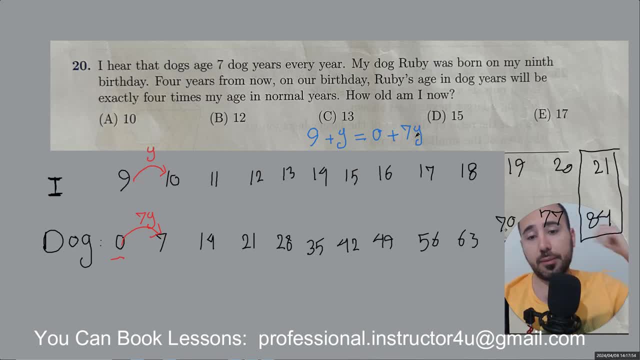 okay, but we don't want them to be equal. we want the ratio to be four, like this, okay, so then we add the ratio to the smaller one. right, i'm gonna be smaller. so if i give this four, both sides of the equation will be equal. so if i go and expand here, i'm gonna maybe write it here: it's gonna be 36. 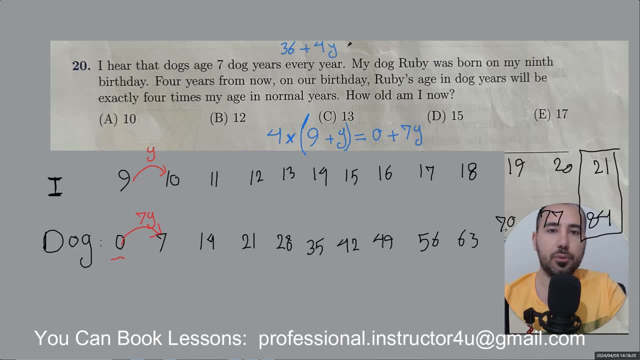 plus 4y is equal to 7y, 7y, 7y, 7y, 7y. so then y from here will be 12. and what is this 12? it's going to be all this big increase from 9 to 21. that's going to be 12, but remember, we still want four years back, so the answer will be 17 nonetheless. so which one you use is up to you. okay, so this is this. may take a little longer, but it's safer. okay, but if you're good at writing equations, go with this. it's fascinating. 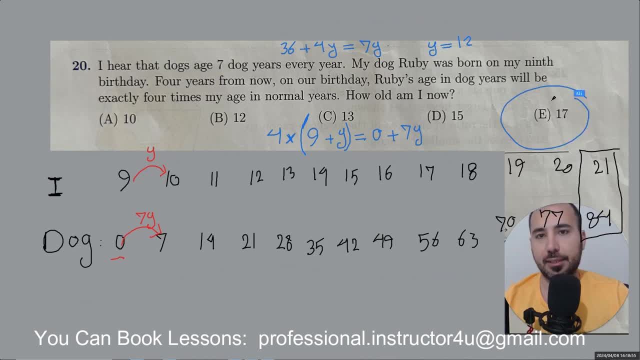 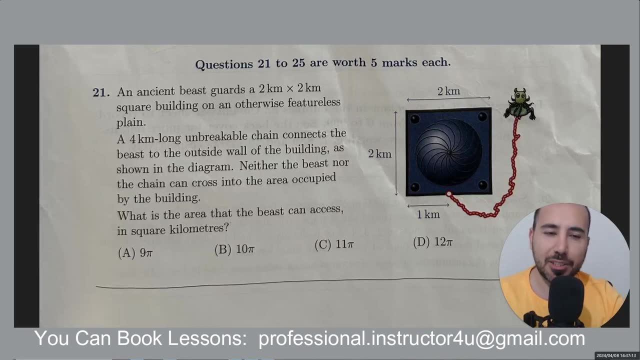 there. so, nonetheless, the answer is 17.. okay, problem 21: uh, it's again requires a little visualization and like drawing the path, so you know that it's gonna take more time than the other questions. uh, that we did and we're gonna do. so. let's see and let's read the problem here. we have an asian beast guards, a 2x2 square building on a. 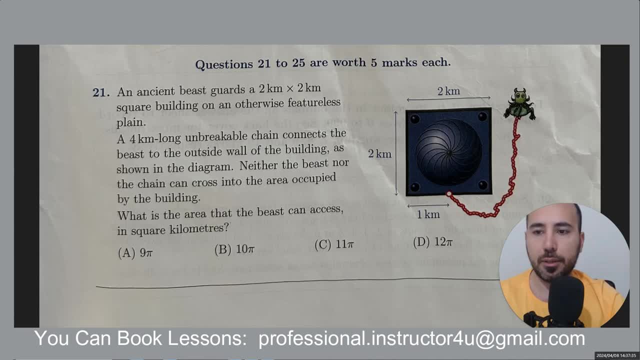 otherwise featureless plane. a four kilometer long unbreakable chain connects the beast to the outside wall of the building. as shown in the diagram. neither the best the beast nor the chain can cross into the area occupied by the building, so that means this beast cannot go inside the 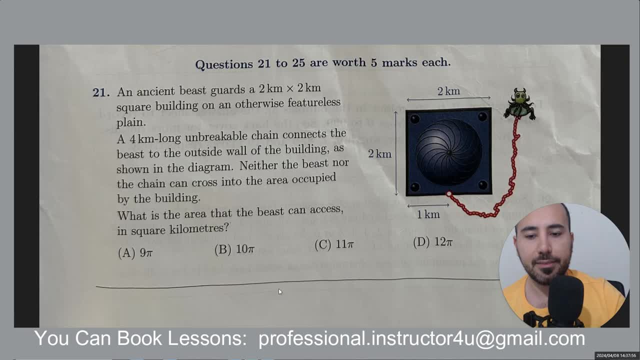 building. the beast cannot be here. and even the chain like this, it can't actually go inside. so the beast cannot be like this, you could only go around. so if the beast wants to go here, the chain will has to be straight and then go here. okay, now what is the area? 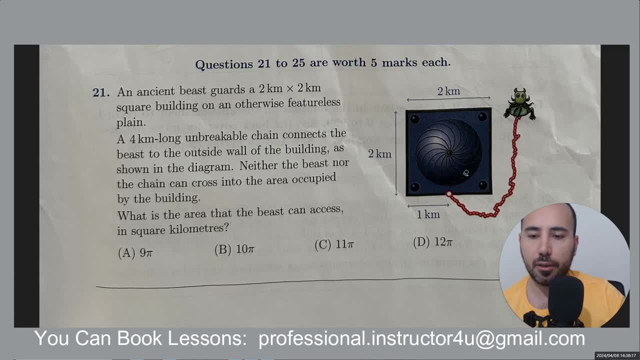 that the beast can access in the square kilometers, because in the answers we have pi. that's also a hint. we're going to use circles, and what is the area of circles? pi radius squared, that's the area and this is the formula we're gonna use. okay, so let's just go and see where the beast can access. so 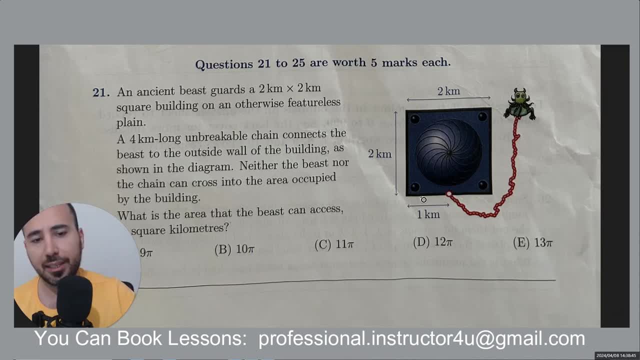 the chain is four meters. if the chain says i'm gonna go only left, right, if the if the beast decides to go only left, that's gonna be four. like this: if say, okay, i'm gonna go only down, four kilometers down, if it's, i'm gonna go only. 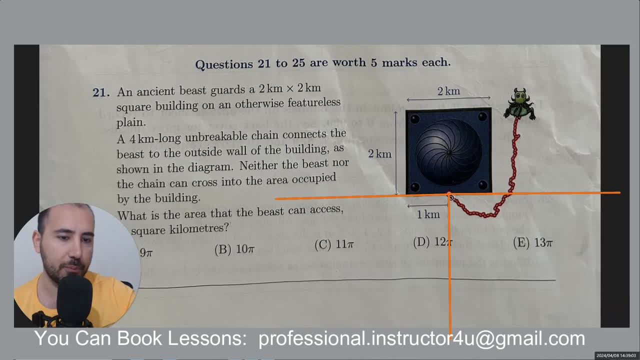 right, four kilometers. right, we could also go. the beast could decide to go in any of these directions that it wants. okay, four meters so, and this is going to be the radius of a circle, so the beast can access any of this area. so what is this? like a orange area? let's just do this. we know that the radius is four. 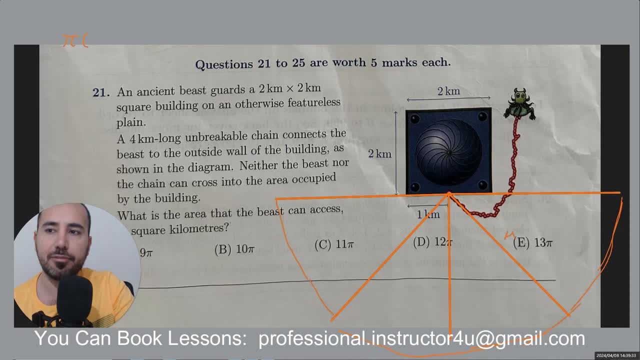 so the area of a full circle would be pi 4 squared, and since it's a semi-circle we need to divide it by 2.. so that's going to be 16 pi divided by 2- 8 pi already. so now let's see other points. if 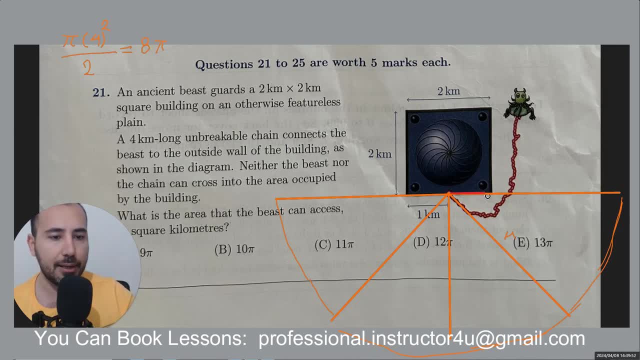 it decides to go up. if it decides to go up, it's going to waste one meter like this and then it has three more meters. it could go completely up. three meters up. it could still go three meters right from here. it could go three meters everywhere it likes to go. three meters, three meters, and 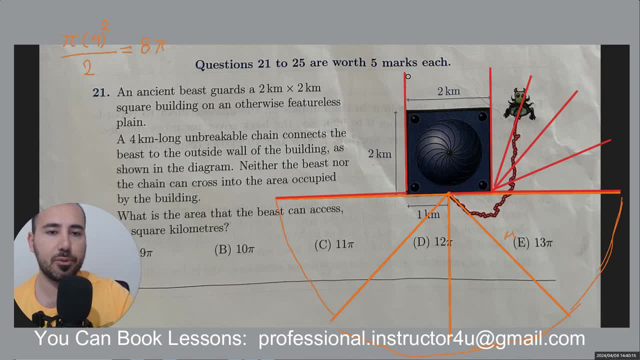 whatever happens here, it's just happening to the left side. it's going to be completely symmetrical, since we're just dealing with a square. okay, so then that's going to be like this. that's going to be another semicircle. when we added them: this is a quarter, this is a quarter. 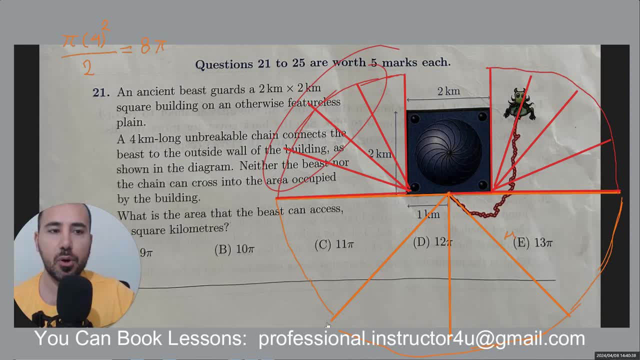 this is quarter the red ones together they make a semicircle with the radius of three. so i'm gonna go pi. three squared divided by two. three squared is nine. divided by two is four, four point five. so the red region is going to be four point five pi. 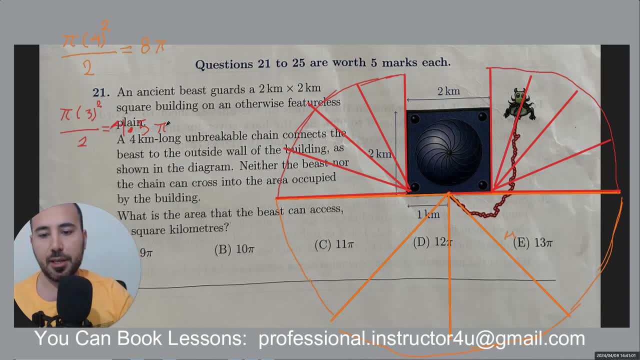 is there something that we haven't dealt with? yes, because after going up see, this is one meter here. right, two meter here. we still have one more meter to go. so it could also decide this one meter to go anywhere it likes in any of these directions. so 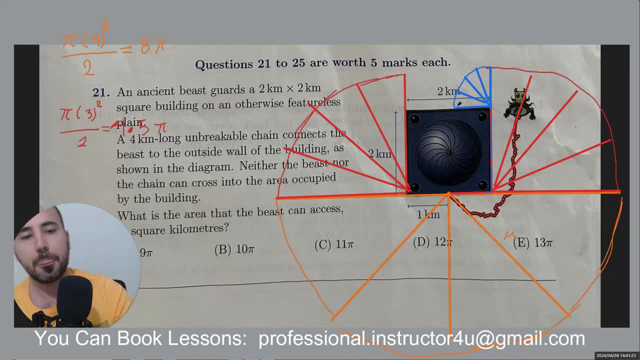 that's going to be a quarter of a circle with radius one, and then another quarter of a circle with radius one. okay, so one, one, one, one. so it's going to be again pi, since the radius is only one one squared. this one divided by two is only half zero point five pi. so you tell me let's add. 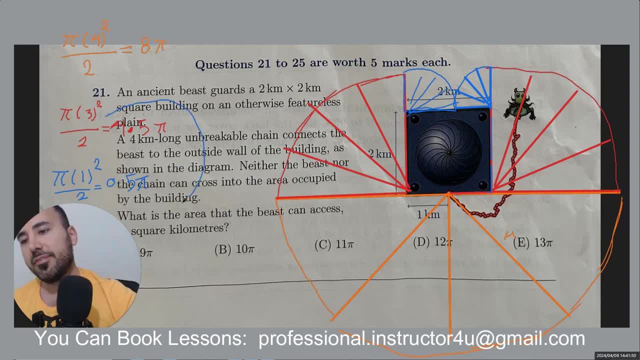 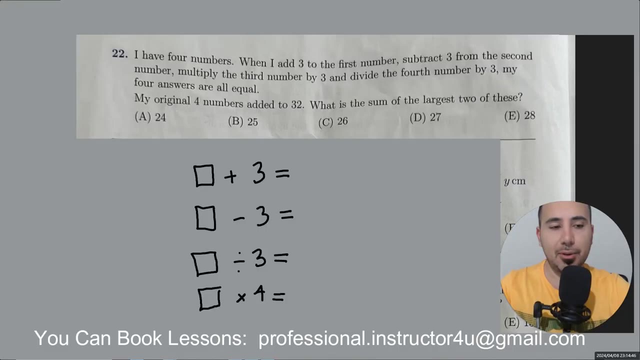 them together: four point five plus point five is five pi, eight pi and five pi are thirteen pi. so this is the right choice. okay, this problem is actually kind of easy to be- problem 22- and you must definitely get this if you can just watch it like you need to learn two ways to get a problem like this, and i'm gonna. 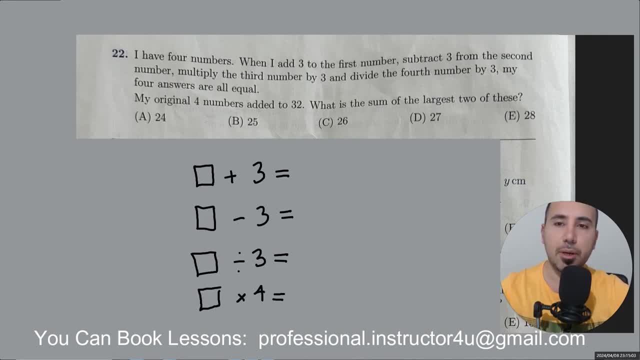 teach you two ways to do that. so i have four numbers. when i add three to the first number, okay. or subtract, okay. or divide it by three, or multiply it by four, okay, all these numbers multiplied before fourth number by three. i got a mistake here. the fourth number. when you multiply it by by three, all of them become the same number. now 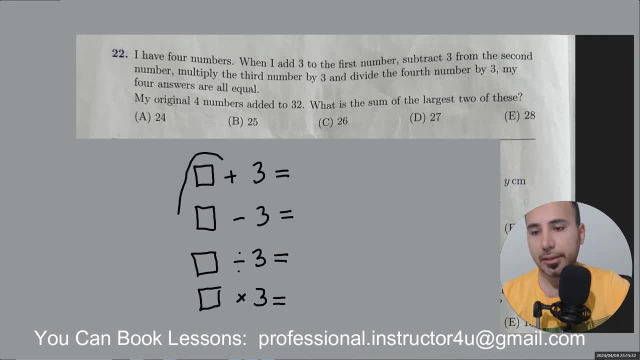 um, the sum of these numbers that are here is 32, and what is the sum of the largest two of these them? okay, so one way would be by guessing, and probably it's even a better choice. um, let's go here, i'm gonna go right here. eight, so all of them should be eight, eight, eight. 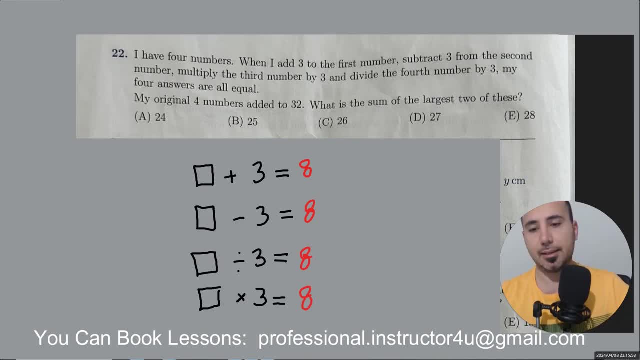 but look, if i choose eight is eight divisible by three. okay, so for example, here this one: what number should i write? that i multiply by three becomes eight. okay, it's going to be a decimal value. so what does that tell us? this number over here should be a multiple of three, for example. let's go and try this. for example, three is not going to. 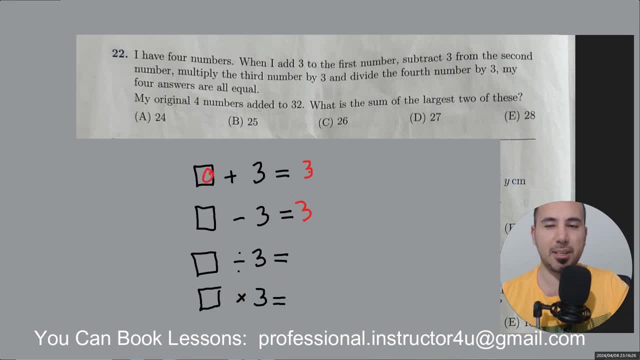 work because, okay, this number, then it becomes zero. so let's see something else. i'm going to start by guessing, and probably it's going to be a decimal value. so let's see something else: six, six, six, six. okay, then this number was three, this number is nine. this number was 18. 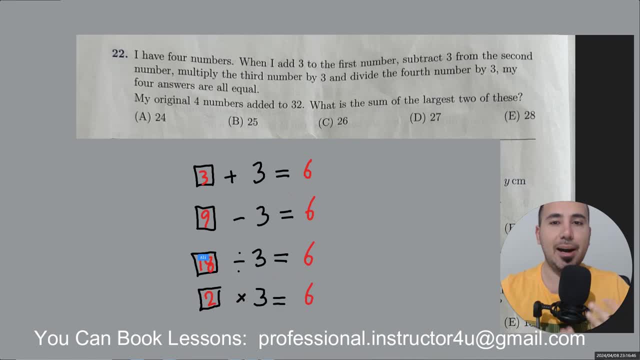 and this number was two. now i add them up. if this sum is 32, i've already answered the question. let's go and add them to 18, 20, 29, 32. i got the answer. now what is the sum of the largest two of the? 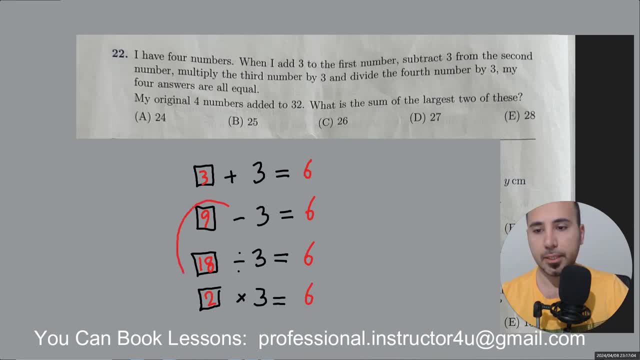 these. it's going to be these two: 18 and 9, 27, really easy, okay. and because it was a multiple of three, you don't have a lot of choices: maybe it's three, maybe it's six, maybe it's nine, because you know, the sum is not really that large. it's around this and it's a multiple of three. okay, if six didn't. 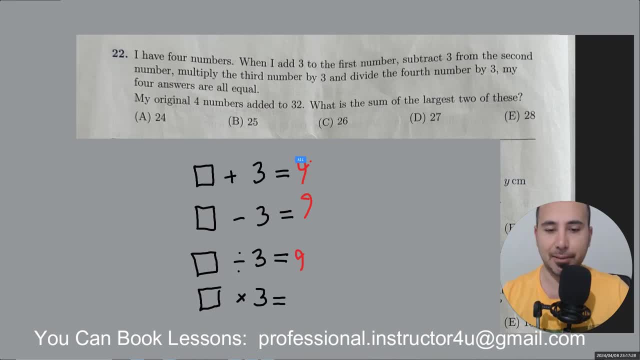 work, then i would just try nine, easy peasy, okay, so that's the best way to do it and we already got the answer. the other one would be just writing all of these a. we assign a variable. okay, then this one here will become a minus three. this number becomes a. 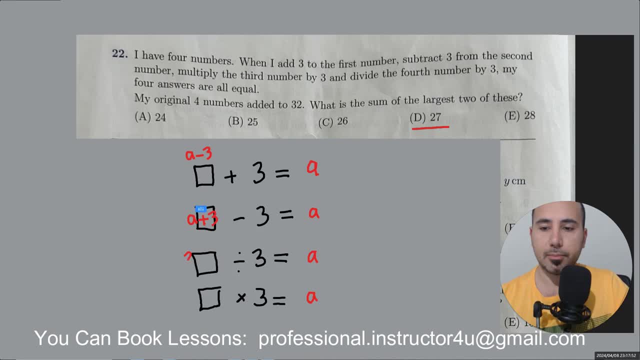 plus three, this number becomes three a, because three a divided by three is a and this one is one over three a. okay, so now the sum of these is actually 32. so i'm not gonna actually solve this, i'm just gonna show you a minus 3, a plus 3 plus 3a plus a over 3. okay, all of this is 32. okay, maybe we could do. 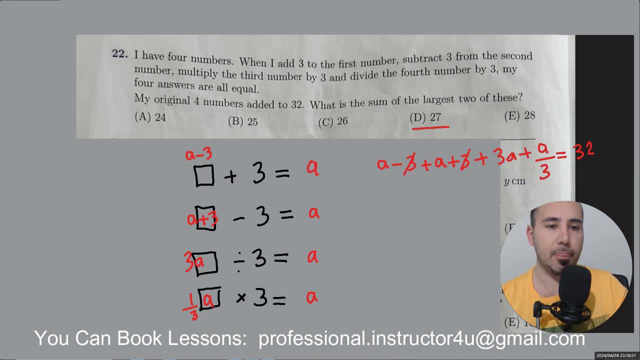 so these are cancelled right over here. so we're gonna have 5a plus a third is 32, so we could see that the a is actually like 6 from here. okay, so if a is 6, just you just have to replace. then you get this number 18 here and this, you get your 9 over here. 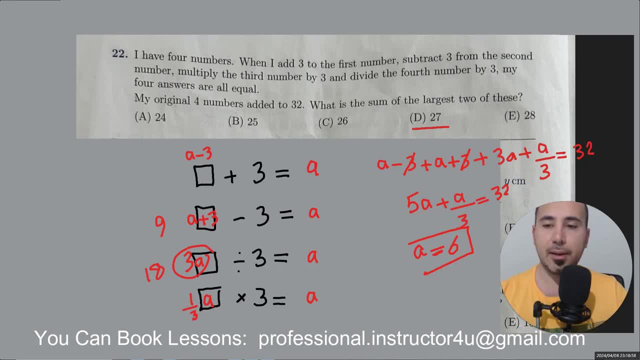 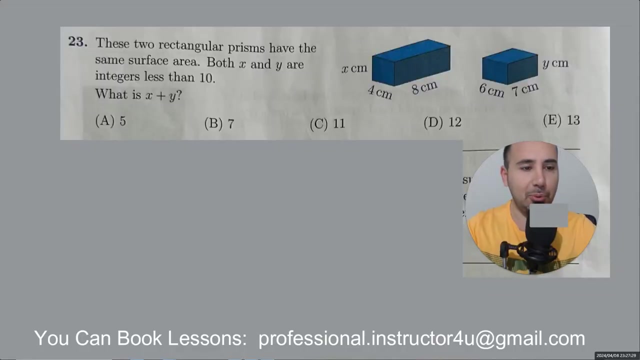 okay, so this is like two-way, but I would encourage you to start one or two examples first before you just try all these variables and equations. okay, so, either way you choose, it depends on your skill level, your preference. I both are really good ways. another problem that is doable, nothing really difficult. 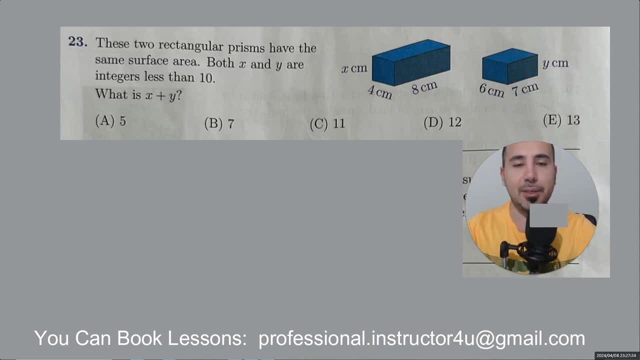 about this one. anyway, let's go through it and see how this is done. these two rectangular prisms have the same surface area. both x and y are integers- less than 10. what is x plus y? okay, so the first thing to note is that we have, from each okay shape that we have here, we have two of them, so we have 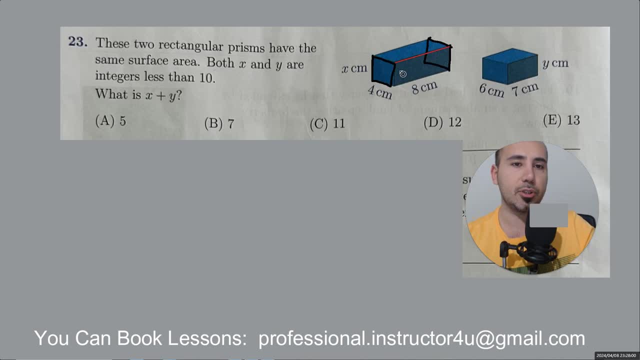 two of this, okay, and then we have two of these, and then we have two of these, and then we have of this, Okay, And there is going to be like one here in front of it. So from each one we're going to have to see, the way to save time is just going to be a writing, one from each side, and then say: 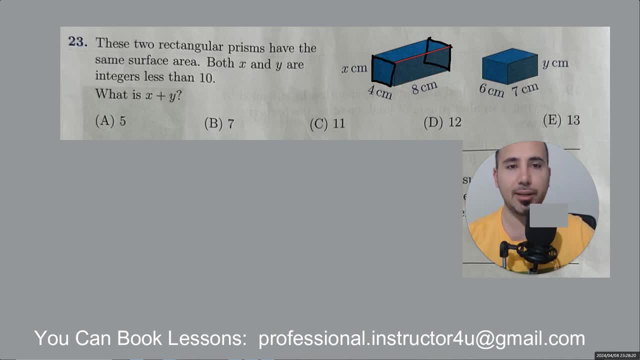 they're equal. But I'm not going to do that here, because I want it to be simple to understand for everyone. Okay, So what is this area here? This one, this one, it's going to be four times X and we're going to have two of it. So I'm going to have four X, Okay, But we're going to have two. 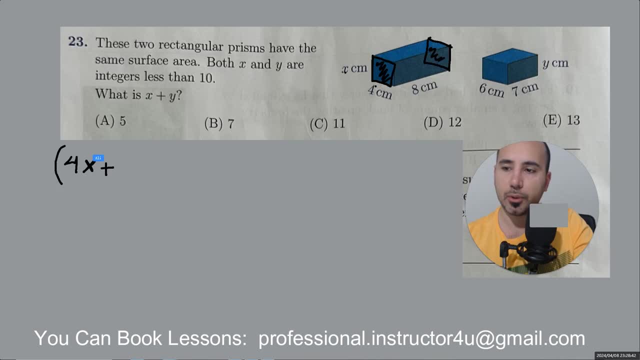 of this. Okay, So I will multiply this by two. right over here We have two of this, four X. Now let's go see the other one. What is the area of this part right Over here? this one again. we're going to have two of this. One of them is eight times four. 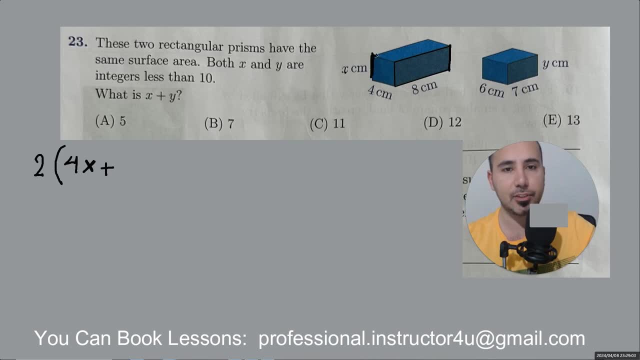 No, sorry, Eight times X, because this is X, So is this X Again. we're going to have two of this. And lastly, okay, we're going to have two eight times four. It's going to be this one at the. 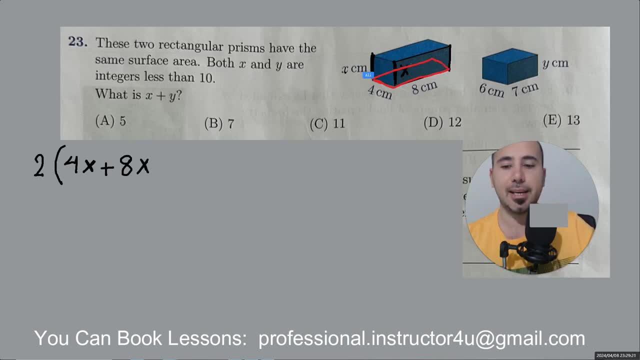 bottom here It's going to be right here. This one is eight times four, And again we're going to have two of this, See. writing this is unnecessary because later it will be canceled. Now let's focus on the other one. This is okay. Y. This is six. Okay, If this is Y. 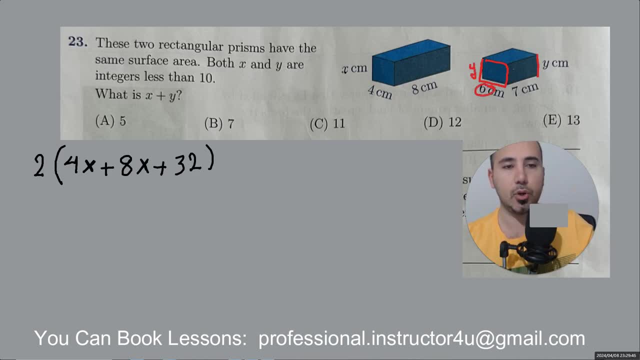 so is this Y. This is also six. So this one is going to be equal to two Six Y. And let's see it here. We have done that. So how about this one? This is seven Y. And lastly, we're going to have this one If this is seven. let me change color If this is seven. 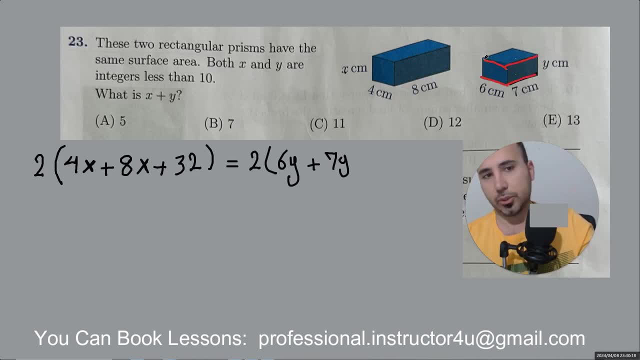 this is also seven. If this is six, this is also six, And this is a rectangle, right? So this is six times seven, So it's 42.. There you go, And you see. now these two are actually canceled. Bang bang If I divide both. 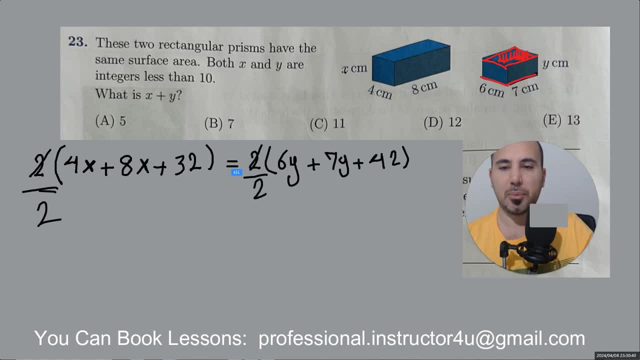 sides by a two, that is, both of them are really canceled, So I don't really have to worry about them. So I'm going to cancel them from both sides. I'm actually going to clean them from both sides. So you cleaned. 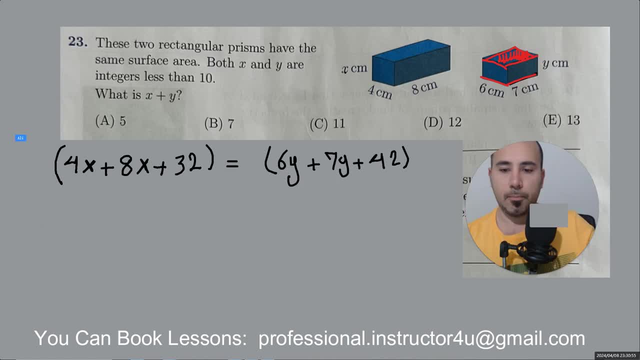 And this is also cleaned. Okay, From here we're going to have 12 X plus 32.. And the right-hand side, these two are 13 Y plus 42. Okay, So I have two numbers. I don't like. I just want to have one number on any side To do that. 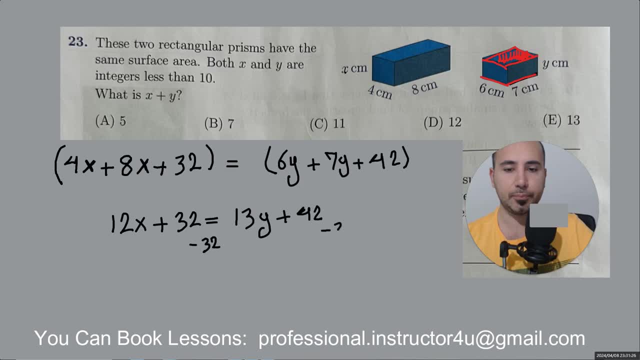 I'm going to minus both sides by a 32.. When I do this, this is canceled. 42 minus 32 is just a 10.. So, bye-bye, 10.. Okay, So from here we could practice with different values. We know X plus Y, We want. 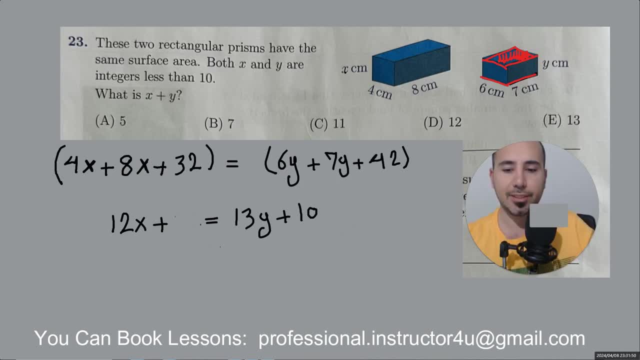 X plus Y, And we know they're less than 10.. So let's just start by the simplest one. If Y is one, this is going to be 13. This will be 23.. Is 23 divisible by 12? No, It's going to be. 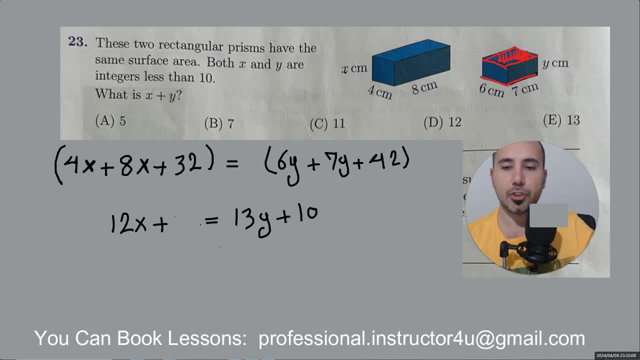 1.9 something. No, If this is two, this is 26 plus 10 is 36.. Is 36 divisible by 12?? Yes, Let's see how. So if this 36, Y is two, 36 divided by 12 is actually three. Now the equation is true. holds true for X being. 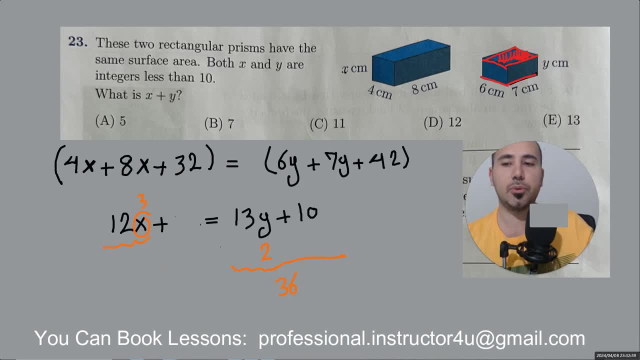 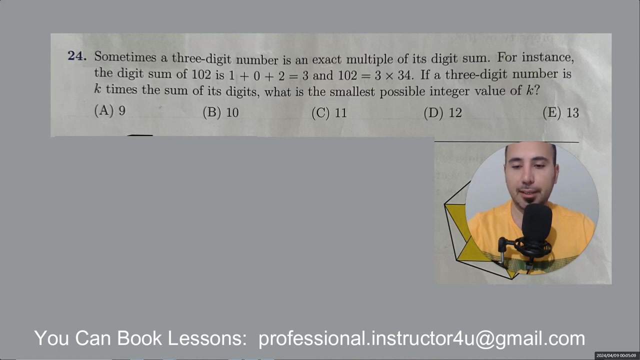 three and Y being two. The question wants X plus Y, So five is the right choice, Not difficult, especially for problem 23.. It's not very difficult Now. little by little the questions are getting more difficult. Okay, So one thing that could help. 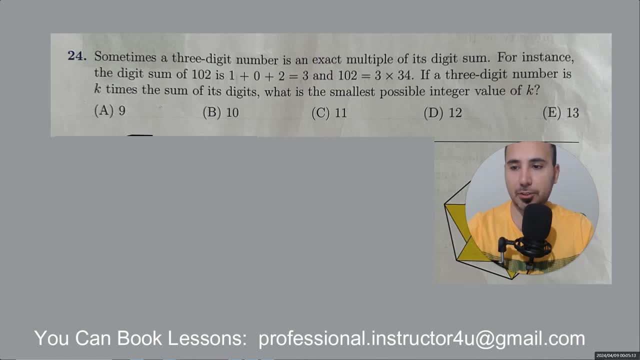 you to deal with a question like this is this: So, for example, if you have this number 345, see, I could write it as three times a hundred plus four times 10,. right, Because four is in the tens digit and five is in the units digit, right? 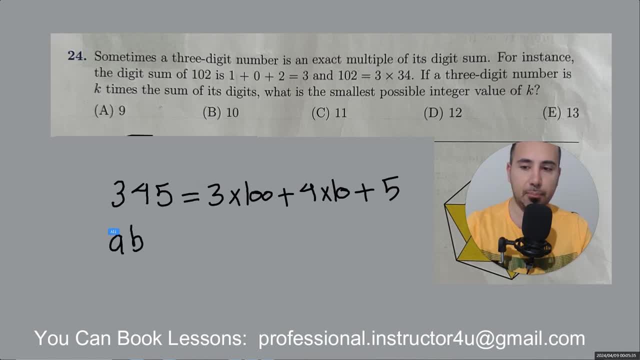 So then, if I change the numbers into variables, this A is in the hundreds position, So I could write it as a hundred. A plus B is in the tens position plus C. Okay, So we're going to use this format to be able to do the question more easily. Okay, Now let's read the problem first. 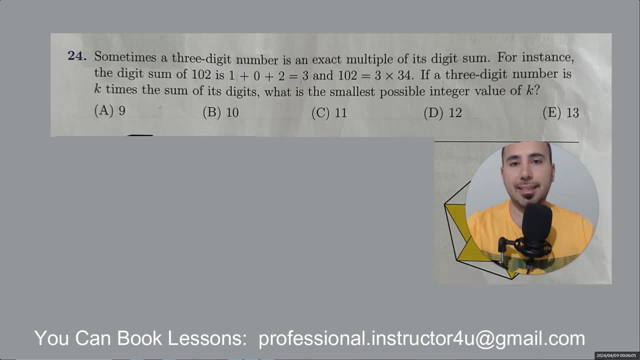 Sometimes a three-digit number is an exact multiple of its digit sum. For instance, the digit sum is 102.. Okay, Let me write it here. And when you divide 102 by its digit sum three, you get 34.. Now here it says: if a three-digit number 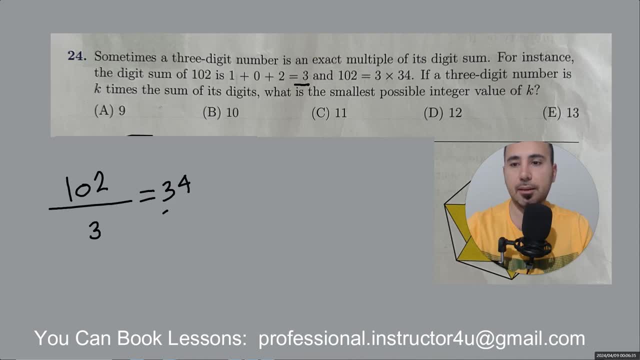 is K times the sum of its digit. okay, it's going to call this one K, What is the smallest possible value of K? So we want to make this really really small. So how would you change this number to make it a small? How do you change it to make it really really big? 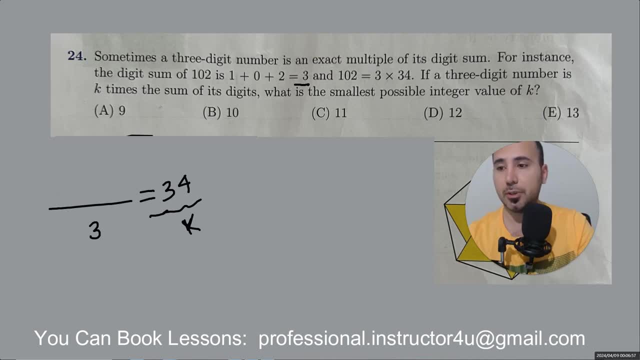 So the way I would make it really large, I wouldn't write it as writing these 900.. I would write this as writing the K. Okay, So I'm going to make this 100-100 divided by this And dividing this by nine. see, that's one way to make it really really large. Now the K is a hundred. 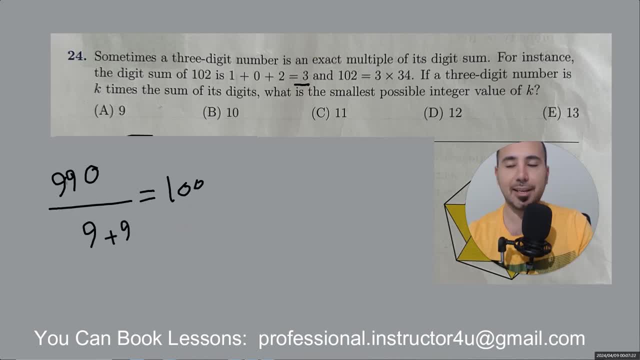 So if I make this 990, but the digit sum becomes nine plus nine, What happened to it? is it getting more or less? It's getting less, right, Okay, Okay, Okay, Okay, until you know what's going on. but now we want to make the K value really small. 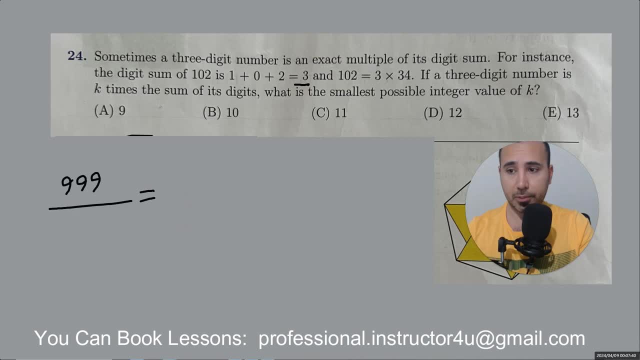 okay, if I write all the numbers big, what happens? 999, it's going to be 37. so how can you make this? now, the goal is to make this really small. the numerator should be really small and this one has to be really large. keep it as large as. 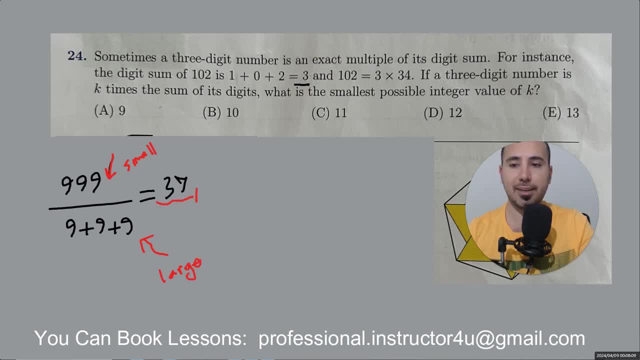 possible? this way, you will minimize the value of K. okay, so to make this really smaller. which digit are you gonna change? this one, this one or this one? I'm gonna change the hundreds digit, right, if I turn the hundred digit into a one digit. I'm gonna change the hundreds digit, right, if I turn the hundred digit into a one. 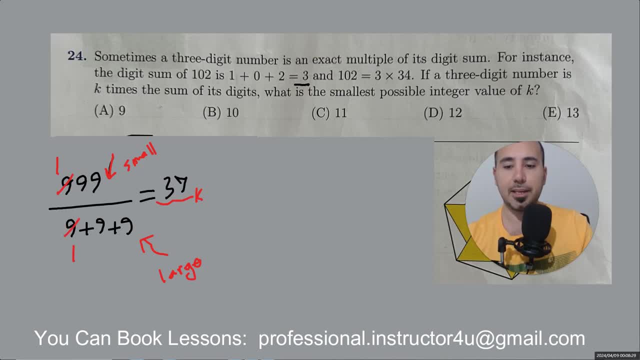 digit. I'm gonna change the hundreds digit, right? if I turn the hundred digit into a one, right? so what happens? it's gonna be right. so what happens? it's gonna be right. so what happens? it's gonna be. what is 199 divided by 1 plus 9 plus 9? it's. 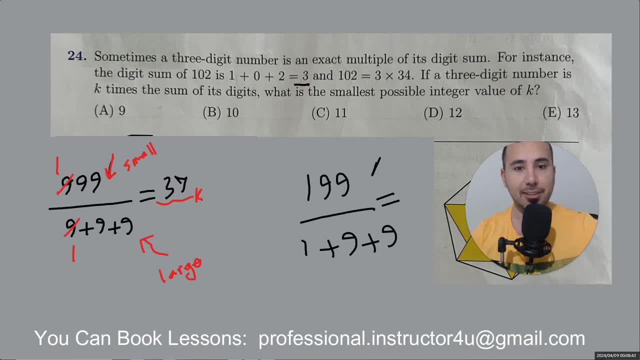 what is 199 divided by 1 plus 9 plus 9. it's what is 199 divided by 1 plus 9 plus 9. it's around 10, 11, 12. see now we got the around 10, 11, 12. see now we got the. 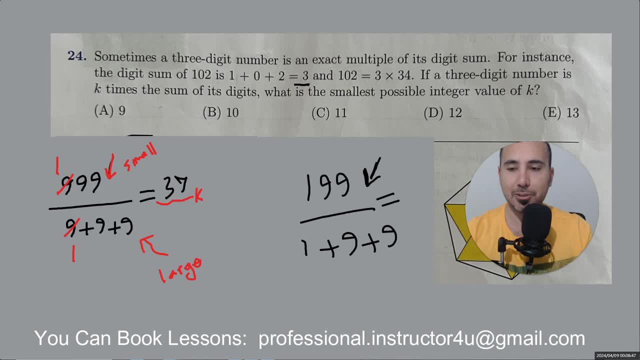 around 10, 11, 12. see now we got the question. we're very, very close. so maybe question: we're very, very close, so maybe question: we're very, very close, so maybe you just play around with this number, you just play around with this number, you just play around with this number, or a more systematic way would be something. 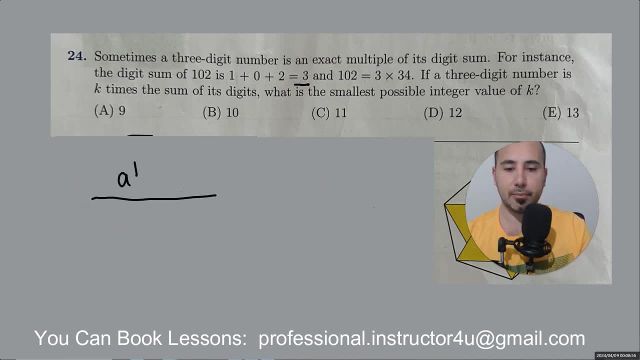 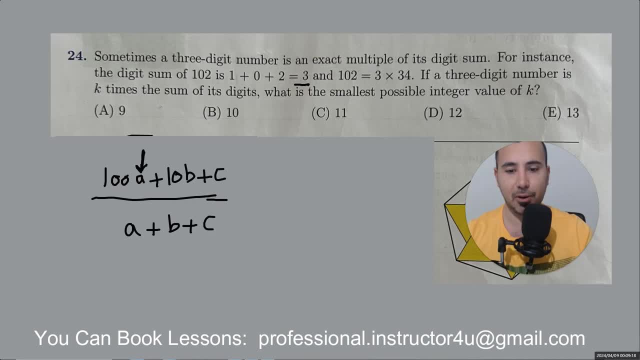 smaller. we want the a value to be really small. okay, because this one is being multiplied by 100, but here it's just one itself, right? so we just want to make it as a small as possible. so I change both of these values by 1. now we have two. 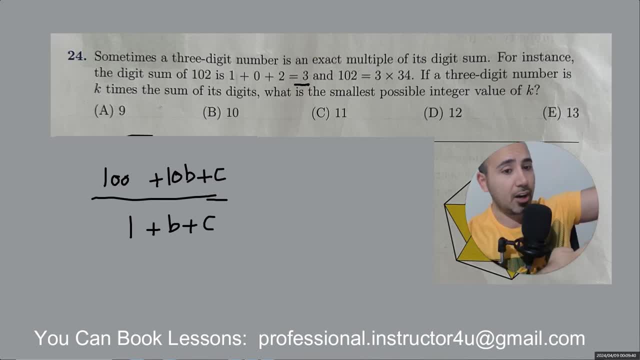 choices would be: should we go with B really large or really small? let's try. so if B is 1, the fraction turns into 100 plus 10 plus C. if B is 1, this is going to be 1 plus 1 plus C, and focus on this part. now what? 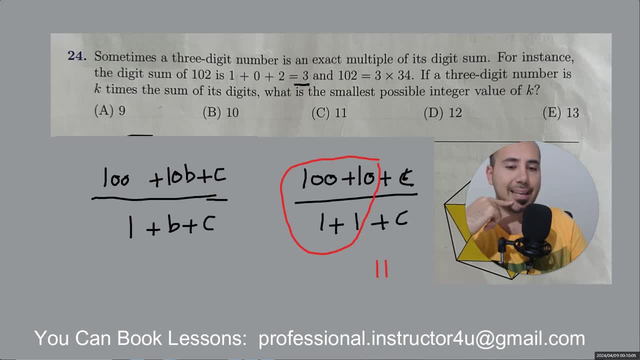 is the ratio of this part 110 over 2. this is 55 really large within one that. so instead we should do the other thing, which is let's make this 9, and if we try with something really large, let's see what happens to the ratio. 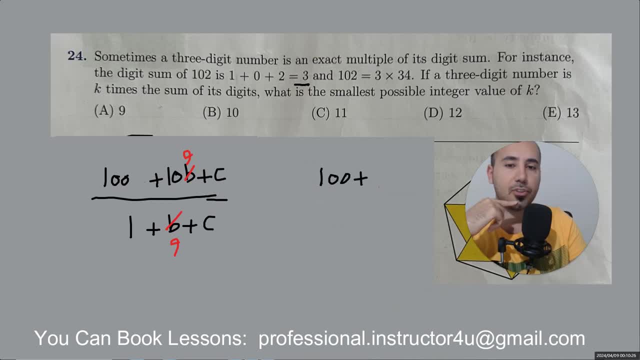 it's going to be 100 plus 10 times non plus C. okay, and this number here is going to be 1 plus 9 plus C. okay, again, we're not focusing on C part now, we're just focusing on this part. this is 190 over 10. 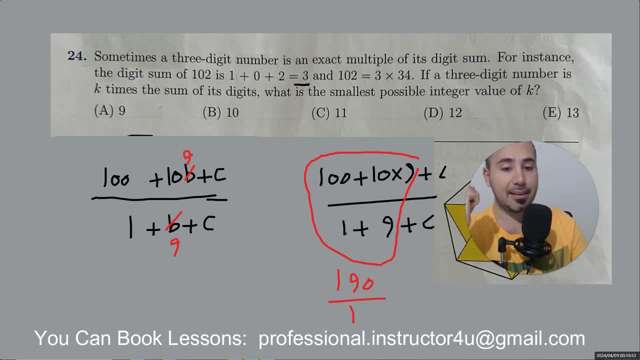 so it's a lot better than 55. but see, now the ratio became 19 from 55. that means B has to be really, really large. okay, so we have the value of B. so here I'm going to make this: if B is 9, this will be 90 and this is 9, okay, so we're gonna have something like this: 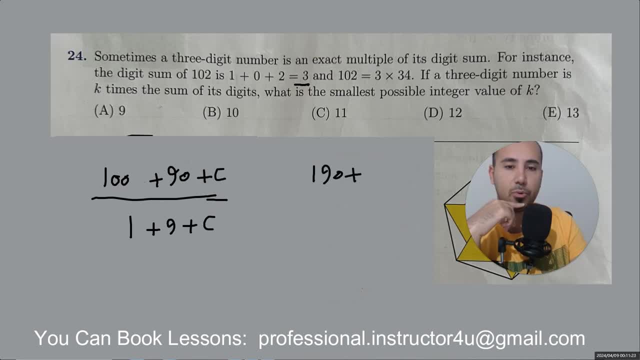 190 plus C over 10 plus C again. should we go see very small a real? if we go with very small, 101 over 11, not really good. but even if C is 9, it's going to be. if C is nine, the ratio will become 199 over 19. there is a problem here, that is, this is: 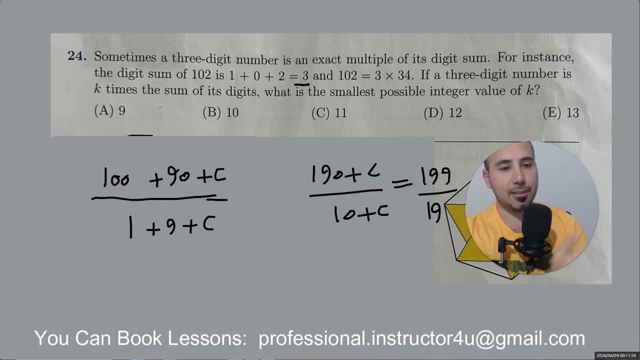 not. actually it's not divisible. so what we're gonna do? if nine is not good, then we're gonna try something smaller. so how about, this being eight, and this being eight, it's gonna be a hundred ninety eight divided by eighteen. now, when we simplify this, both of them by nine, let's go, or both of them first by two is going. 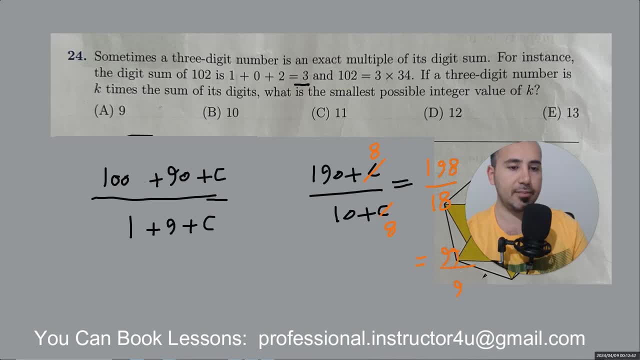 to be nine. this will be 99. if we simplify them, it's going to be 11. okay, that's very good, okay. one thing we need to check though here: when we have 189, if we switch these two right, maybe we could make the ratio even the smaller. so, for example, if I 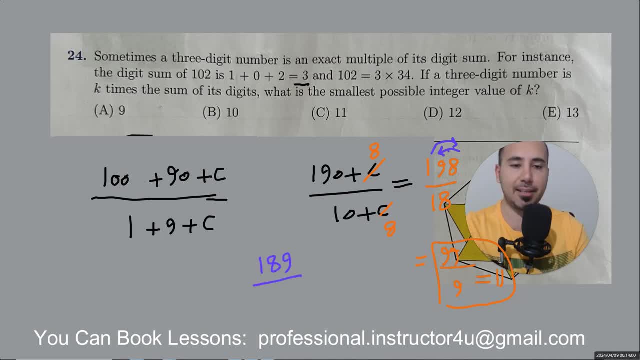 have 189 divided by 1 plus 8 by 9. okay, 189 is a smaller, but it's going to be 189 divided by 18. the problem here is that this one is not divisible because the numerator, the top number, is odd. this is: 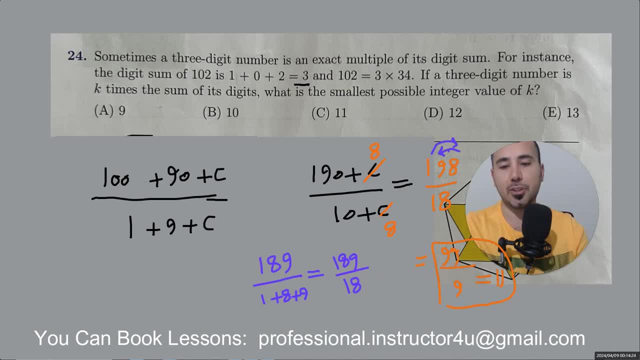 even not going to be simplified, so we have to go with this value. so it's going to be 109 over 18 and the essay would be 11, okay. so anyway, if you write it systematic like this or just try different values, okay, you just have to play around with this and you'll. 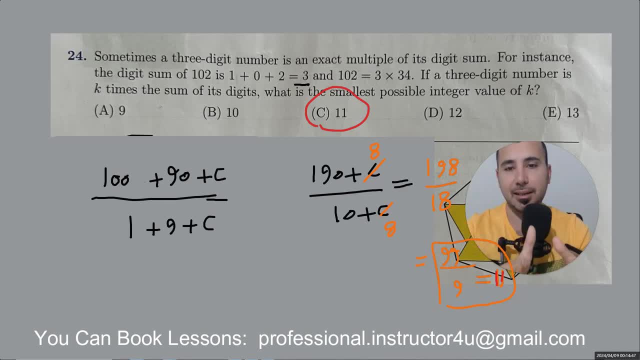 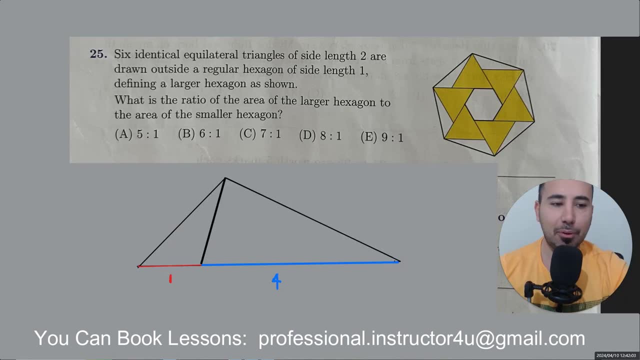 be working around with different numbers to make this really, really, really small. okay, so for problem 25, there is a very simple way of dealing with this question, but to fully understand it, this is the fundamental that you need to know, and I want to check with you if you know it or not. so how many triangles do you see here? three, right. so what is the? 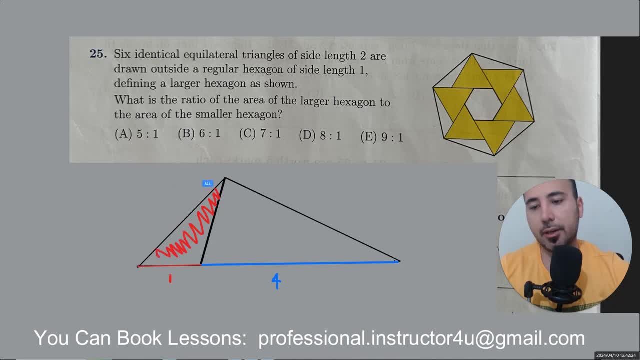 ratio of this red triangle to this blue triangle, the ratio of the areas of the blue triangle and red triangle is the same as 4 to 1. okay, so, for example, if the red area, if you assign a letter to it, for example, if this area of this is a, the blue one will. 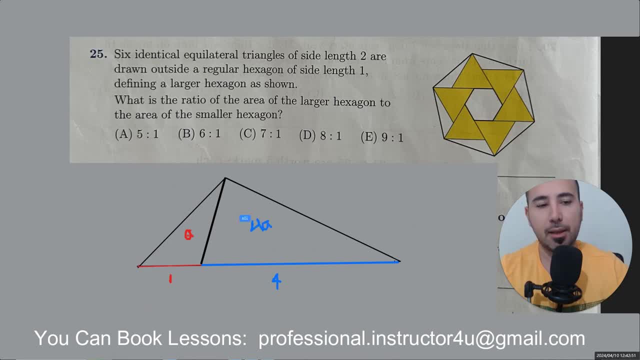 be also 4 times more. okay, and it has a very simple proof. okay, and the proof is very simple. I'm just gonna mention it in case you're curious now. so both of these triangles- for this one and the blue one- both of them will have the same height. 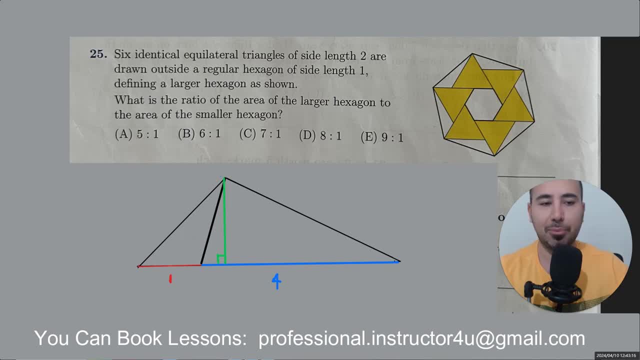 okay, this is the same height for both of these blue triangle and the red triangle triangle, but so they have different bases. if the ratio of the basis is 4, so the ratio of areas is 4. I don't want to go through it any more than this, okay. 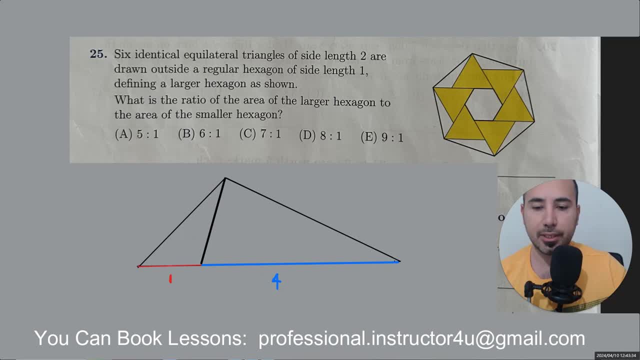 and how is that helpful? because if we see closely here that, for example, now the question tells us if this is 1, the question is giving us that and the question is also telling us this is 2. so in this triangle- let me highlight it: okay, if the red one is 1 and the blue one is 2, right, what is the ratio of the? 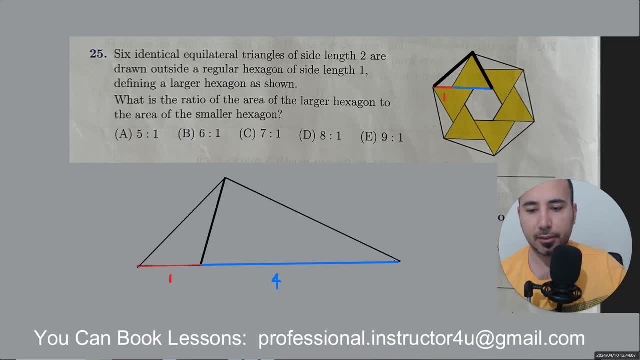 areas. let me go right in here. so the blue one is 2. then what is the ratio of the area of these two triangles here? ok, the one that is red and the one that is blue. so here this one is actually yellow. here the yellow triangle, here the area of it is two times of this area of the little one. 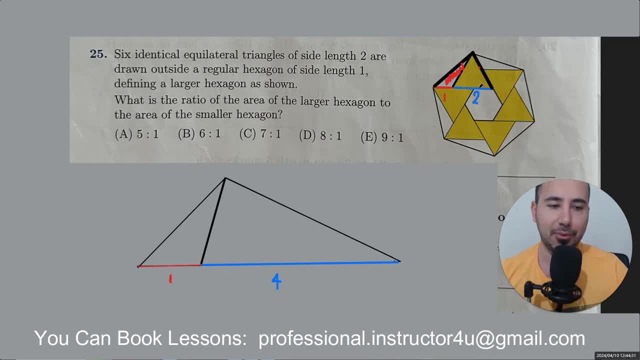 because the bases are two to one, and that's the only thing you need to know. and let me explain why that is. I'm gonna make the question really simple that you wouldn't believe. now let's read the problem. there's six identical equilateral triangles of side lengths- two, okay- are drawn outside the regular. 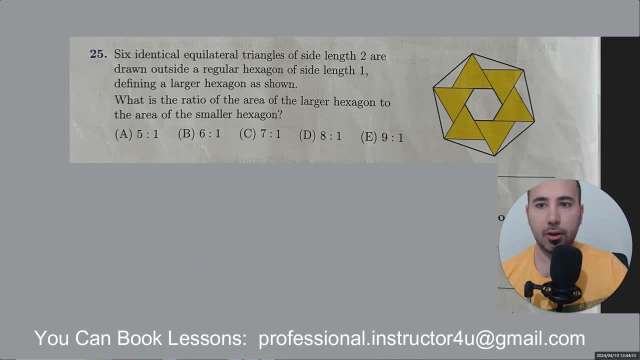 hexagon of side links one. okay, defining a larger hexagon as shown, what is the ratio of the area of the larger hexagon to the area of the smaller hexagon? so I've used this technique for other questions in previous years. right, and they keep you like using this idea. so we know that each hexagon is made of. 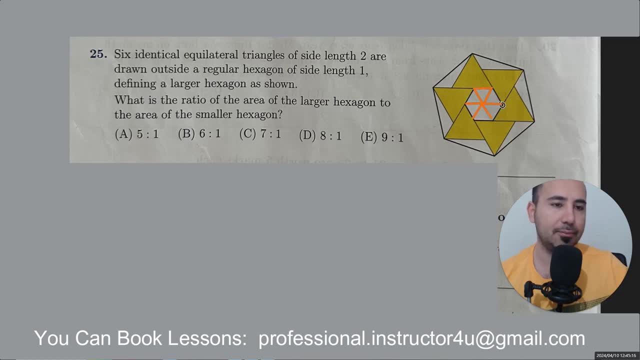 hexagons, and then the smallest hexagon is made of hexagons. so what is the ratio? six smaller equilateral triangles, okay, and each of these- uh, yellow triangles are made of four of these, and that's all that you need to know. so, for example, if the area of one of these triangles 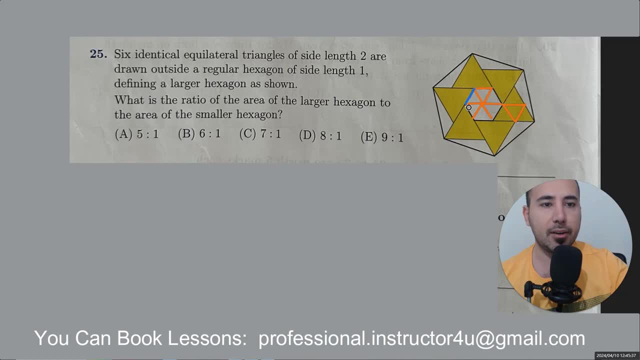 let me see here, let me highlight it by blue: if the area of one of them is a, okay, what is the area of the small hexagon over here? it's gonna be six, eight, right. so what is the area of one of these triangles? this one is 4a, right, and i just said at the beginning that if that is one, 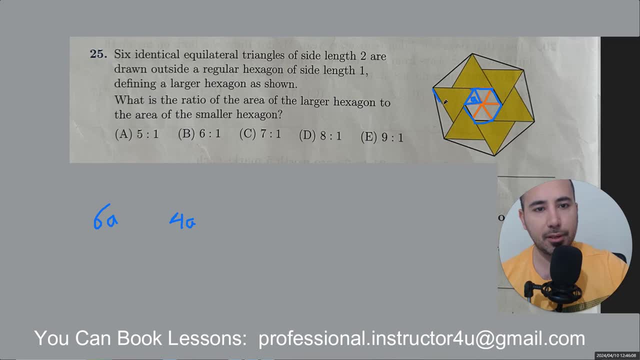 of them is 4a. what is the area of this part? we just talked about that, about it, that the yellow area, if this is 4a, it's two times of the small one, it's 2a. So that finishes the question, right? So what does the question want? Okay, the question wants the ratio. 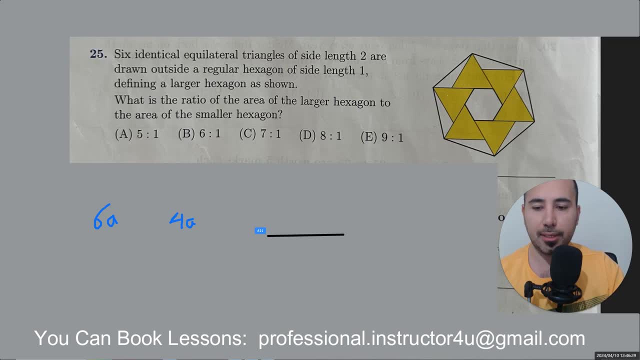 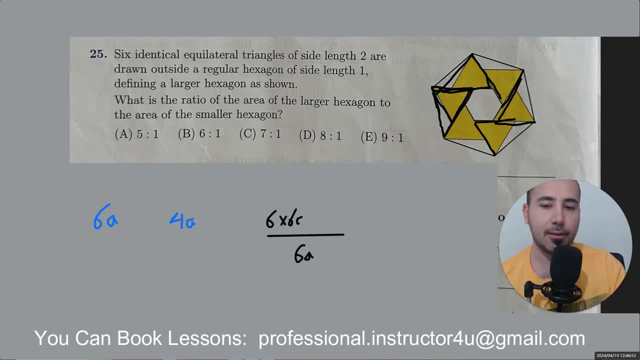 are actually six of these 6a's. Okay, but we're finding the area of the big okay hexagon That includes this part too, right? Right, this is again another 6a. So that's it. So the top one is 42a numerator, This one is 6a, So the ratio is actually 1 to 7.. And there you go. 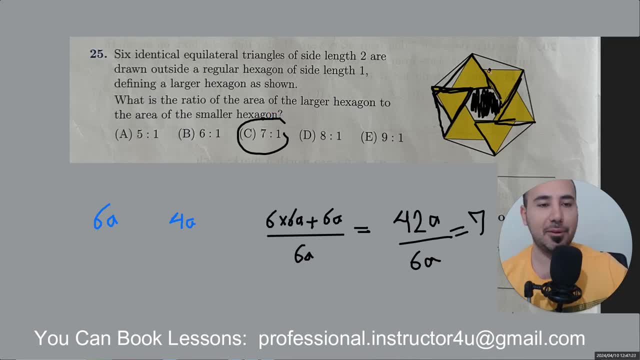 It was so simple, right? Not very difficult. Okay so, and this technique, especially for AMC, Australian AMC. they use it all the time, They love this. So turn equilaterals and hexagons, just divide them into. 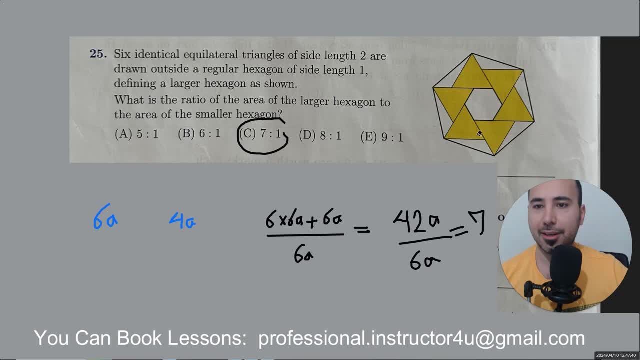 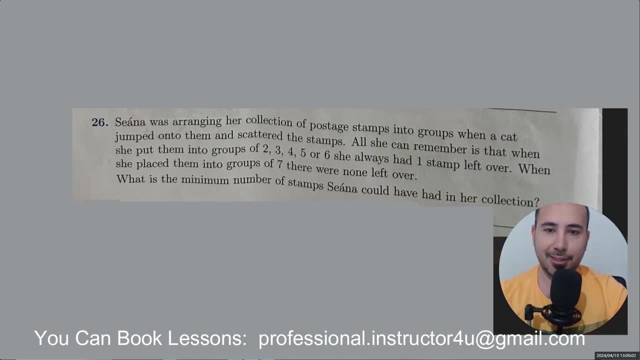 smaller equilateral triangles, and that will solve the question for you. Okay, sorry, if the question looks a little weird, It's because I don't have the PDF version of the questions. Just one of my students took a picture of the test and sent it to me, So that's. 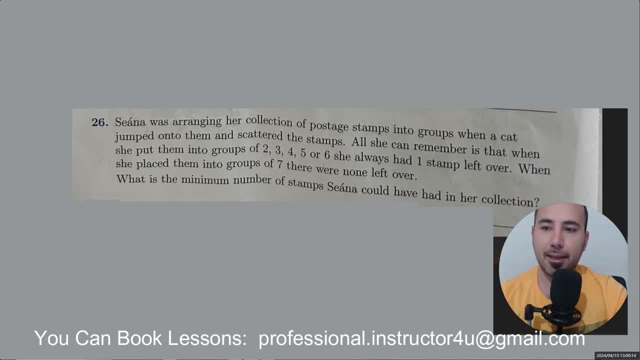 the best thing I have. Sorry for that And personally about this question. I think it's not really that difficult. You can all answer a problem like this, So let's just read it first and then let's do it together, Okay. 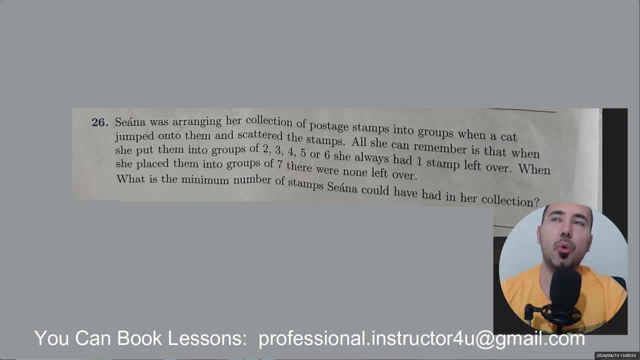 collection. okay, so imagine you know nothing about this type of questions. right, you read it. you don't know. so what is the first step you take? okay, the first step is you don't try to answer this problem. you try to try to answer a simpler, similar problem first. okay, so, for example, now imagine these are not 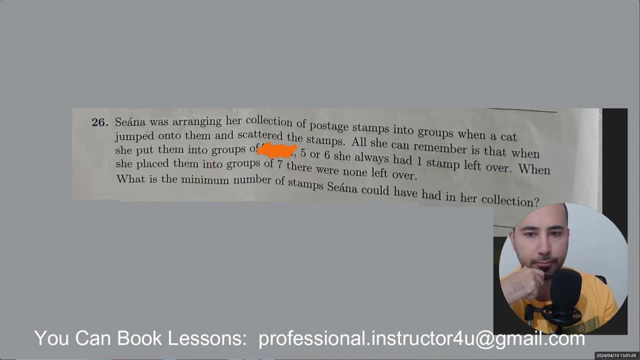 part of the question. okay, so we want a number that when we divide it, okay, when we we want a number that when we put them in group of five, it has one remainder. when we put them in group of six, it has remainder one. what is that number? so what you can do for this one? 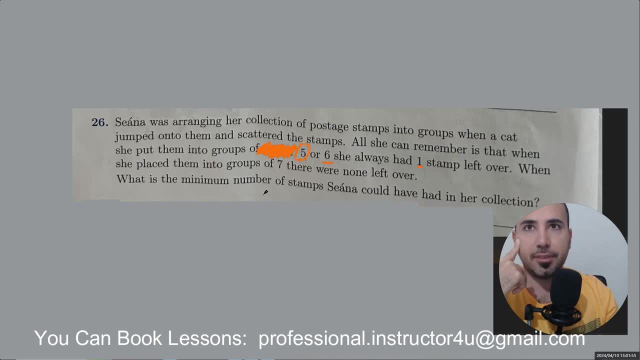 you say: okay, when I put them in group of five, there's one remainder. what is the first number that is like that? it's six. we want the number when we divide it by five. the remainder is one. the next number is 11. the next number is 16. the 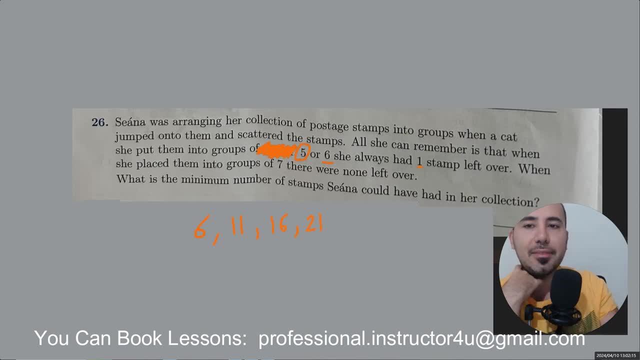 next number is 21, 21. you take any of these numbers and you divided by five. so, for example, I'm going to take 16, one would divided by five, that's 350. you have the remainder is 1. okay, but how did I make that number? how do I make these numbers? I say okay. 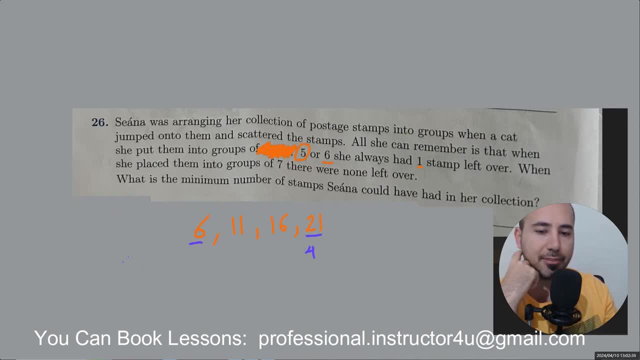 so, for example, this is 4 times 5 plus 1. okay, this is okay. four times four plus a 1. you see now how they are actually being made. okay, sorry, this is not. this is 3 times 5 plus 1. I made a mistake. this is 3 times 5 plus 1. this is 2 times. 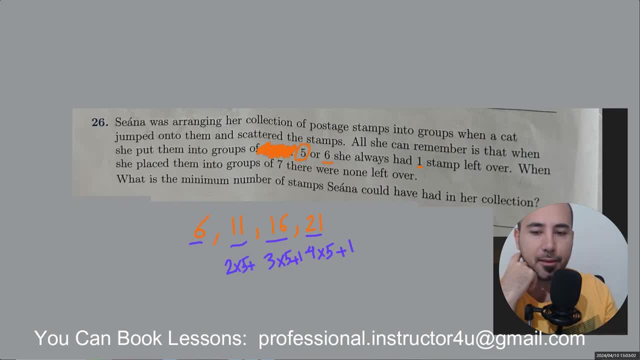 5 plus 1. yeah, you see that. okay. so what is the next group of numbers? you tell me the numbers that when we divide them by 6, the remainder is 1. what is the smallest number? like that? it's 7. what is the next number? 2 times 6 plus 1: 13. 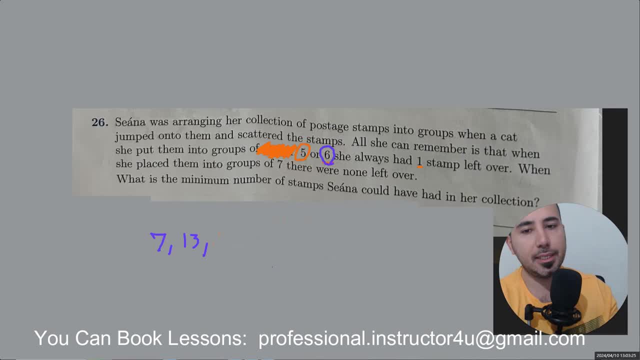 what is the next number? 3 times 6, 18 plus 1, 19. see now. ok, the numbers will continue like this. now we want a number that, when we divide them by both, ok, the remainder is 1. ok, so it's very simple. what? 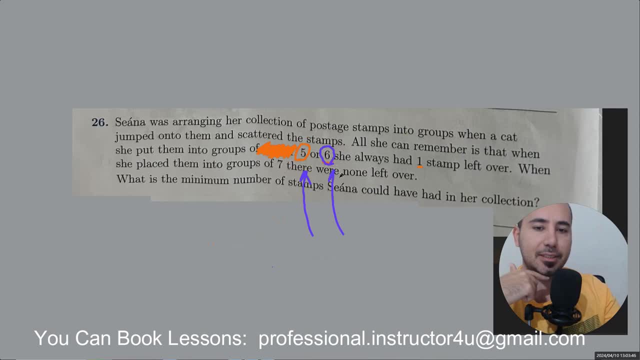 the number that, when we divide them by five and six, it's divisible by both of them, is five times six, and we want the number to be one more remainder of one. there you go. so the number we're looking for is 31 when we go, if i divide 31 by 5, the remainder will be 1.. when i divide 31 by 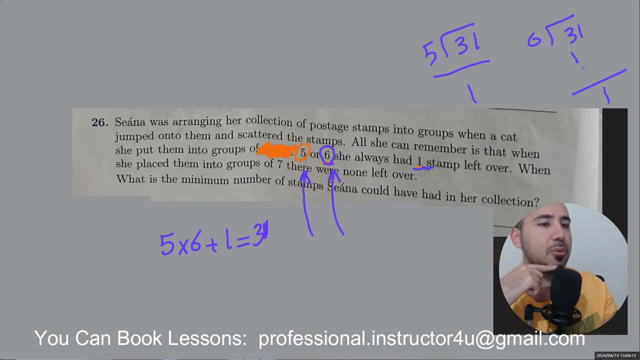 6. okay, blah, blah, blah blah, the remainder will be 1.. what is the next number? that is like that: that when i, divided by 5 and divided by 6, the remainder is 1.. okay, it's very simple, you'll go. okay, 5 times 6 times 2, because we want the next number plus 1.. that's going to be 61.. 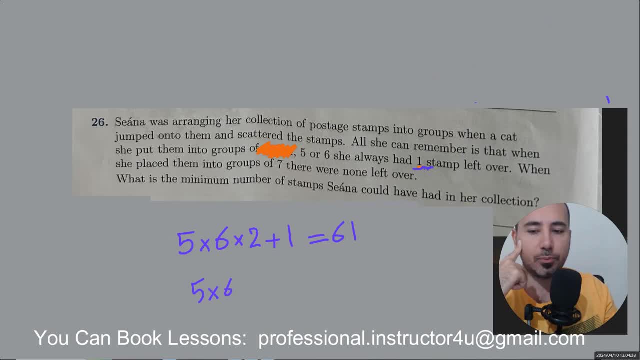 what is the next number? 5 times 6 times 3 plus 1.. that's going to be 91.. okay, so you need to have this like foundation, right? you have to have this experience of playing with these numbers. i know this, okay, if you don't know, you will. 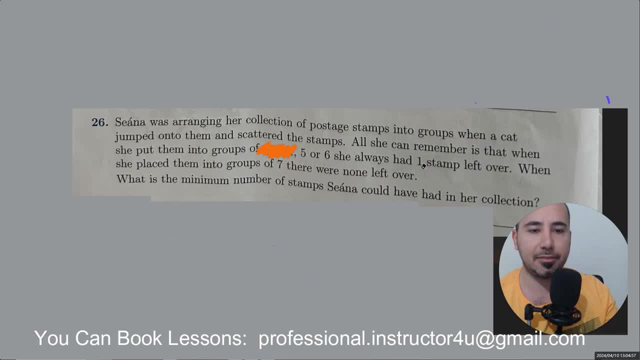 start with simpler numbers and then you build that for yourself. now we want a number, okay, that is divisible by all of them. okay, but when we divide them by the rest of these numbers, you will find that the one remaining number is 1.. so we just need to add that one without any hásti. again, the number remaining number is one. so 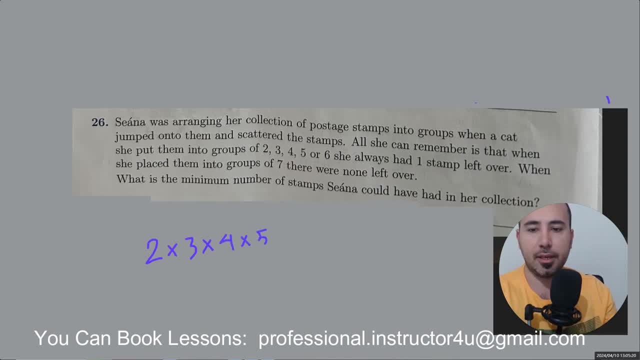 all we have to do to find that number is just multiply all of these together 4 times 5 times 6, and then plus it by 1.. so, uh, 4 times 5 is going to be 20, 20 times 6 is 120. 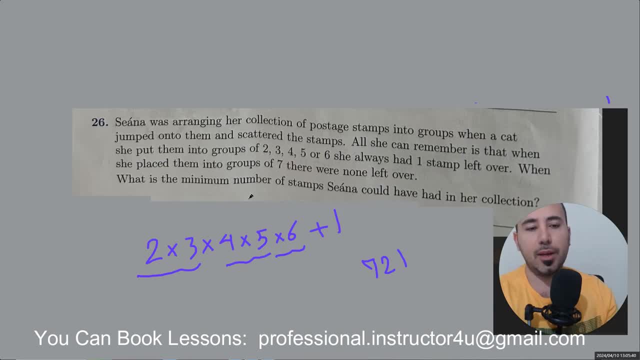 721. we want this number to be also here. it says when we she placed them into groups of seven: okay, there was none left over. so if i divide it by that number, okay, it's going to be 103 here and the remainder will actually be zero. is that going to be the answer? should i go? oh, i found one. 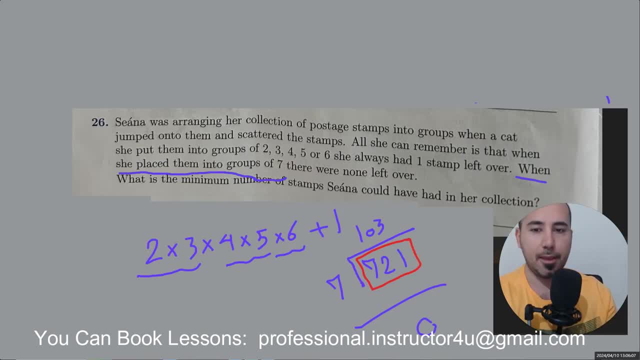 721. good, there is one thing here. it says what is the minimum number of the stamps? what if there is a smaller number that just have has all these conditions? okay, so to find the smaller number. okay, not this one, we'll do something else. you see, when we multiply all these, 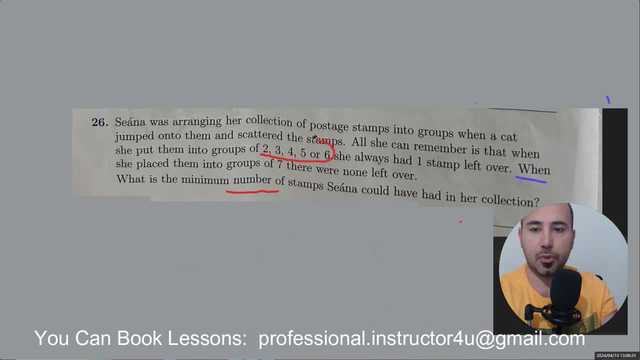 numbers. okay, we just want to find, okay, the least common multiple of these numbers. so to do that, for example, like, look at this: this one, six is a two times three. okay, if a number, so that means we don't really need this one. so there's a two, that's a three, this is a two times two, okay, 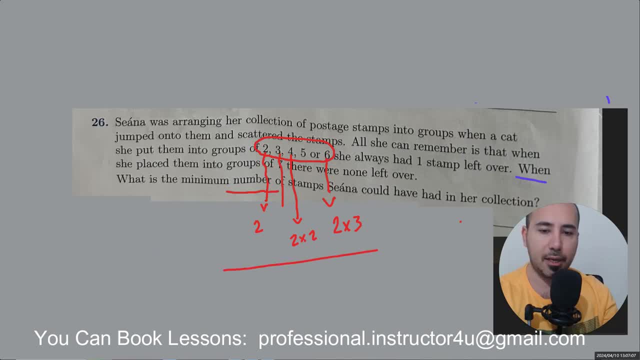 okay, okay. So we just want the least common multiple of these numbers. so what is that? we want the number first to be divisible by 6, so i'm going to write 6.. We want it to be divisible by five? okay. we want it to be divisible by 4, but it's already divisible by 2, right, because there is? 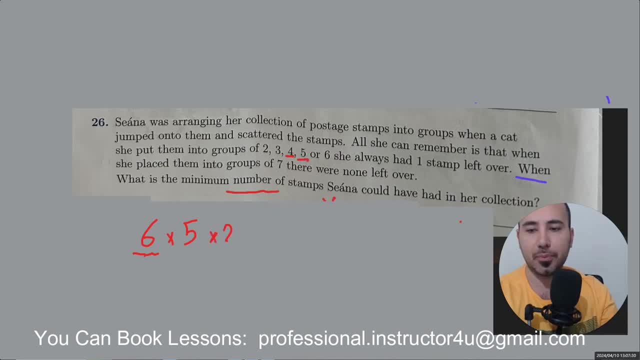 a 2 in 6, two times 6. so i'm just gonna multiply it by two, and if a number is divisible by six, we have six here. no need for this, no need for this. so the least common multiple is going to be 60.. 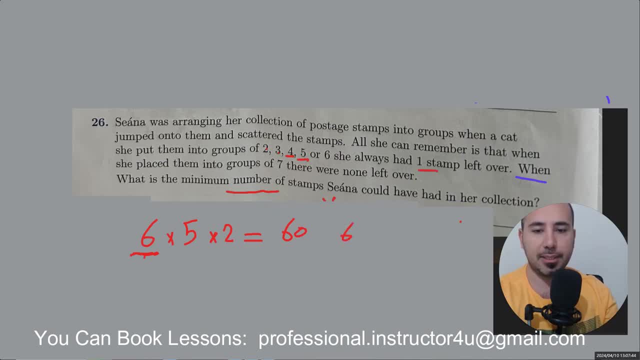 so then i have to add one to it. it's going to be 61. so you try that. so 61. when you divide it by any of these numbers- two, three, four, five, six- the remainder will be one. this is the smallest one. okay, 31 will not do that for you. okay, because 31. 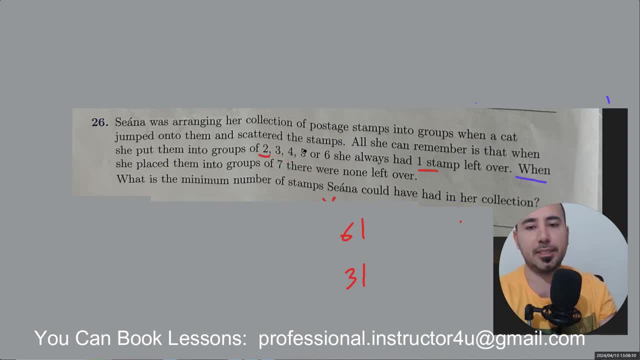 is not going to be not for four. okay, because 30 is not divisible by four. so anyway, now what is the next number? uh, the next number. the numbers are going to be like this: 61, 60 times 2, 121, and the next one 60 times 3 plus 1. 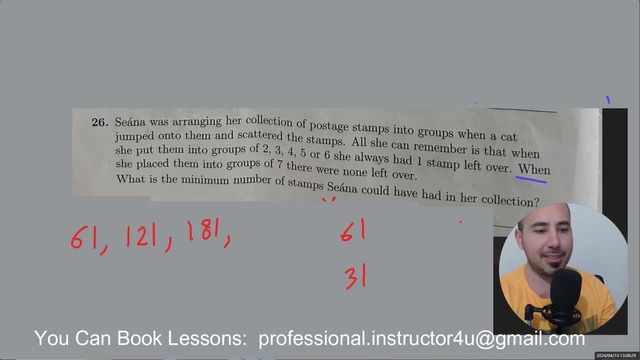 81 and the next one. you see where i'm going with this. the next one will be 241. so we want a number one of these that is divisible by seven, also because when we divided by seven, there was no remainder. so let's go here, the next number. 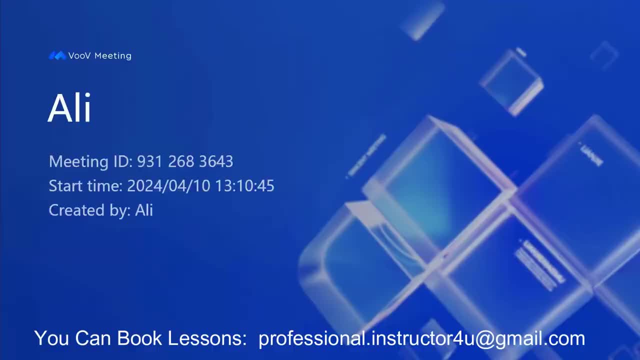 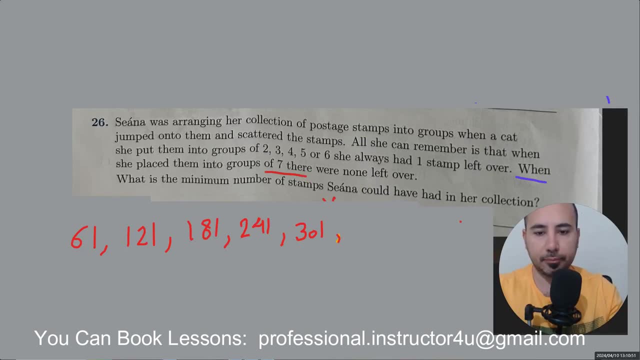 is going to be uh, 301. okay, so now i could continue writing the next one like. the next one will be 300, 61. the next one is okay, 60 times seven plus one um 421. but what is the smallest of these numbers that is divisible by seven? is this divisible by seven? no, 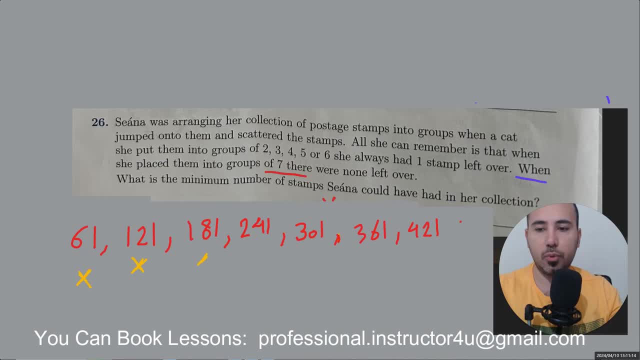 this one, uh, no, how about this one? 181 divided minus 140, it's going to be 41- is not divisible. so if you don't know how to do this, maybe you just go and just divide them by seven quickly see if there is a remainder here. so, however, you know so, and then 241. 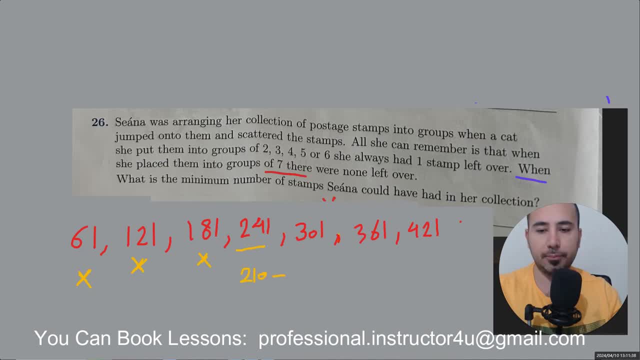 this is going to be 210 plus 31. okay, so this is how i do it. this one is divisible by seven, so good, but 31 is not, so 241 is not divisible by seven. there are other ways to learn the visibility by seven, but this number 301. 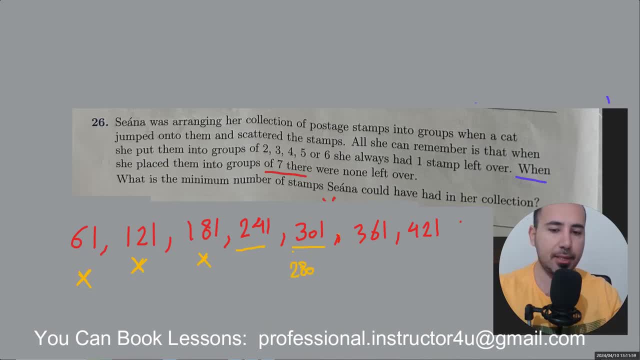 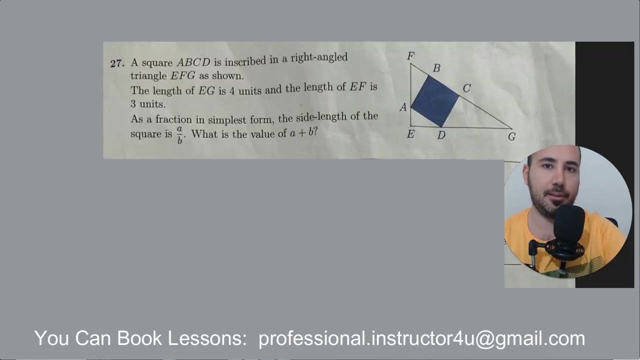 uh 280 is divisible by 7, because that's 7 times 40 plus uh 21. both of these are divisible by seven, right? so then you would go and choose this as the right answer, because this is going to be the smallest, the minimum of all these numbers. okay, so for problem 27, I'm going. 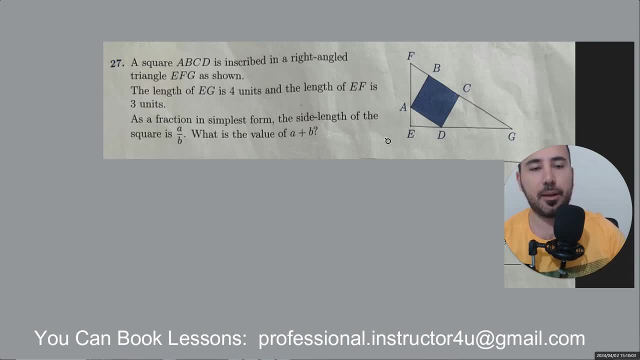 to ask you some questions. in this diagram, how many right triangles do you see? that's one, that's two, that's three and all of it is four right angle triangles. and let me tell you, do you see parallel lines, since the question says that the shaded is a square. okay, so ABCD is a square, then we're going to have 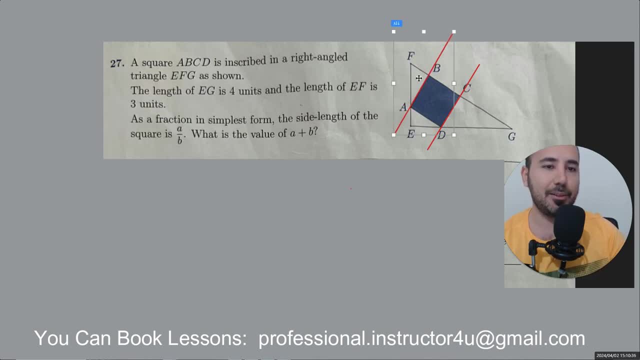 parallel lines. okay, so parallel lines and triangles, they make similar triangles, okay. so for all of these triangles, right, for this one and this one. now, this angle is equal to this angle. this is 90 degrees. this is 90 degrees. so the third angle has to be equal if all the 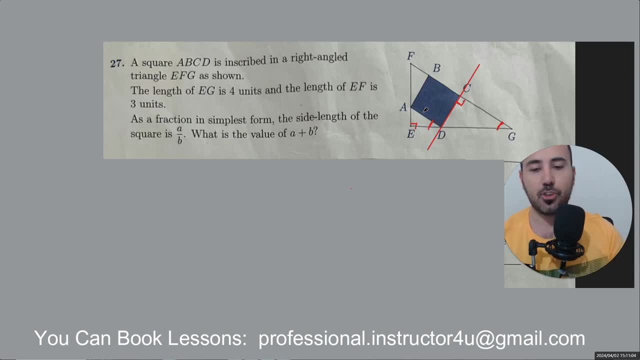 angles are equal, they're going to be similar. so remember this: triangles and parallel lines that come in different types of questions- that the answer in the approach is three Similar triangles. right, I want you to remember. okay, Parallel lines, triangles. then you look for similar triangles. 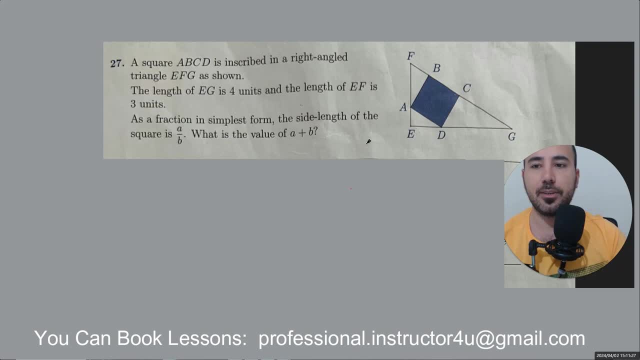 That's your clue. Good, Now here it says: the small one here is 3.. This one is 4.. Then the large one is 5, right, We know that. Good, And what does really the question want? The question wants the side of the square. 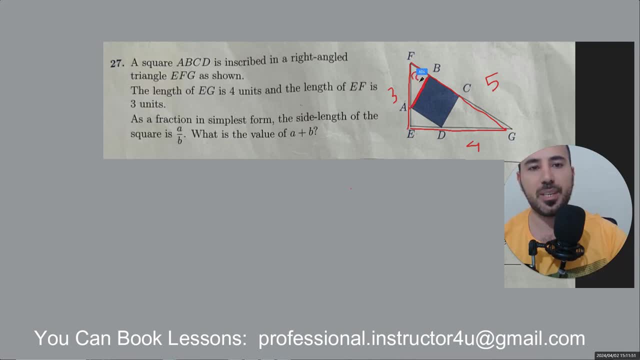 We're looking for this, But it's going to be a fraction, right. And then, for example, if the fraction is going to be 1 over 2, then the answer would be 1 plus 2, right, That's the problem. 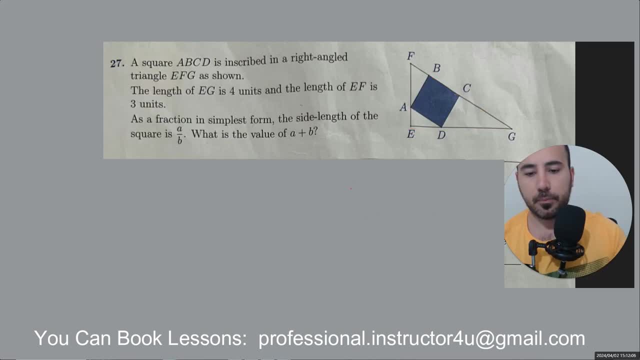 And let's see. okay, Now, when you just choose variable, you might think they're really important how you name them. I think they are very important how you name your variables. okay, So I'm going to call this one red and I'm going to go call this one blue. 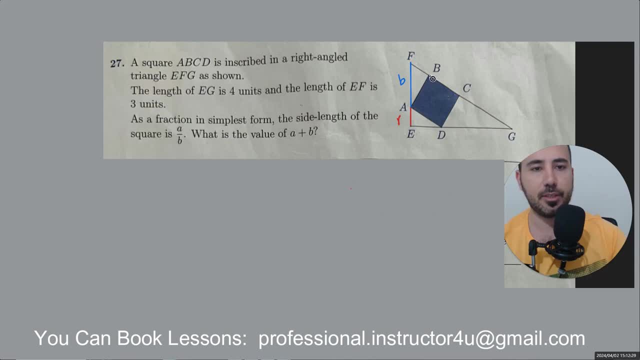 And we just want to find the side of this BC I'm going to call. all of it are equal, So each of these sides. I usually name them A and B, But since A and B are already taken by the question, I'm going to call this one. 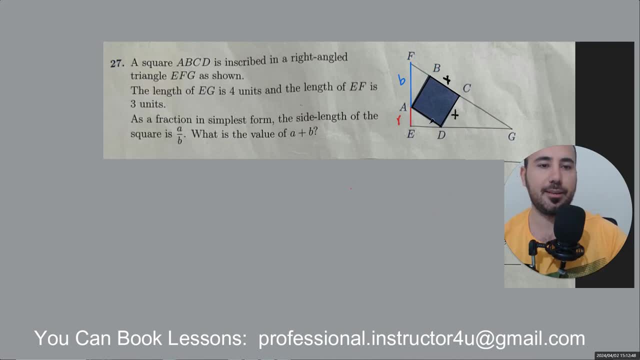 X. Okay, this is also X, This is X and this is X, right, Each one is X. Good, So in the question we already have, red plus blue is equal to 3.. 3 is the smallest side of the triangle, right. 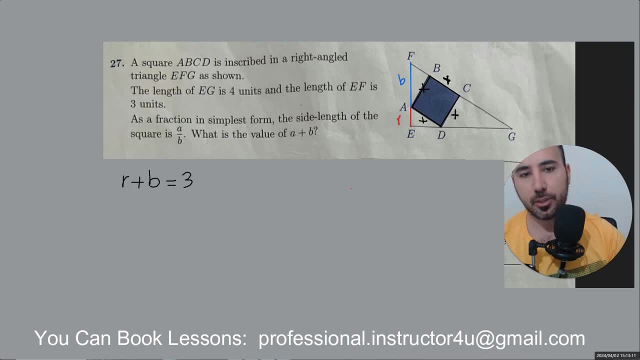 So, and then I'm going to focus on this triangle. Okay, So in this blue triangle X, is it the smallest side, Is it the largest side or is it the middle one? This one is the middle one, right? So I'm going to write it over here. 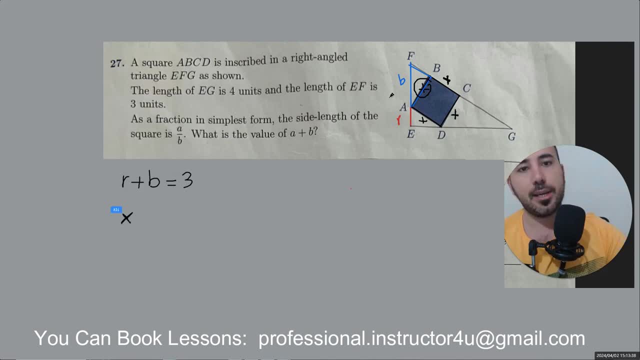 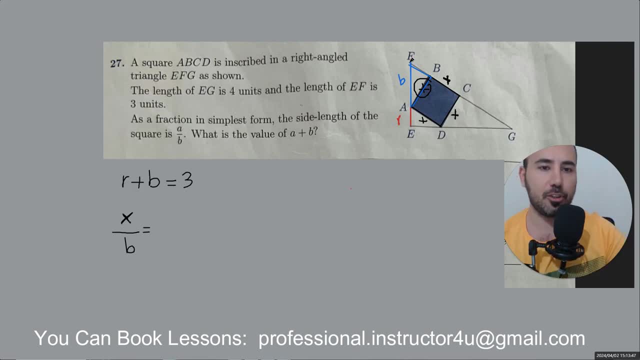 Okay, Okay, Okay, Okay, Okay. Good, Let's say that we have 5 plus 6 plus the lunch. There we go. Good, Okay, Okay, Okay, Ü cradle, the middle side is equal to right. 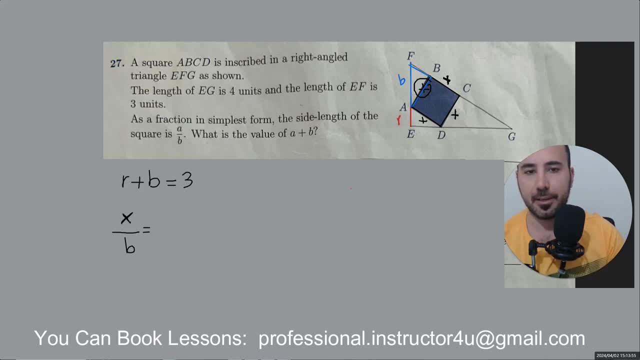 In the main triangle. what was the middle side? The middle side was four, The large side was five is equal to four over five. Okay, So this equals to 4 over 5.. Okay, That's one, And we're going to repeat the same steps for the red triangle, right? 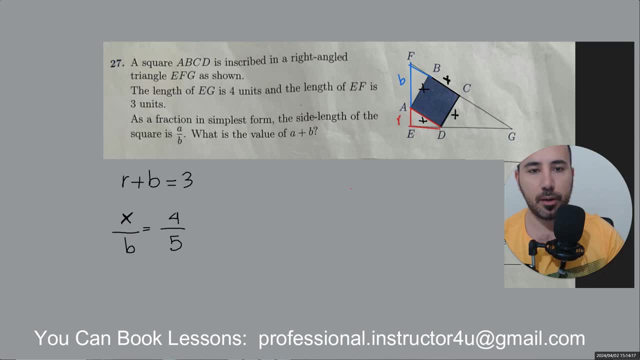 Okay, okay, the red one over x is equal to what red over x. okay, red. this side is the smallest side of the triangle. x in this triangle is the largest side. so in the big triangle the smallest one was 3, the largest one was 5 and the question is solved now. okay, so we have r and b. we want r in terms of. 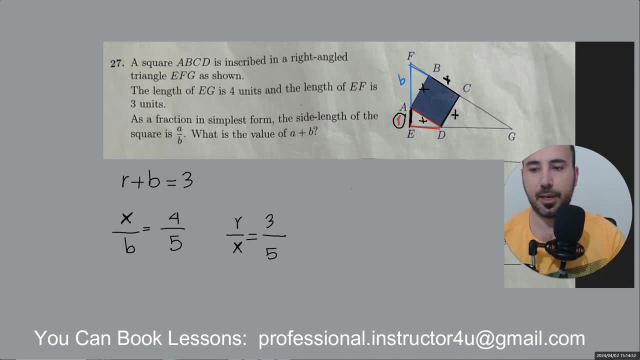 x. we want b in terms of x. what does that mean? let's do that, okay. so from here, um, i'm going to cross, multiply, i'm going to get, for the first one, 5x is equal to 4b, so b is equal to dividing. 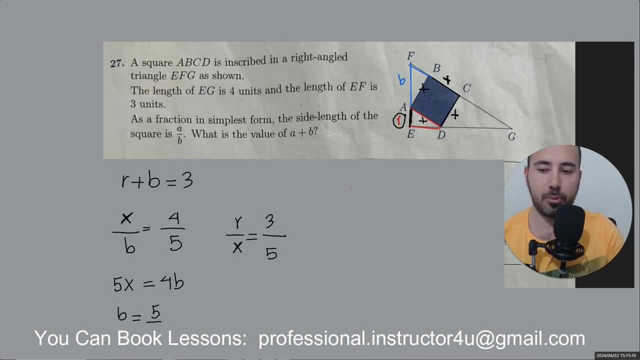 both sides by a 4, 5 over 4x. good, let's do that for the other one. cross multiply 3x is equal to 5r and r is equal to dividing both sides by a 3. r is equal to 3 over 5x. okay, now how do we do this? 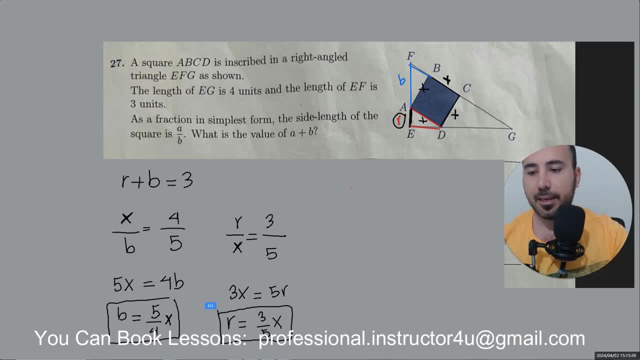 we're going to do a. okay, now, how do we do this? we're going to do a replacement- what's what's not? instead of r, i'm going to write 3 over 5x instead of b. i'm going to write 5 over 4x- replacement, right? so then, if i replace them- and i'm also going to change color- 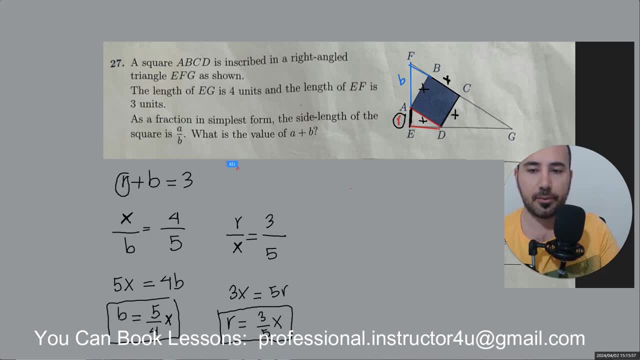 instead of r, i'm going to write 3 over 5x and i'm going to replace b by 5 over 4x, and both and both of these are equal to 3. good, so, since both of them they have x, i could, because it's. 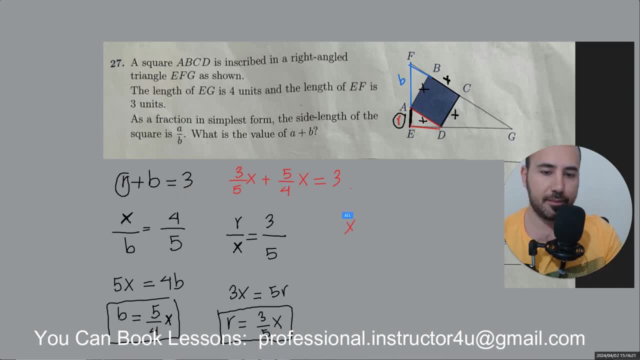 common. i'll factor it. i factor it out. so x will be 3 over 5, plus 5 over 4 is equal to 3. so i just need to add these two fractions together. so x multiplied by what is this? when we add them, it's going to be five times four. i'm going to write it. 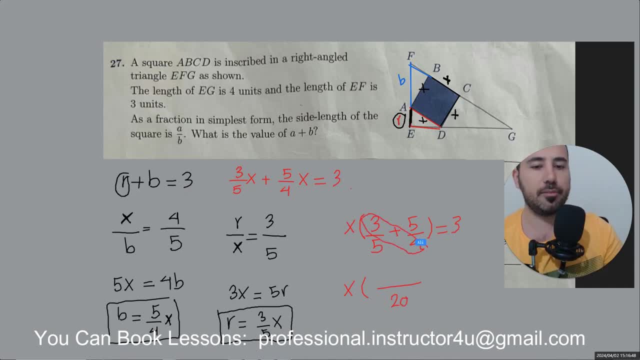 here three times four, twelve five, five times five, twenty five. if i add them together, that gets me 37 is equal to three. so and here, um, let's see. so i'm going to go- x will be- i could multiply both sides by 20 over 37. i hope that confuses nobody. okay, so x will be three times okay. opposite of: 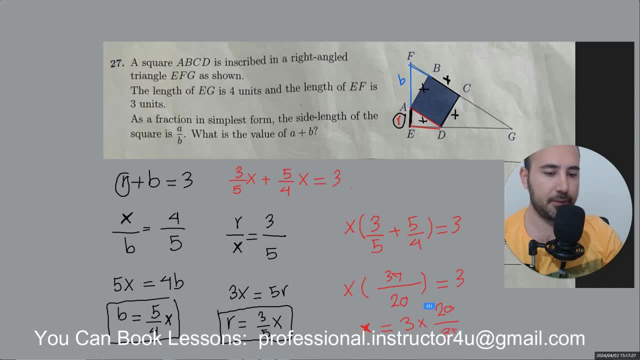 this 20 t over reciprocal of 37. so x will be 60 over 37. that's that. now can we simplify 60 and 37, right? are they both divisible by a number? no, so they are in their simplest form already. so then, what does the question want? it says: if this is a, this is b. 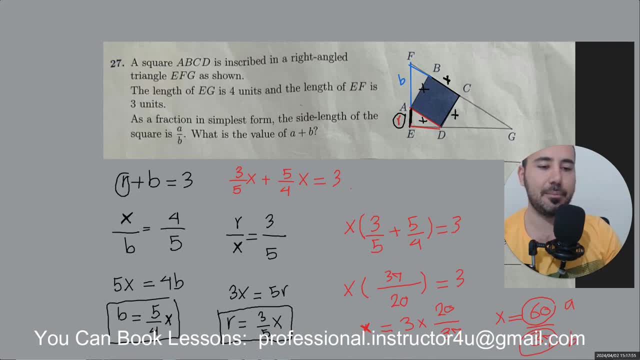 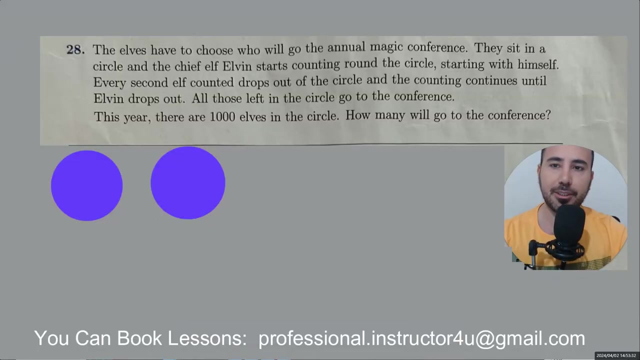 we want a plus b, so add 60 plus 37 and that's going to give us 97, which will be the answer to the problem. if you find these type of questions confusing, i know the reason why. right, the reason is that you don't know where to start. you don't know. 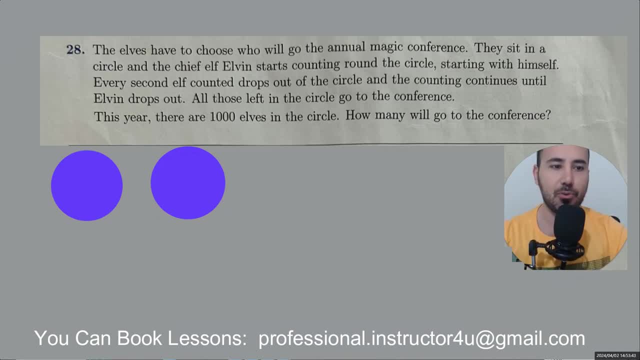 what the first step is. what is the second step is right. so you read it and say i don't know, and then you give up, right? so let's see how we deal with a question like this. it's easier than you think. the elves have to choose who will go to the annual magic conference. they sit in a circle. 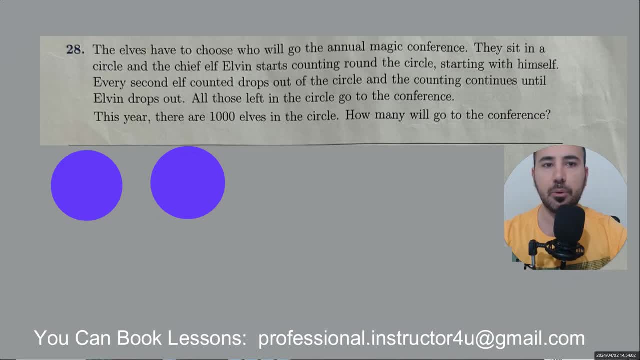 and the chief elf, elven, starts counting around the circle, starting with himself. every second elf counter drops out of the circle and the counter continues until elf elven, the king, drops out. all these left in the circle go to the conference this year. okay, now this is the case. 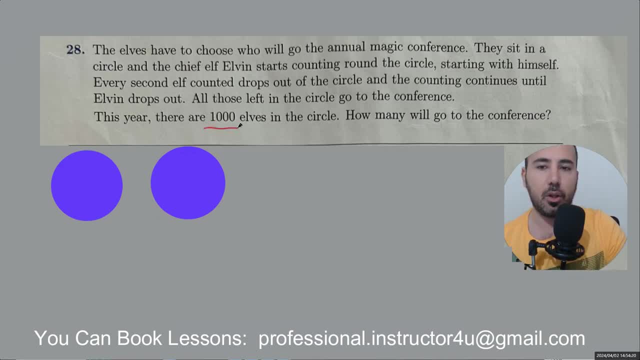 this is important. there are a thousand alts in the circle right, so a lot of people decide to start with a thousand and analyze the thousand, and that's why they can't do the question right. so to understand this problem first, this, the first step, is to do the similar question with an easier. 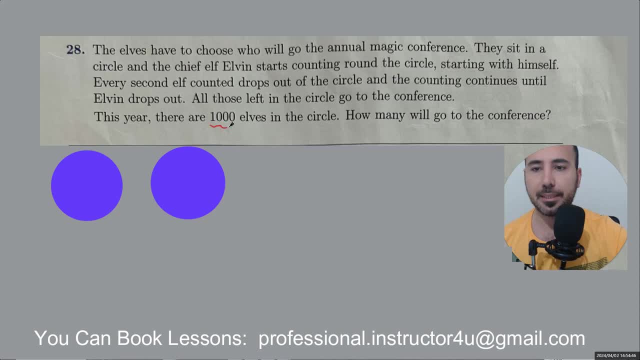 example, right, so basically a thousand. instead of doing the question with thousand, i'm going to go with 10, right, and let's see how it is. so we're going to have only 10 people here and we're going to just decide how we could answer this question with with 10 instead of a thousand, and see how this is. number one is: 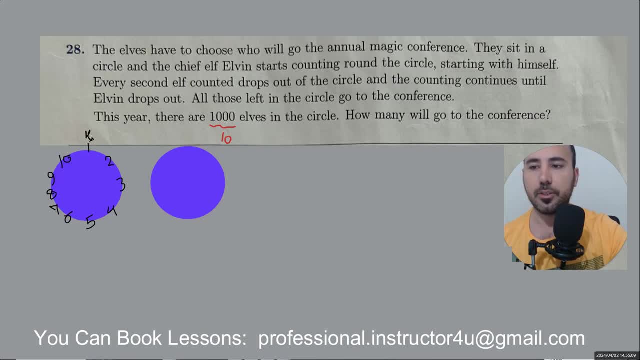 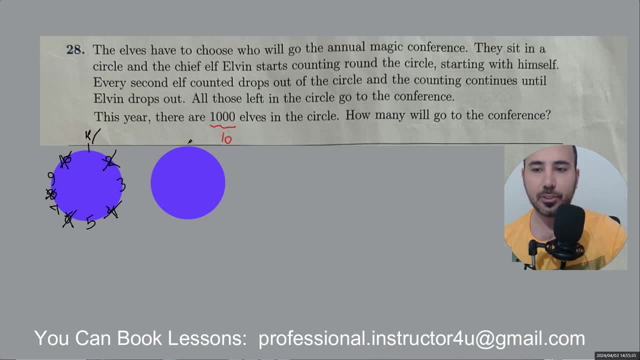 five. i crossed the even numbers, so the numbers that are remaining are one, three, five, seven. and now let's go and repeat the same steps. okay, then king counts himself first. the second one is three, so three will be kicked out. okay, so let's kick him out. three is kicked, then five is day, seven is kicked, and uh-uh. 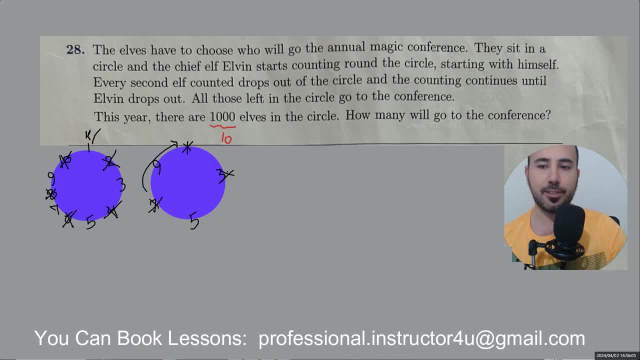 the king was also kicked out. so what are the two numbers remaining? only five and nine. do we really understand what's going on? can we apply this to a thousand? i would say no. so let's come up with the other example. see another example would be maybe an odd number, but i'm going to go this example. 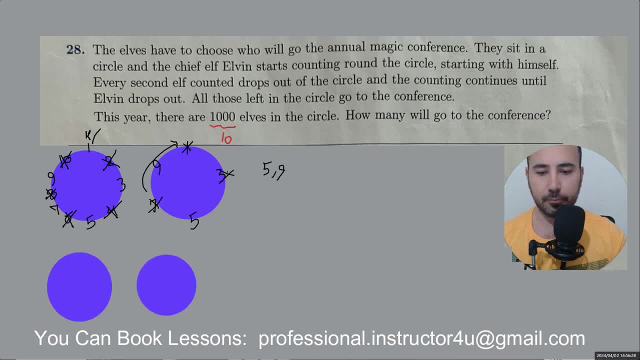 another example with eight instead. okay, so let's see one. maybe i go with a different color, i go with red. so we have one, two, three, four, five, six, seven, eight. you repeat this examples until you get what's going on. okay, so then the king doesn't count himself, counts himself. so ten and me. 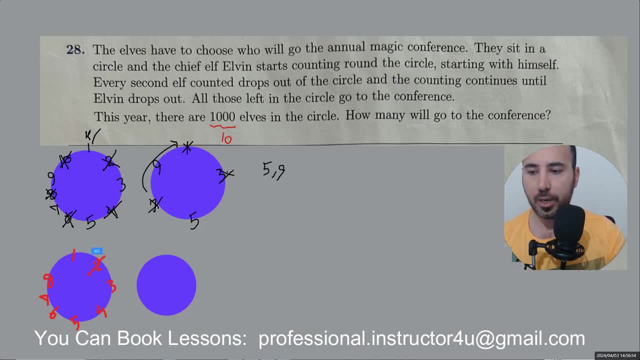 king doesn't count himself, counts himself. so two out, four out, six out, eight out. what numbers remain? one, three, hm, folks can't see slamming in. five and seven remain. and then what happens? see, we have four numbers remaining. this, so that would be two out four, six. and then what happens? 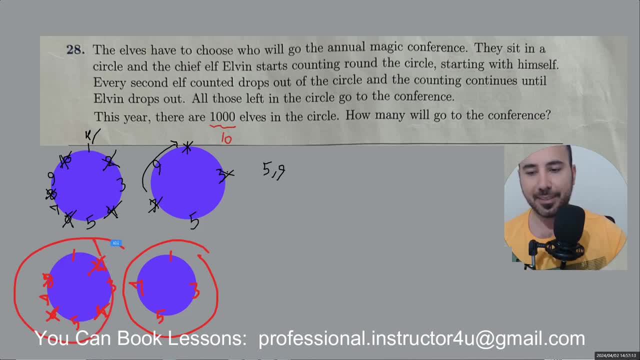 number. eight was even now. four number is even. let's see its behavior. okay, so the count: the king is here, three is out, five stays up, seven is out, so the king stays. it would be like a one and a five: King counts himself and then five is out. 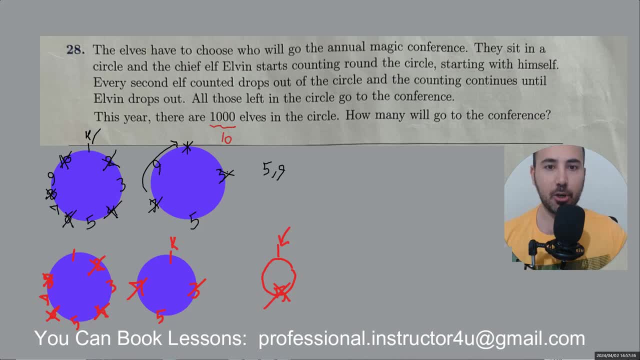 so if the number was eight, nobody goes to the party, right, like no one. but see, we have to understand what's going on here, right? so then another example. let me go with something that is only odd numbers: one, two, three, four, five. okay, so the king is here, the stars eliminating the next one, then the next one, and then 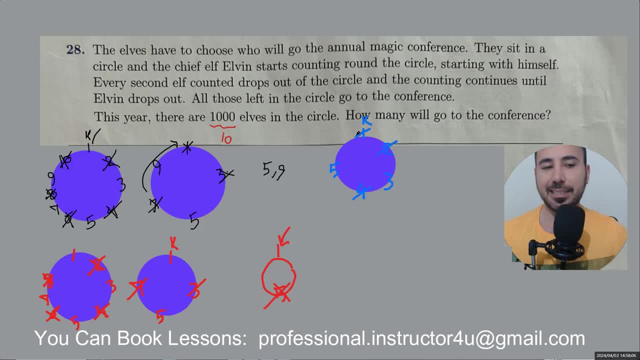 the king will be eliminated. see after these examples: okay, you can come out with what's going on here. if the number is e is odd, like five, at that turn the king will be eliminated. but if we start with an even number, so like this example, it was eight. okay then. 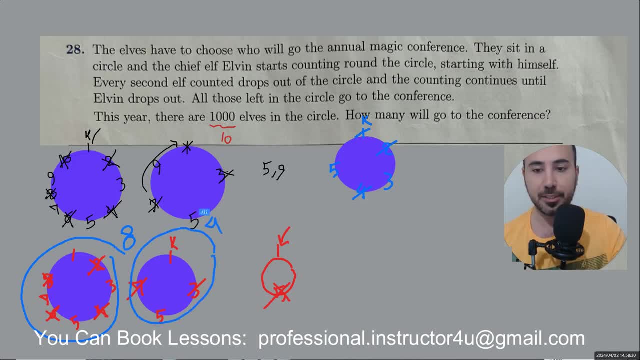 we divided by two became four people is still even, so it continues. two was, though, even right, and then the only one. even the king will be out right, but, for example, the example that we had with ten coming right, the number in this case is the beginning is out. okay, so it's. 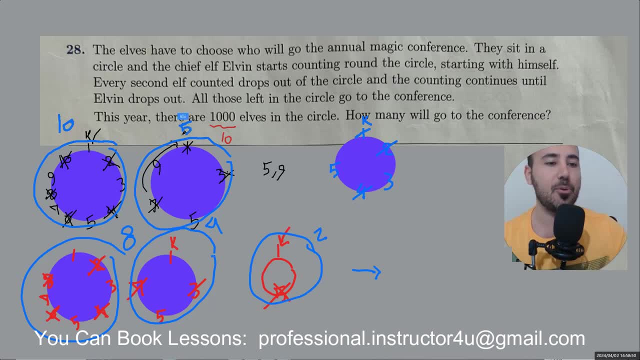 an even number once it became odd five number they can is out. so really, basically, this thousand could have been 2,000, it could have been for you, it doesn't really matter, okay. what we can understand is that each time half of them, that the even numbers are kicked. but when we have five people, how many people are kicked? 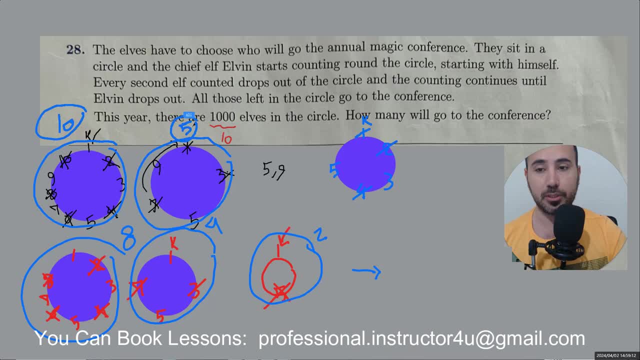 they are이스還د kicked. this is really important. okay, first three is kicked, then seven is kicked, then the king is also kicked out. right, we have to keep this in mind now. okay, all we have to do is just apply the same thing once you understand what's going on in this question. okay, then it's going to be. 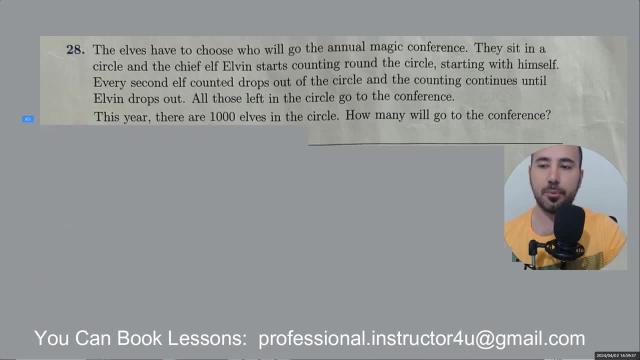 very, very easy. so we have a thousand people. is this odd? or even it's even: is the kick? is the king out? are we going to kick out the king? no, it's just going to be so: half kicked, half a stay again. we're going to do it another round. it's even half kicked, half a stay again. 125. 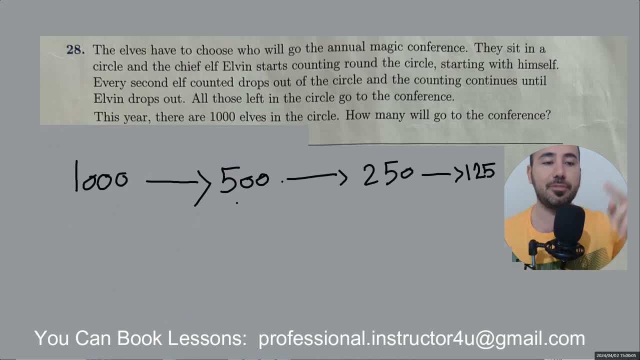 this is now special because for the first time, we have one, two, five, so. and then we're going to kick out all the even numbers. see now, just visualize this: one, two, three, it's going to continue all the way to one, two, five, and we're going to kick out everybody who is even from here. 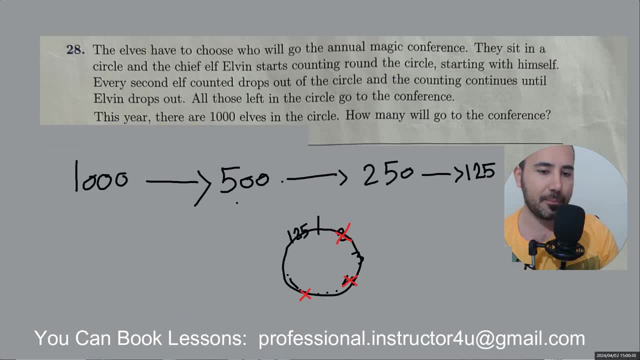 so how many even numbers are? 125 is odd. 125, 124 numbers divided by two. so how many number even numbers do we have? we have 62. we're going to kick all 62 out, okay, so it's going to be 125 minus 62. 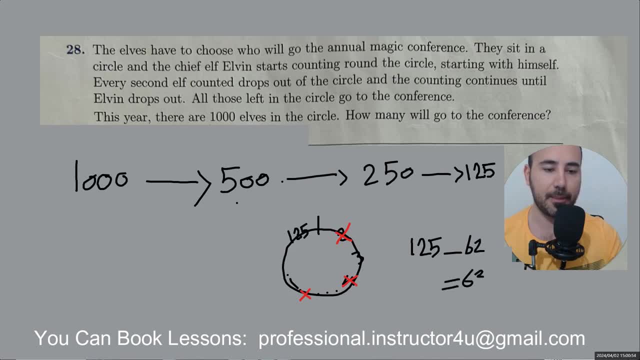 but we have to be careful here. okay, because we have kicked, okay, 62, and once we are here, after we kick 123, 124, sorry, we're kicking even numbers two, four, six. after we kick this. now, once we go back, do we kick out the king or not? am i gonna go 63, all the odd numbers? if we kick out the king, we 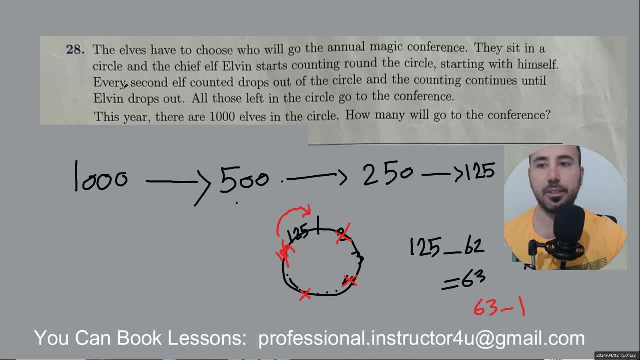 have to minus it by one. let's just see it here. read the question. every second elf counted drops out a circle, and the counting continues until 11 drops out. so we have to kick them out too. so the number is actually 62. so that's the answer. 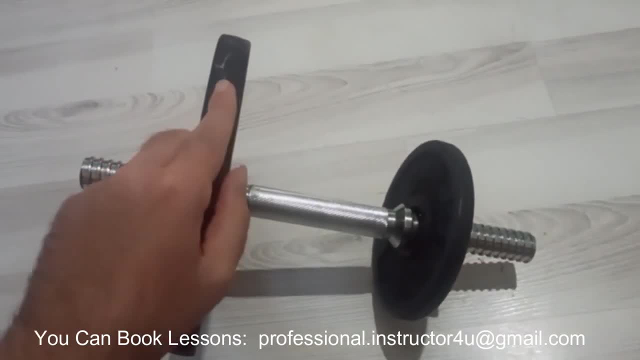 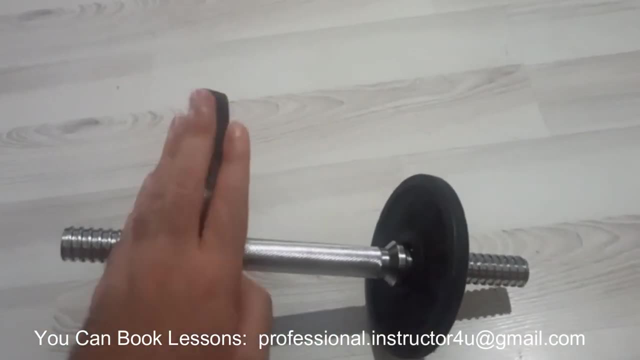 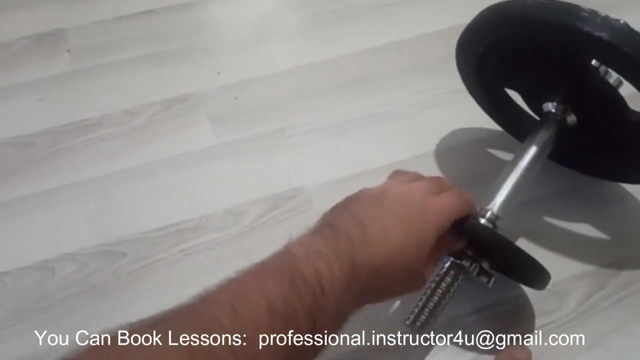 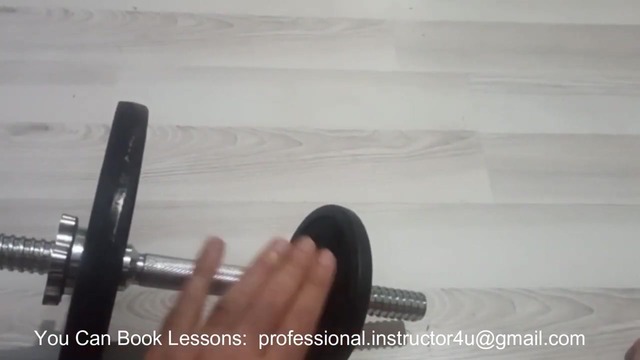 now, as you see, i have a dumbbell, but the plates, uh, they have different sizes. okay, and i'm going to push this away straight this way and we're gonna see what happens when i do so. so, as you see, it's going to travel in a circle, right, this one will travel a larger circle than this one, okay, and how big of a circle. 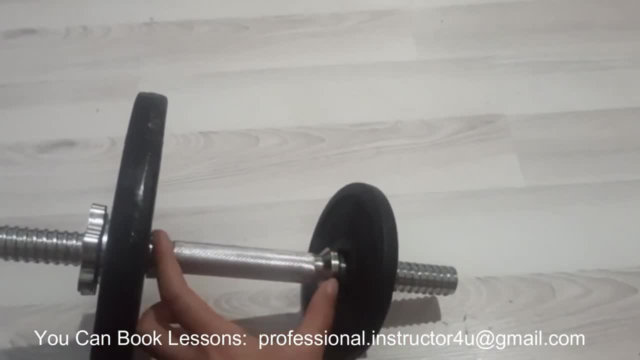 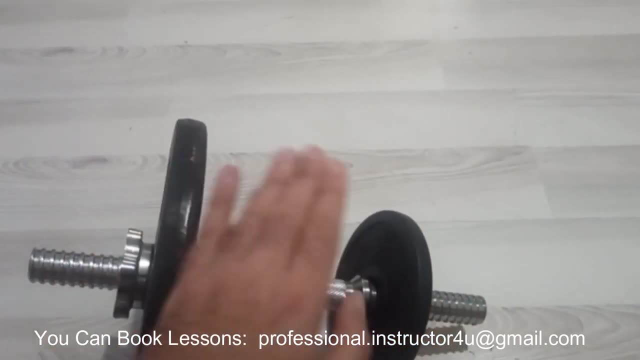 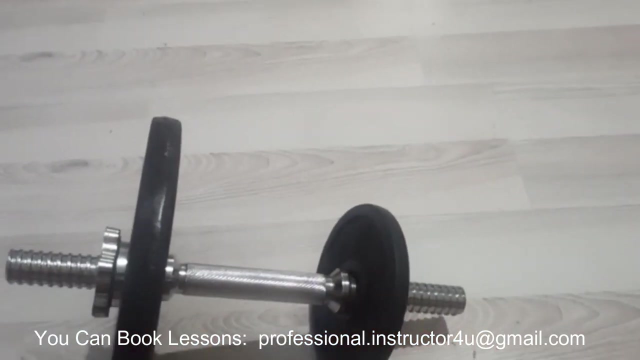 it makes. it has to do with the size of this shaft over here and also it has to do with the ratio of the wheels. okay, the closer the two wheels are. so if they are, the ratio is very close. okay, it's going to travel a very large circle, but if this one is really large, this one is very small. 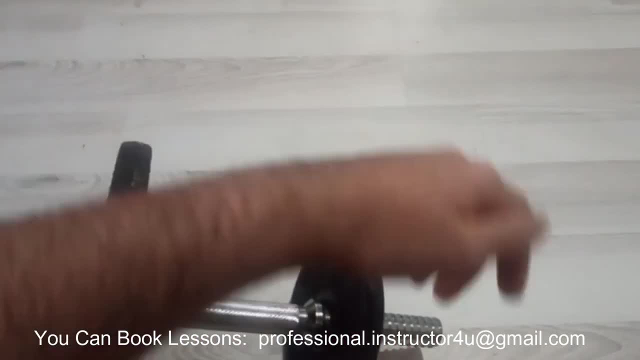 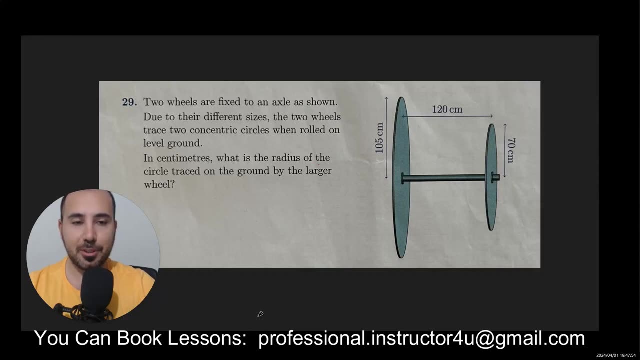 it's, it tends to actually become smaller and just go around itself. okay, we're going to do a question right, just about this one now, in this math competition question. well, they basically made the dumbbell that i showed you, that is, there is a shaft with two wheels that are fully attached. 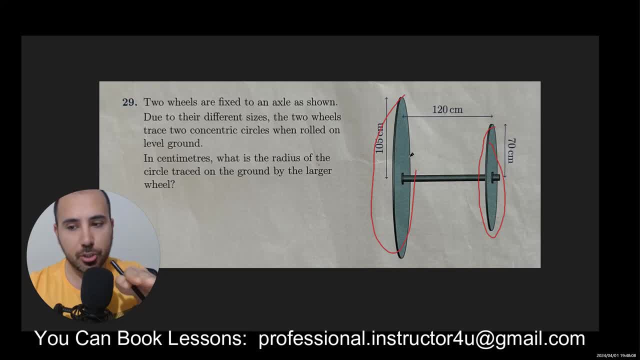 okay, and we're gonna roll it on. we're gonna just like push it forward on a level ground and they're gonna create a circle, or they're going to make two circles, okay, and that's all right. thank you for watching. right, it's going to be. there's going to be a small circle, like this it's going to go, or rather, 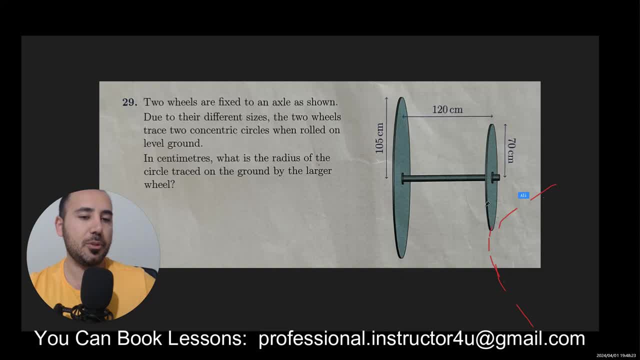 just draw it better. it's going around the smaller circle. this one will go around the larger circle and the question would need the radius of the larger circle. so- and i'm going to explain this step by step so that we fully understand this problem and we can do all similar questions- 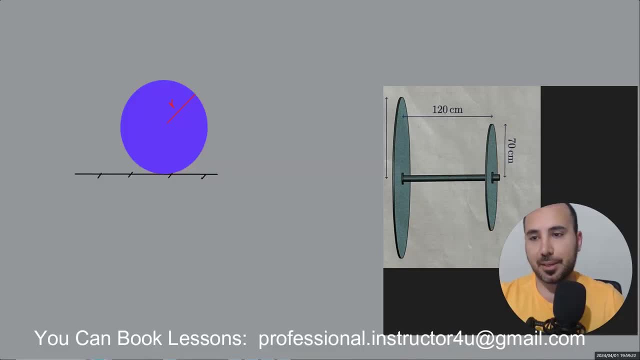 now i have a question for you. okay, imagine we have this wheel. okay, and this wheel is going to turn around itself once one revolution. does it move forward or not? the answer is: it depends. if there is no friction, like if it's happening on ice. imagine you turn a wheel on ice, it turns. 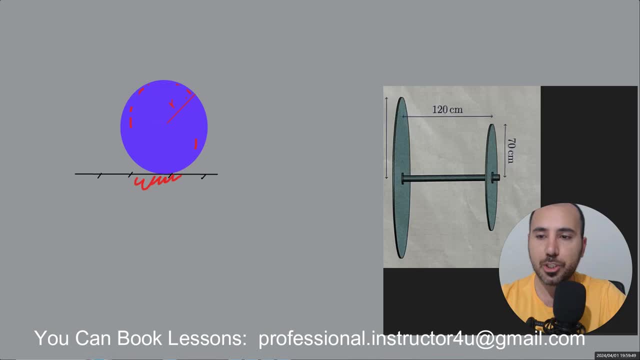 it doesn't go forward. but if there is enough friction here as it's rolling, it starts to go forward too. so after one revolution, okay, this is the same ball. how much does it go forward? what is this distance for one revolution? two pi? r if it goes around itself two times, two times. two pi? r if it rolls 10 times. 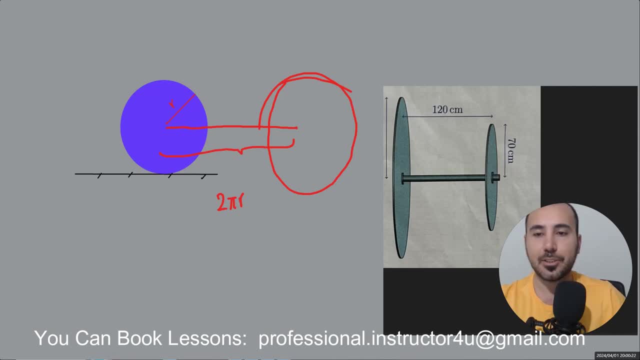 two pi r, right. so now let's focus on the question here, the dumbbell question, for example. we could call it. see, just visualize this shaft. you see they are completely connected, right, it's solid. so if this one turns, for example, 10 times around itself, okay. if it goes, 10 rounds turn. 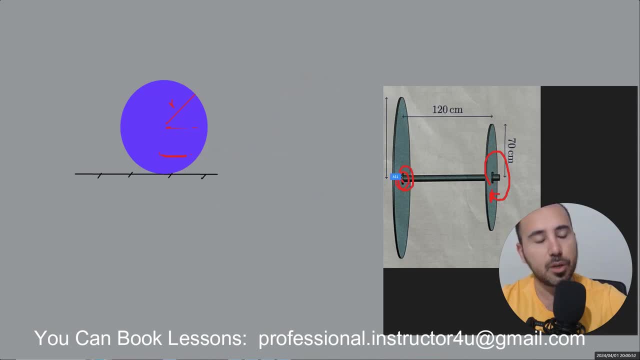 over how many revolutions? how many revolutions? this bigger one will go again: 10 revolution, because they're connected. so this small one will also go by two pi. the smaller one. i'm going to call it two pi r. this one will always go because the radius is larger. i'm going to call it capital r, this one. 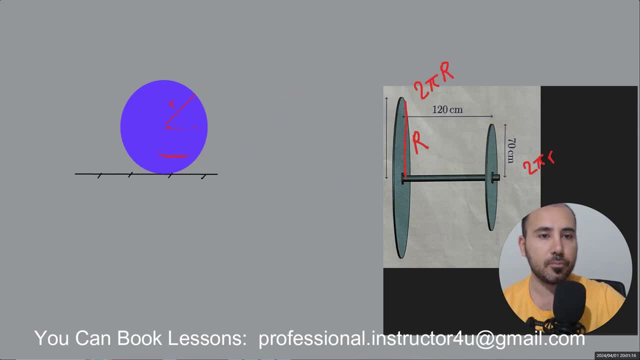 will always go with two pi? r. okay, and they're connected. so, for example, if they go 10 rounds, the bigger one will go 10, 2 pi r, the small one will turn also 10 times. so you would see how much they go. how many rounds they go is not important, because they. 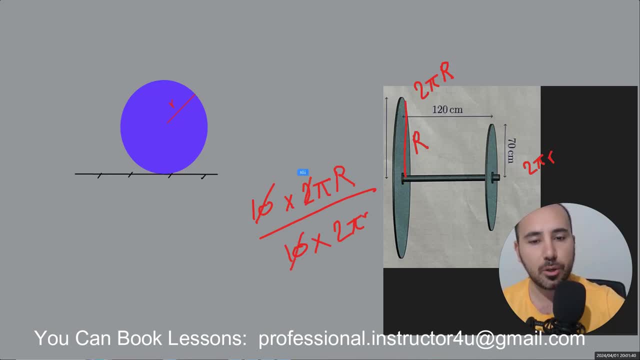 get cancelled out. 2 pi will also cancel out. so the distance this small one travels and the distance the big one travels, okay, has correlation with the ratio of the radii. so let me just write it down. so this one, let's just see, let's just write them here. i'm going to draw this circle here. 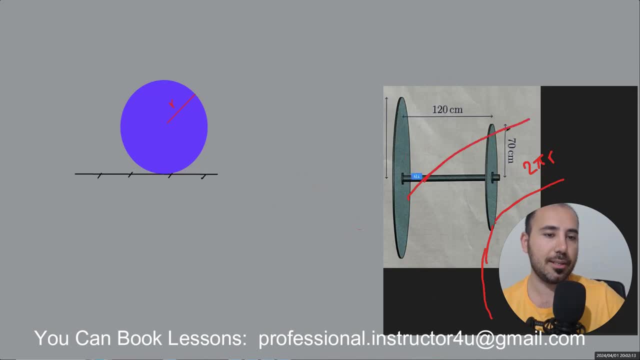 this is the small circle, this one is the big circle, so this one, the big circumference. okay, let's call this one a small c. so this is a small circumference. the big circle, the big c, right, the capital c. so the ratio of the circumferences is equal to the ratio of 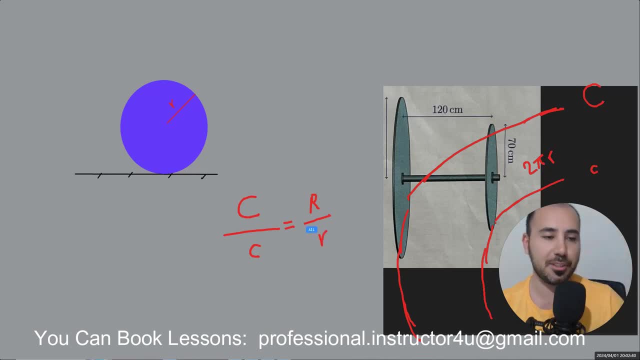 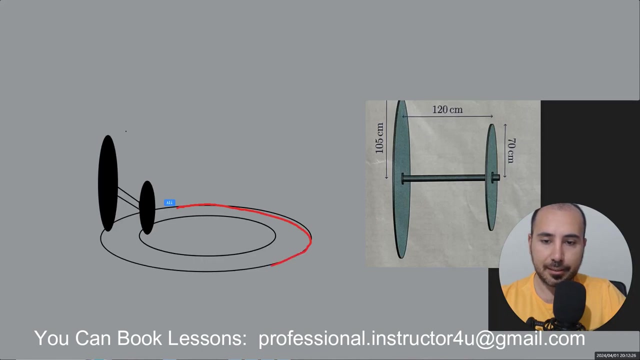 the radius, the big radius over the small radius, and this is the key. so i'm going to draw another diagram and we're going to continue this video. now, what we learned so far is this: so is that the circumference of the large circle, if i call it c? 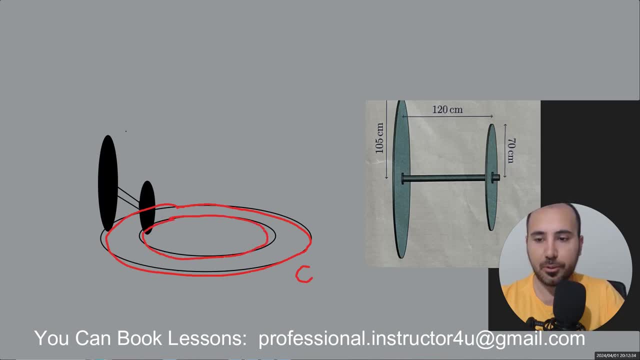 over the circumference of the smaller circle made by the smaller disk. we just learned that this is equal to the ratio of these two, so i'm gonna write it down and i'm going to cancel them. so the first one is three times 35, this one is 2 times 35. so when i simplify them is the ratio is 3 over 2. okay, and what does the question? 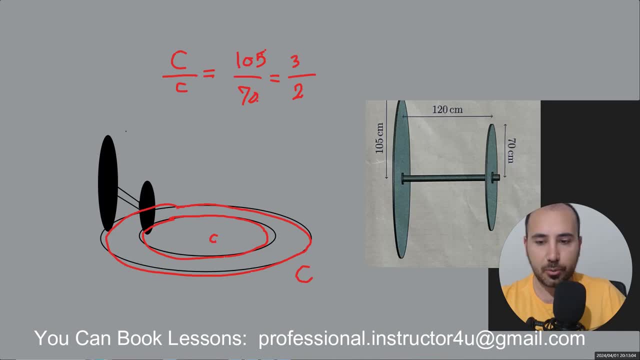 want the question needs. we need to find this one, this large, okay, radius, but we don't have enough information to find that we also need this distance over here. okay, if we have this distance over here, okay, then we have answered the question. we're going to focus on this part, so i'm going to 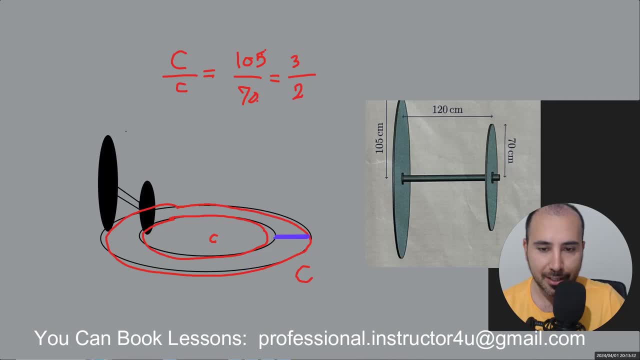 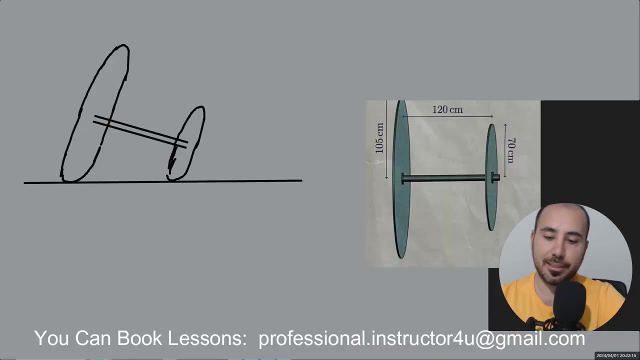 draw another diagram. so we're going to focus on this distance and then we'll have the questions completely figured out. okay, and now this is the final diagram that we need. okay, so one thing is that the shaft and the two discs- right, they're always perpendicular and they're 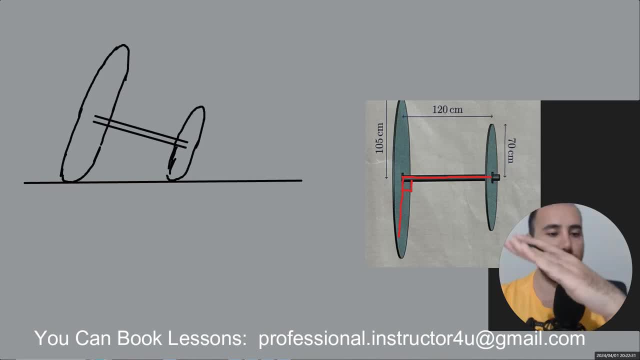 always making 90 degrees. even when they are tilted a little still, they keep that 90 degree over here. so this is the 90 degree here, and how large is the shaft is 120 degrees. so when the two wheels are tilted, okay, the distance they have is going to be more than 120.. at first the distance is 120, but once we put them, 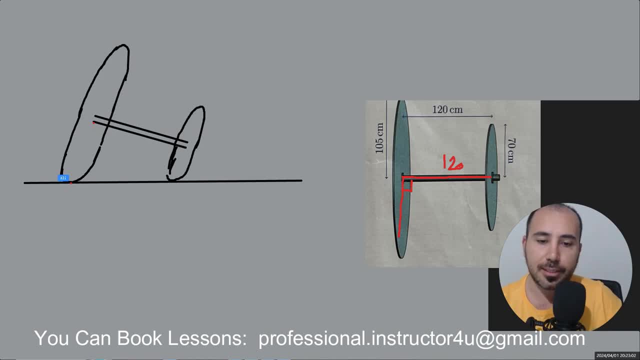 on the ground. this distance that we need is going to be more than 120.. okay, i'm going to go like here to here is going to be more and we need to find that distance. so all we really have to do is to find this distance. is you see this line over here, the red line? 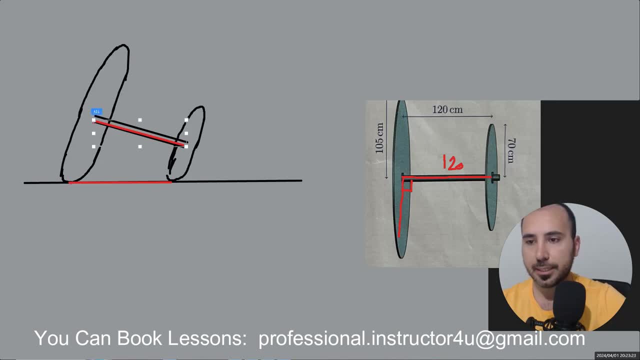 going to draw it here and i'm going to just see it's completely parallel. i'm going to just move it here this way, right over here, and now i'll have a beautiful, okay right angle, okay right triangle right over here. so this is actually 90 degree, this is 120. 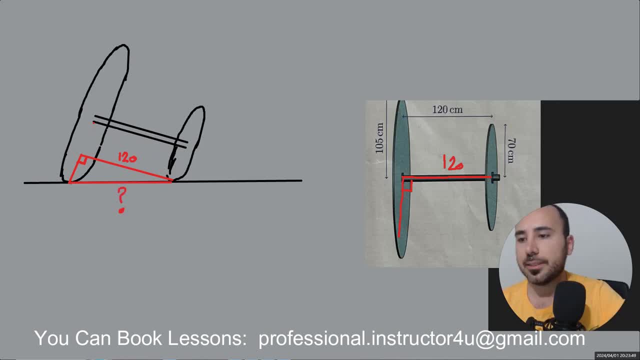 so, and this is what we need. and what is this distance? this is going to be the big r, all of this. let's just call: if this one is r, minus this one, minus this one. so from here to here, all the way is 105. so, minus this part, 70.. 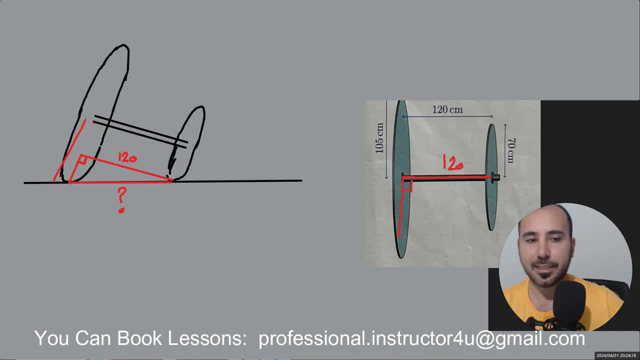 so what is this? a small part: 105 minus 70 is going to be 35 right over here. so what is the question mark? so a tip: you would never go something like this, you would never go 120 without a calculator. you never go like this. okay, we need to simplify them first. 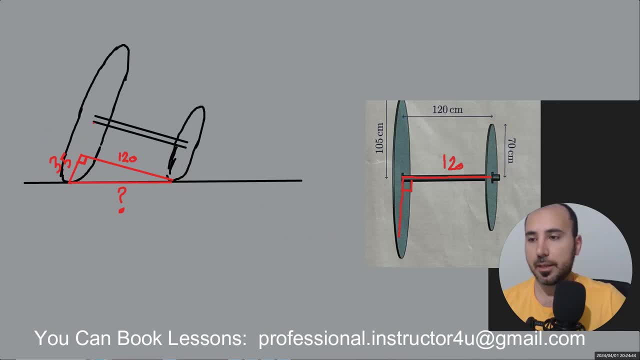 okay, and then use a pythagorean theorem, so let's just go here. i'm going to divide them both by 5.. so instead of doing this a 7, this one 24. okay, these two right angle triangles are similar: 70, 24.. so 7 squared plus 24 squared the square. 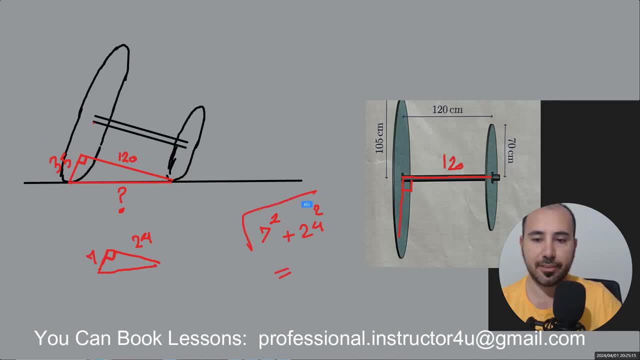 root of that is actually 24.. so the first one is 25, right so? and now these two triangles are similar, so this one. you see both of them. if i multiply this one by 5, it becomes 120.. this one, multiplied by 5, is 35. so this one. 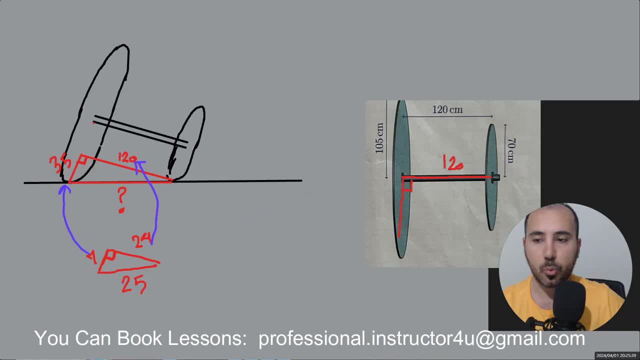 multiplied by 5 is 125.. we do this to save time, okay. so, because it's a task, we need to be quick. so this distance over here is actually okay: 125, okay, okay, and now to find the answer. we just need to use a simple replacement to find the answer. 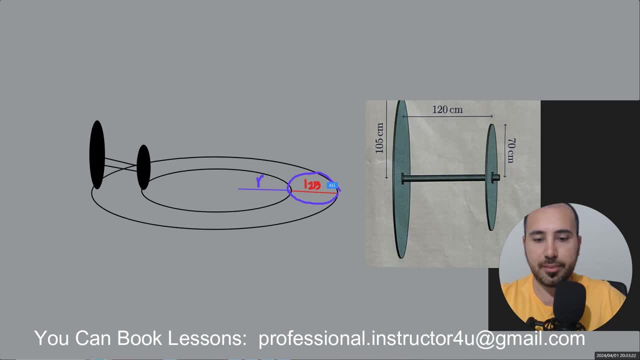 uh, the distance was 125. we just found that and the large radius from here to here is going to be the small radius plus 125. okay, and uh, we also had the large radius over the small radius. okay, is the same as the ratio of the big circumference and the small circumference which we had. it was three over two. 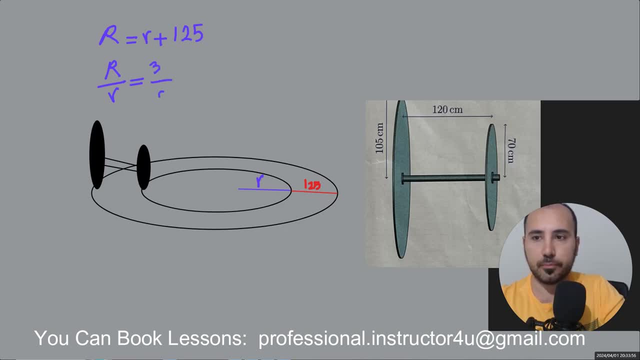 so i'm gonna go like this and we're going to replace, instead of capital, r, i'm going to write this: so we're gonna have r plus 125 over r is 3 over 2, 3 halves from here i'm going to cross multiply. 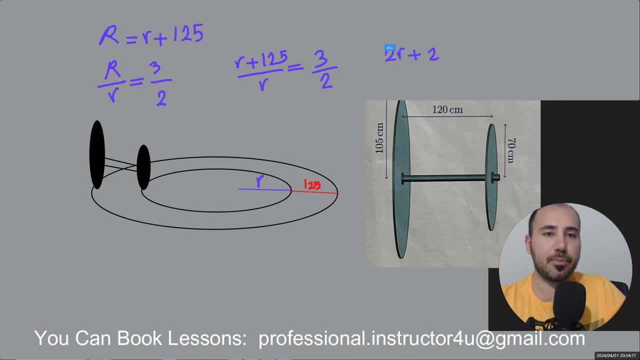 so i'm going to have 2r plus 250 is equal to 3r. so from here we're going to have r is equal to 250.. So this small r is 250, but the question is asking us for the larger r. so from here to here. 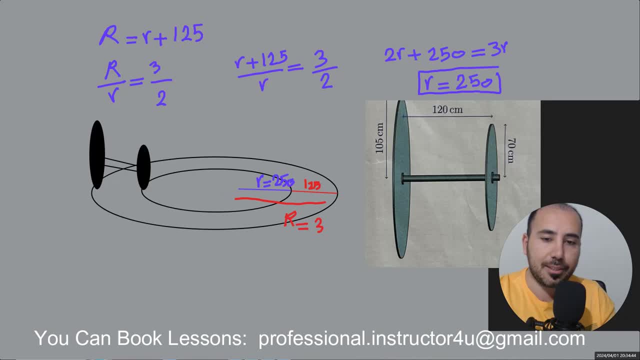 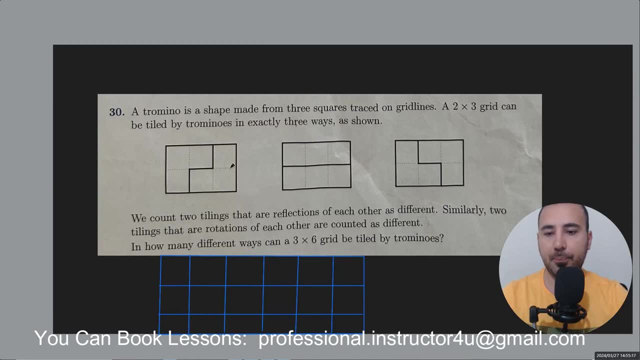 so the answer to the problem is 375.. Welcome back to Mathics. In this video I'm going to do this math competition question. The question is asking us to tile this 3x6 grid only using trominoes, and trominoes are three squared trace on the grid line. so for example, they could be like: 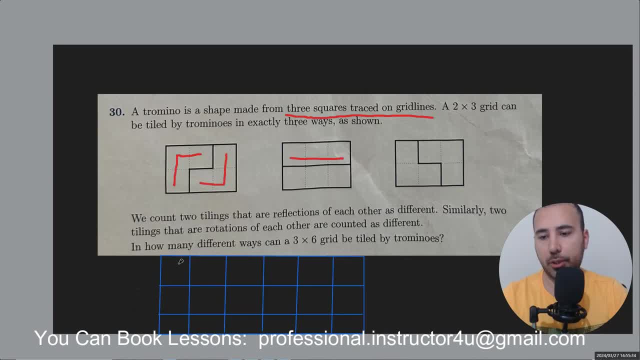 this like this, horizontal or completely vertical. so, for example, I could tile this grid, maybe like this: okay, so how many ways are there to tile this 3x6 grid? so I've done a lot of different ways. the one that I think is the best is called recursive tiling and we're going to learn that through one example. and if you have, 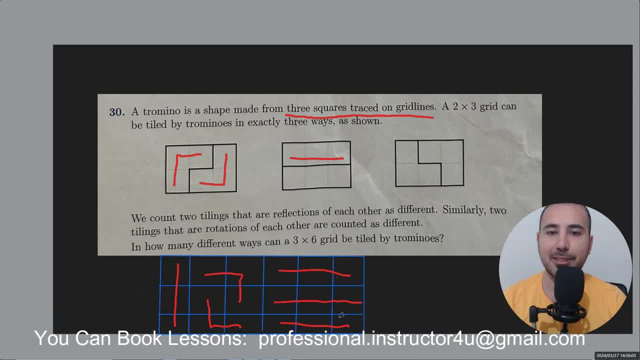 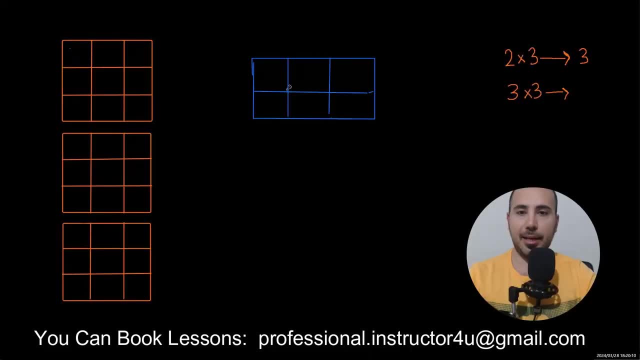 never heard of it or you don't know how to use it. this is the place to learn it. okay, let's get started. Okay, in the example we just saw that a 2x3 grid can be tiled in exactly three ways. maybe like this, maybe like this two and number three. so that's why I wrote it here. a. 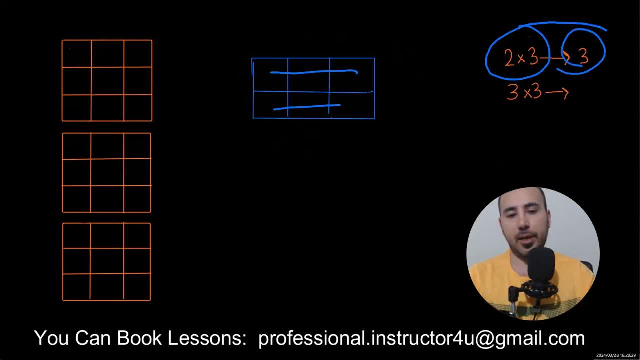 2x3 grid- okay, can be tiled in three ways and we're going to focus on a 3x3 grid, okay, and we're going to use recursive tiling. why is it recursive? because when we're going to do 3x3, I'm going to 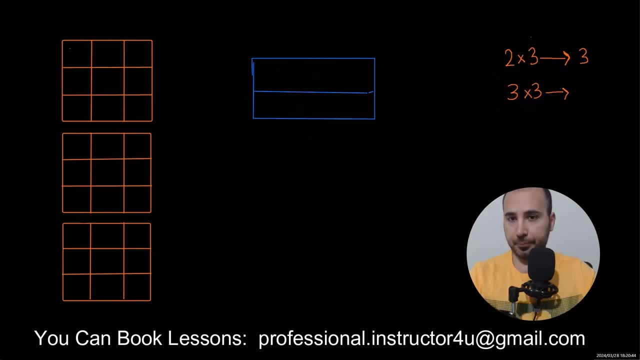 use that previous information. okay, and how do we start about this recursive tiling? we're going to start from the top left corner. you could also go this one, this corner, just fine, you just choose any of them and ask yourself this question: how many ways can I just tile this square? only, okay. so how many ways can we do that? 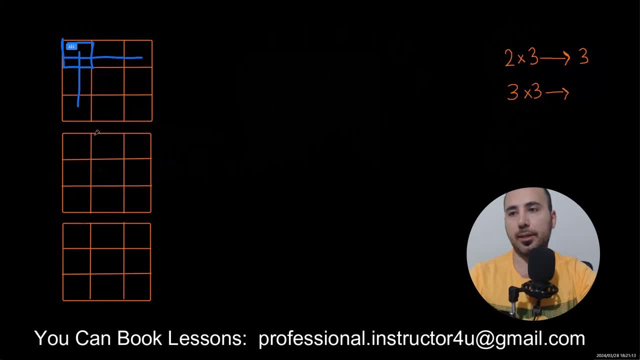 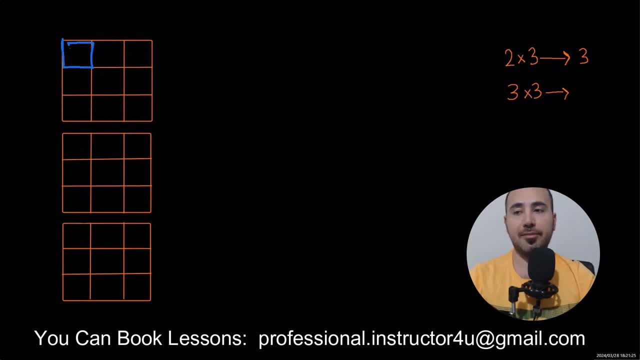 the top left corner can be tiled in five different ways, so I'm going to write them like this: maybe horizontally, maybe vertically, maybe something like this, maybe something like that and lastly this one. as you see, they're going to be five different ways of tiling them. let me just write: 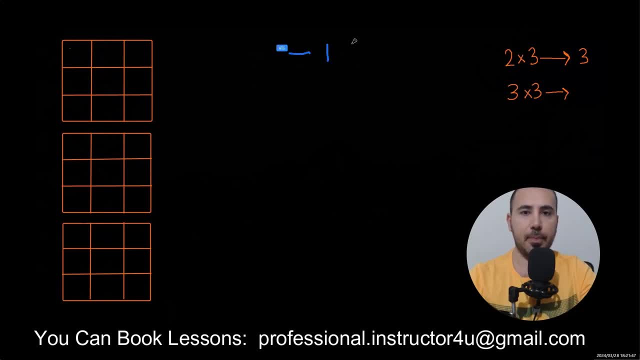 them little to the right, because I'm going to need that space later. so it's going to be like this, like this and like this, and we have to divide this question in five different cases. okay, it's going to be easier than you think. once you do a few, then you get a hang of it and you become quick. 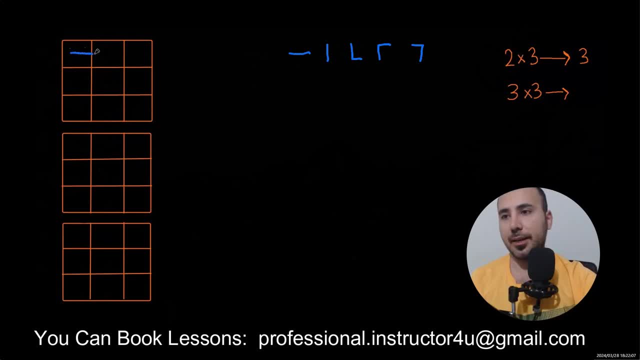 so if the first one is tile like this, what is left is a two by three grit. how many ways can I tile this? recursive tiling, I know, is three, so I'm gonna go and write a three here. so what if it's going to be completely vertical like that? again, a two by three grid is. 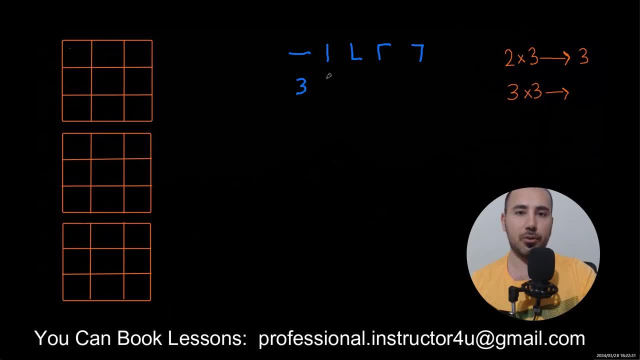 left? how many ways? again three. so we see, we're just gonna write them down like this. if I'll start by L shape something like this: okay, so what can fill this part? there's only one thing that can fill this, so only one way for this one. 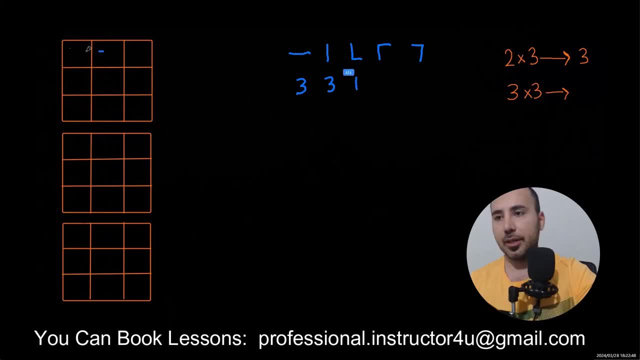 right if I start like this: ah, now is the the tricky part, so let's focus on this one, this tile. how many ways can I tile this part? it's gonna be two ways. maybe I could go like this, or maybe I could go a horizontal like this. so it's gonna create. 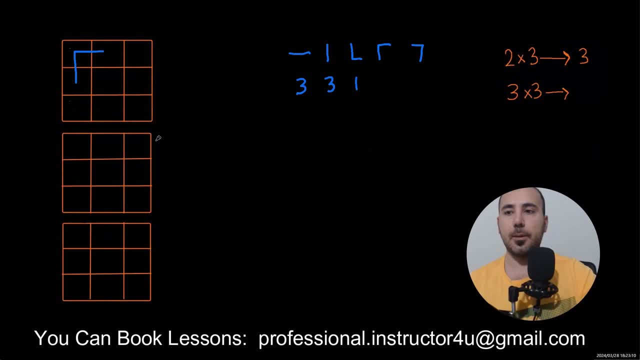 two cases, maybe something like that, maybe something like this. so with this is start, I'm gonna have two, so I'm gonna write it here. so two ways for this, and if I start like that, there's only one way to complete this. right, it's gonna be this one and then this vertical, so one. 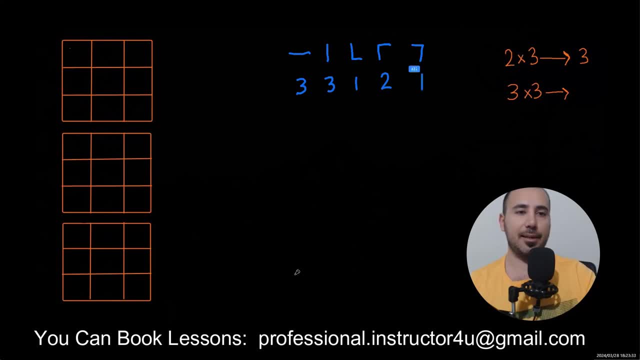 way. so a three by three grid, okay, can be tiled in: exactly three plus three plus one plus two plus one, right? but we're gonna use this, this, this until it right, and I'm gonna go ahead and this, right, and that will be a straight grid, but we're gonna go ahead. 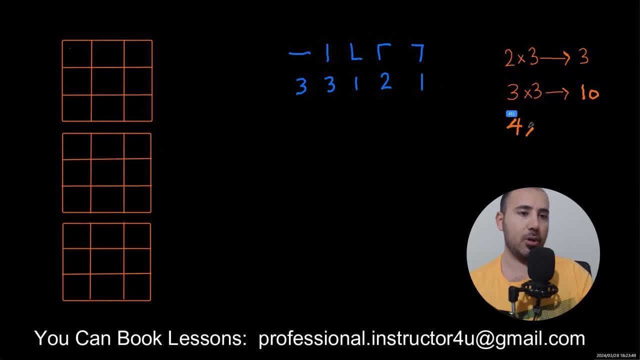 and do this again, and so that's what we want is: hook, collect the 저기, read this and then, sotto, look in the weeds. we're going to want to use so a terribly large grid for things like this is what we're going to want. this is our think. 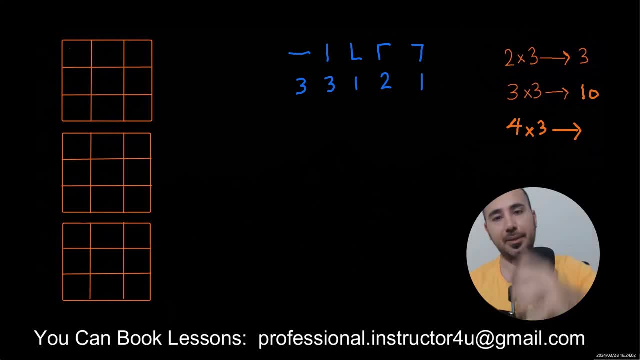 about is to say, into this grid we need to say like: sorry, so we get that in PSA, sir, don't worry, there's a little bit more detail after that, which will one really look slightly different to, I'm sure. but anyway, this is a way to end it. 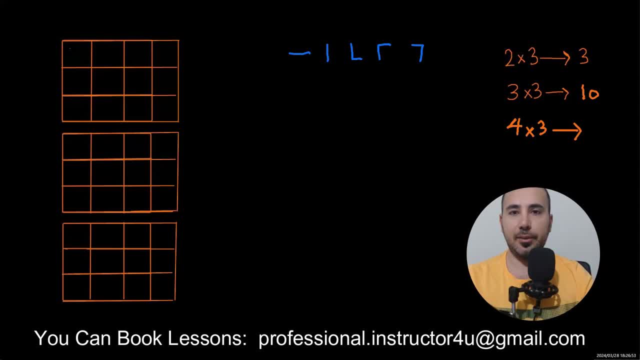 okay, and then I'm gonna go and I look at this grid and I see the little armour, but there is this one. so I'm just going to want to Spell them all, one letter per. to repeat the same process for a four by three grid. what if we start by a horizontal line? okay, 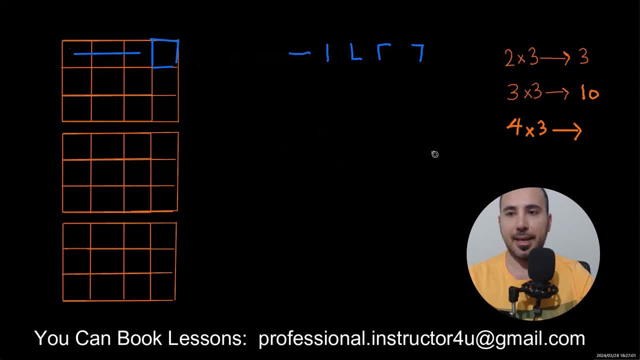 and now let's focus on this. ask yourself this: how many? what ways can i tell this specific square? the answer to this will be two ways, right, if i go the first one like this, the next one, maybe i could go a vertical like this or i could go something like that, right, two ways and nothing. 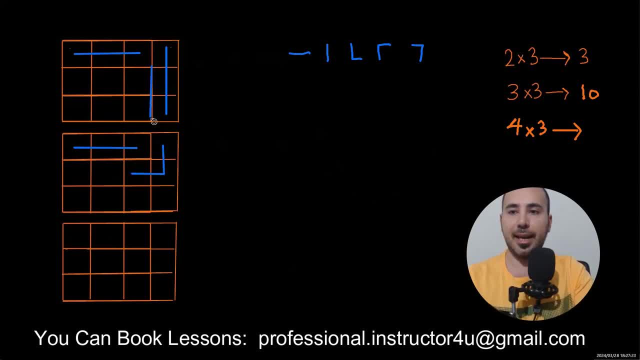 else. look again: when i do it like that, i have a two by three grid. so how many ways can i tell this again? three ways. so this is gonna give me a three. i'm gonna write a three like this: now that i have this one, okay, these two that are left here, uh, let's see, maybe i could fill it like this right. 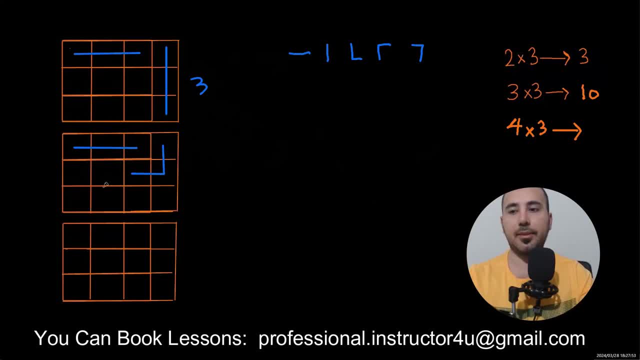 and can i fill it like that? no way, i can't do that. so these two are going to be, um, not like this, only like that. so the only way is going to be this one right here, and it's going to be like this. so this is going to be only one way. so, if i start, 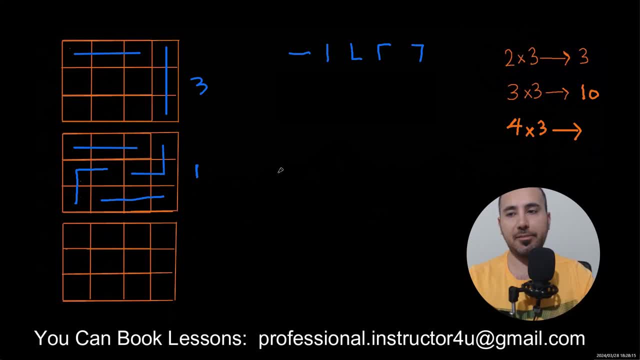 by a horizontal line. there's going to be only four ways of tiling this grid, so i'm going to go four. and if i go with the vertical, the answer is very easy: what is left? a three by three grid. do we have it? yes, so it's going to be a 10.. so this one? i'm going to write this one as three plus. 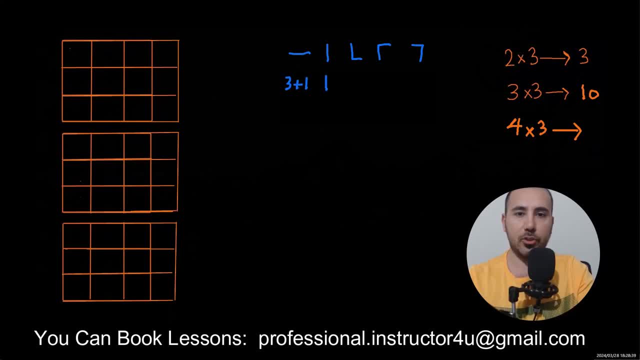 one, the vertical one. i'm going to write it as 110.. now, what if i start by something like this? if i start by this, then you need to ask yourself: can i fill this? how can i tell this a square? there is only one way. there's only one thing. 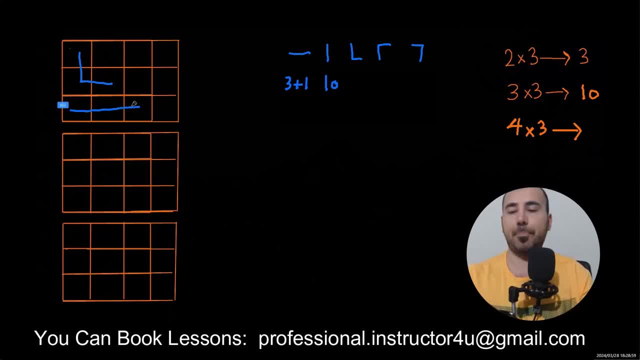 that is long enough to fit there, so it's going to be this one, right? so for this one, for this particular square, there are actually two ways. maybe i go like this. that's one way, or maybe i go horizontal and do it like this, so it's going to be only two ways. so if i start like 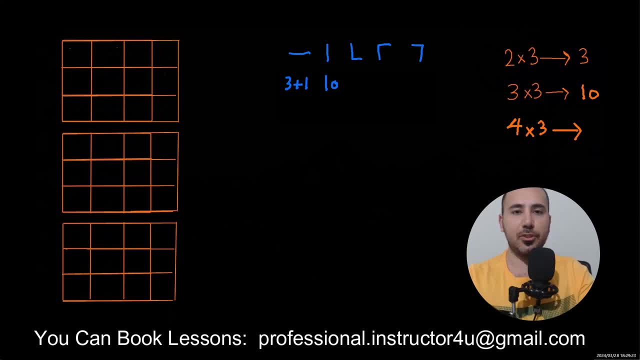 that. okay, the answer is going to be only two. if i start like this, let's go and analyze this one. so let's focus on this. there's only two ways of tiling this. maybe we could tile it like this. maybe we tile it this way. if i tile it this way, this is a. 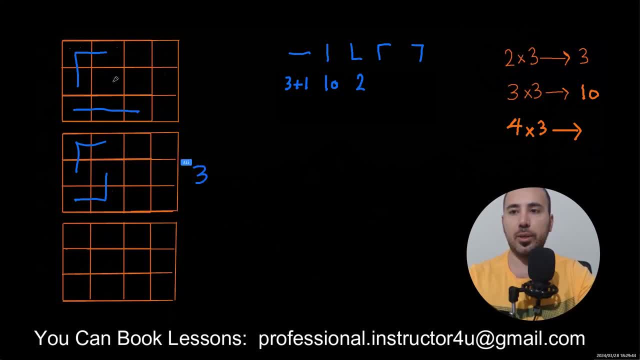 two by three grid. it's going to be three ways, and with this one, uh, let's see with this one, how many ways can we fill this? it's going to be only like that. so only one way, right? so if we start with this, it's going to be a three plus one. again, i try to write it, this one, i'm, i'm not going. 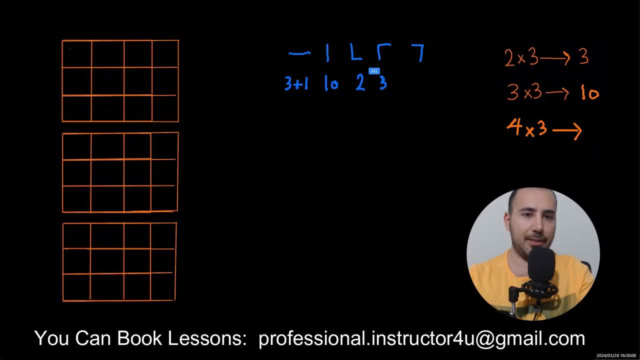 to write it as four. rather, i'm going to write it as three plus one. the reason i write it at three plus one? because this is this three over here that is being repeated. okay, and lastly, what if i start this way? okay, then this one. there is only one way to do this. a two by three grade is left, which is going: 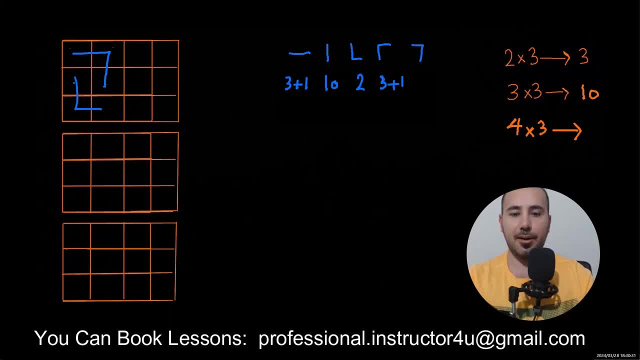 to give us an additional three, so i'm gonna go write another three right over here. so let's add up all of these things together: a four of four and a ten twenty. it's gonna be a total of twenty three for a four by three grid. okay. 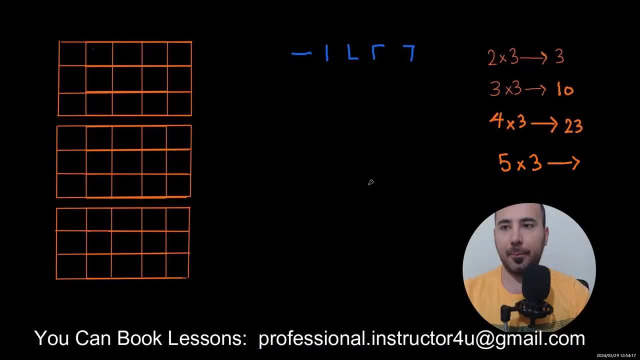 okay, let's go and repeat the same steps real quick. okay, if we start with a horizontal one like this? okay, so we have to focus on this square and ask ourselves: how many way can i, uh, tile this square? this would be one way. okay, this could also be another way. 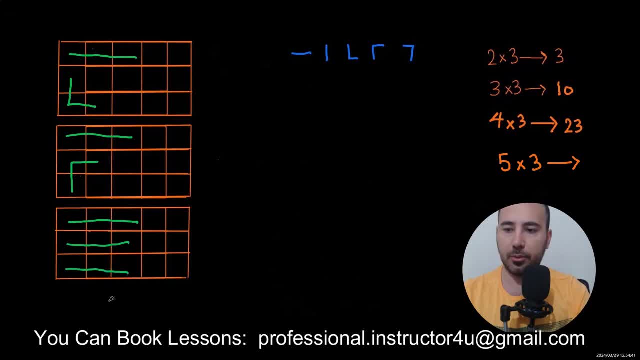 or this particular square could be tall with three horizontal trominos. so, okay, it's gonna give a three, three cases, this easy pc, because there are three ways to tile this one. so this one is three. i'm going to clean it, so i'm gonna write the three though. 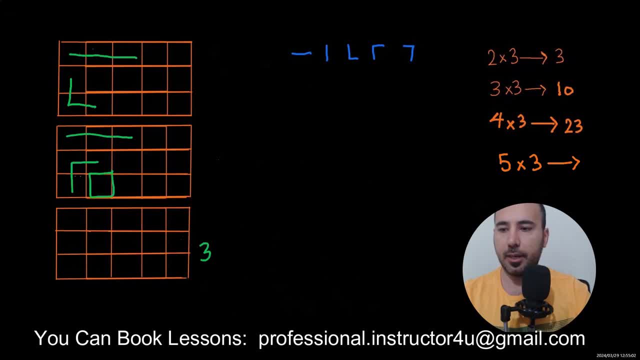 so here for this one. this square is going to be tiled in exactly two ways. if i tile it like this, this is gonna give me a three. okay, and if i tile it like that, i think everything else will be forced, because this one has to be like this and like that, so this one will also give us a. 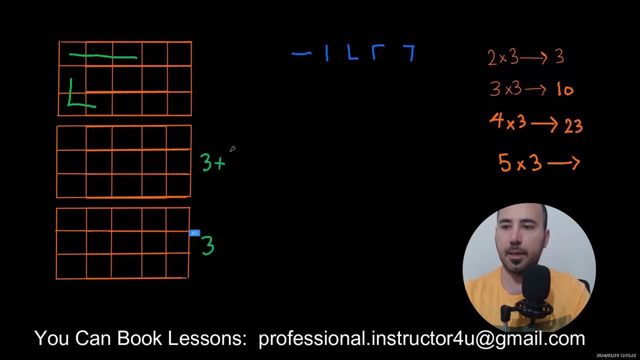 this one was a three. this one was a three plus one. and again, we have two ways of tiling this. maybe if i tile it like that, it's gonna give me a three. if i tile it like this, okay, this one will be forced and this one will be four. so the first one is going to be three of this. 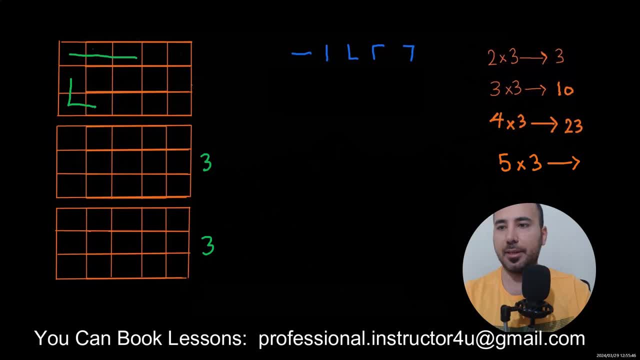 and two extra. so i'm gonna write it here. let me clean everything. it's gonna give us a three times three and then an additional two. okay, if we start with a vertical trauma now, a four by three grid will be left to tile, and we already have it here. so this one is the easiest. so we're gonna have a 23. 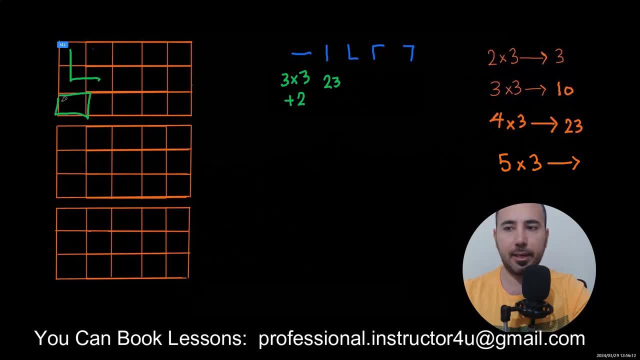 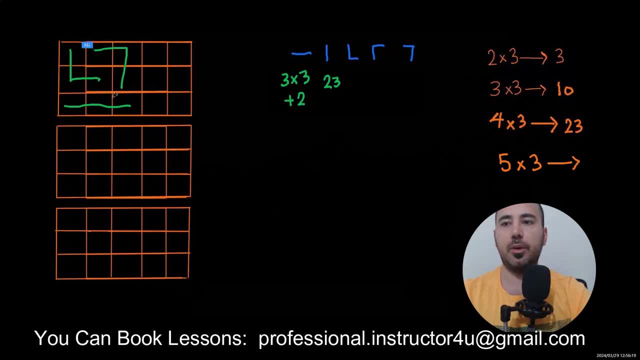 now, for this part, is there only one way? no, there are two ways. if i tile it like that, it's gonna give us a three, as you see over here. okay, and if i tile it this way, it's gonna give us something like this: so all of this is going. 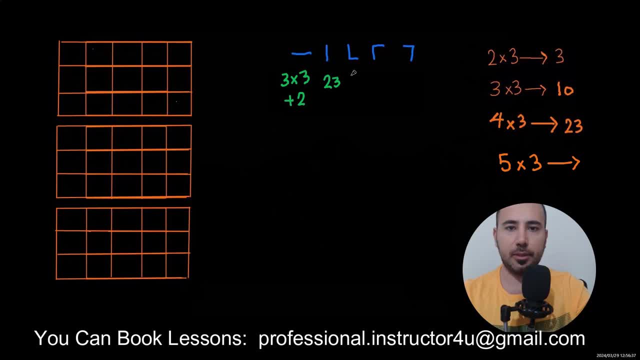 to give us a three plus one, so i'm gonna write it here at three and a plus one. now, if you start with this, this square can be tiled in exactly two ways, maybe like that, maybe like this. so this one is easy, because it's going to give us 10 ways of doing it, and this one 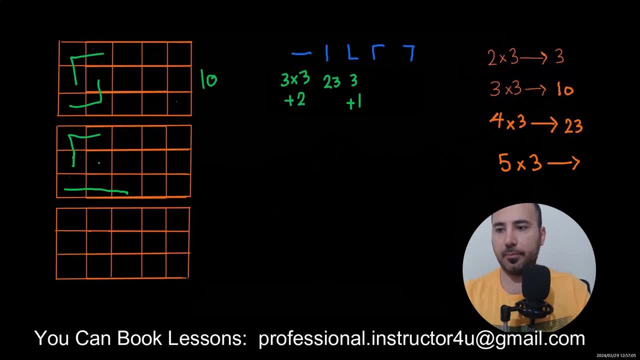 if i go like that, it's going to give us a three, and if i go with the horizontal tromino, this will be forced. this will be forced. so this one is a 10 plus a 3 plus a 1.. so let me write it here: a 10, a 3 and a 1.. 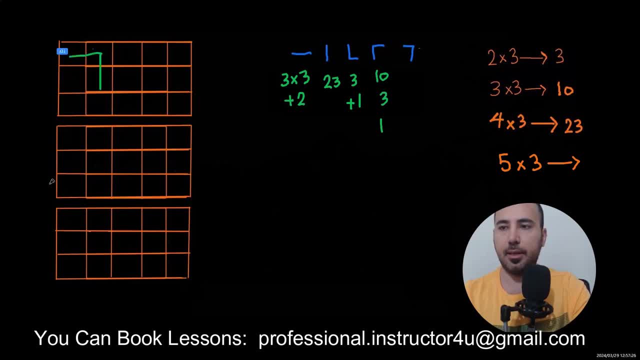 so now, if we start with this- this is also easy because this will be forced- a 3x3 tromino is left only 10.. so you can see that there is definitely a pattern. this one will just go with the previous one. okay, if you start with the shape like this, a tromino like this, it's going to give like that. so 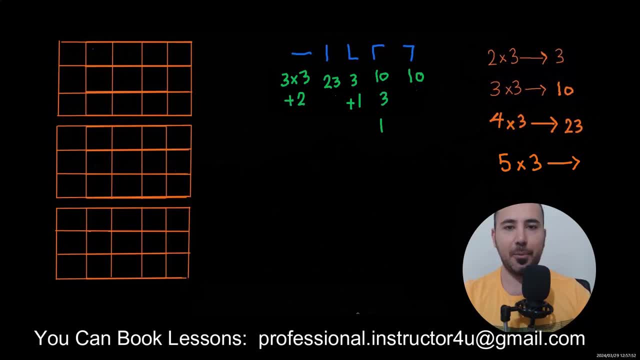 we could clearly see how they are actually being repeated now, so we just need to add them all together: it's going to be a 23 and it's going to be two tens. right, i'm going to just write that as 20.. it's going to be five times three, like three, three, three, three. it's going to be a 15.. 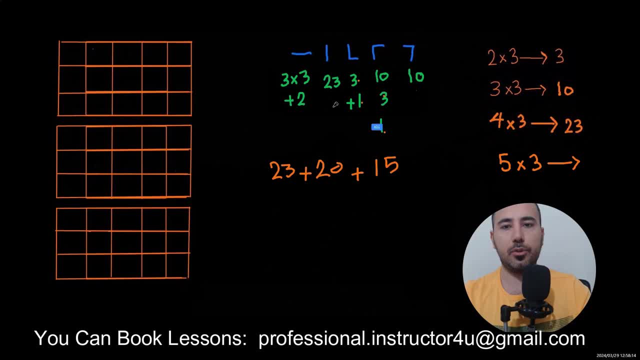 and there will be some extras: one, two and four, see okay, and just we just have to add them all up. this is going to be 53, 58, 60.. i messed up 43, 48, 58 and 462. okay, and you could see the pattern now if you want to do programming. 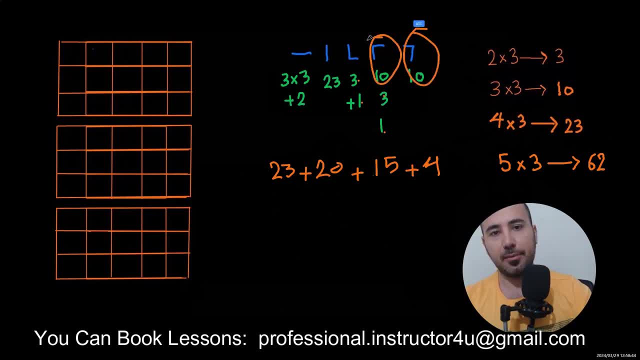 uh, then you have to just do each one individually and sum them up. okay, now we just have to do one more. okay, now let's go and do this one last time for a six by three grid. okay, we're gonna focus on that. so if i start horizontal, with the horizontal trauma now, as we saw before, 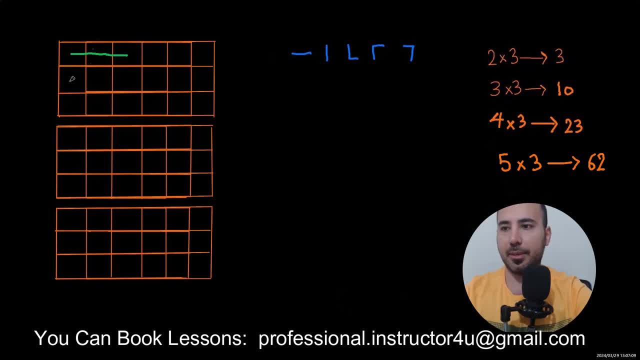 this square, uh will, can be filled and tied in three different ways. okay, maybe like this, maybe like this. okay, so the first one is easy, because uh three by three is left, so it's just gonna be a 10.. now this one, remember, this square can be, uh tied two ways. this is one way. 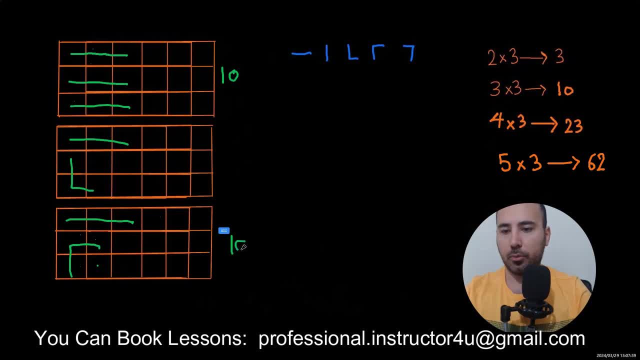 so it's going to give us another 10, or we could go with, uh, something like this. i could go with a horizontal one, like that, and then for this one we're going to have two ways again. if i go like this, it's going to be a plus three. if i go with the horizontal one, it's going to be only. 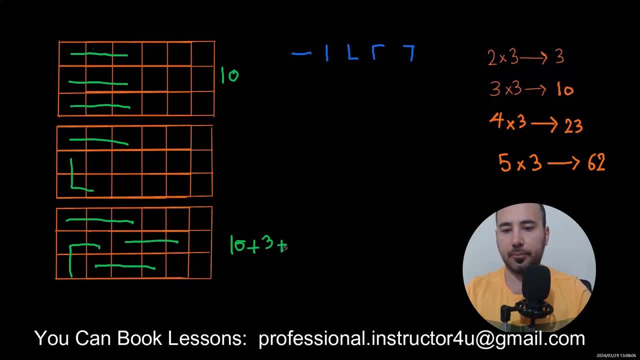 like this and only like this, so everything else will be forced now the the middle one. so we have to be careful here. this one could be done exactly in two ways. if i go like this, again, another 10. if i go with the horizontal one, this one will go with the horizontal one too, but this one. 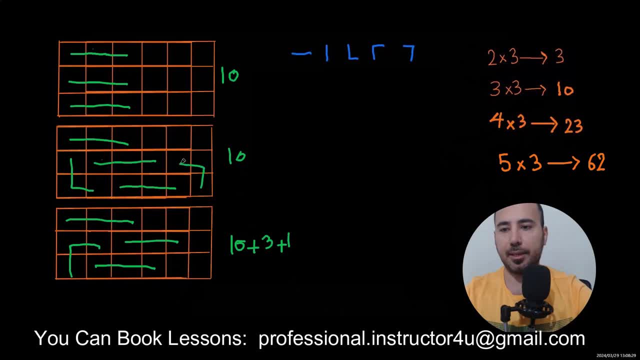 this can be exactly tiled in two ways, maybe like this, maybe like this. so it's gonna give us as an additional 2. okay, so we just have to add all of these, so it's gonna be 3 tens and 1, 3 and again 2 plus 1. so let me just go and clean everything here to. 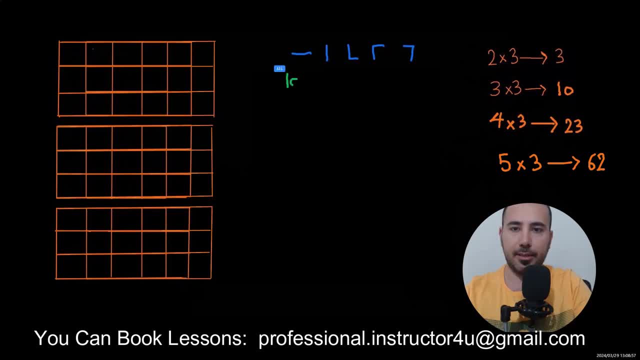 prepare it for the next round. so was like a 10 times 3. okay, there was one of the previous one of 3 like this and there was a 2 and a 1 individual ones that were added. so if you start with a vertical one, it's the easiest because 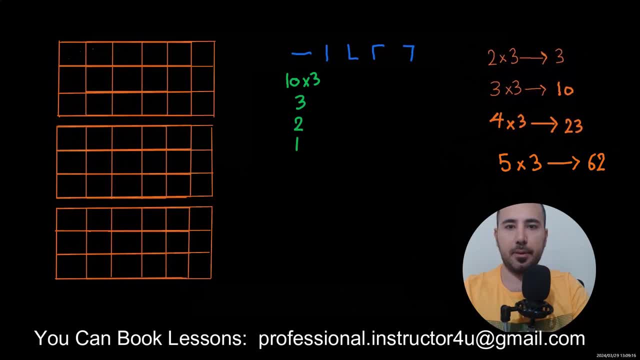 it's gonna be just a 62, the previous number. I'm gonna write a 62. if you start with a shape like this, then this one, as we saw before, will be forced. this one is gonna get 2. if I go like that easy, it's gonna get us. 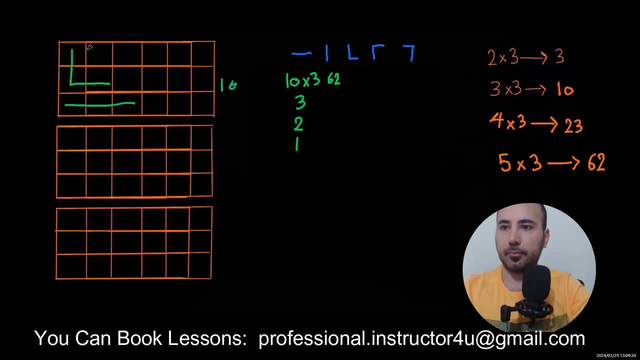 up 10. if I go like this, okay, for this one again, we're gonna have two ways. if I go like that, it's gonna give us a 3. if I go with the horizontal, this one has to go. this one. so a 10 plus a 3 plus a 1. okay, so this one is gonna get us a 10, a 3 and 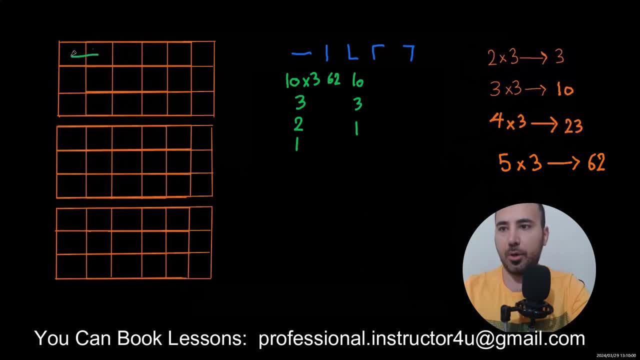 a 1. so we have one more. one is tricky. we have to be careful. if i go with this, this one can be tall exactly two ways, maybe like this, maybe like this. if i go like that, it's easy, a four by three grid, it's gonna give us a 23. 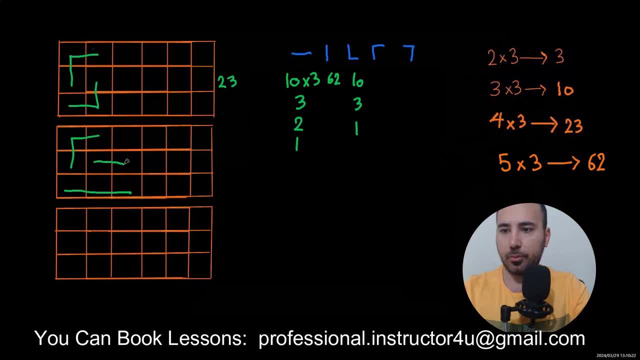 okay, if i go like that, again we're gonna have to. if i go like this, it's gonna give us a 10. and if i go horizontal like this, this one. if i go horizontal- yeah, i did like that- if i go like that, it's a 10. if i go like this: 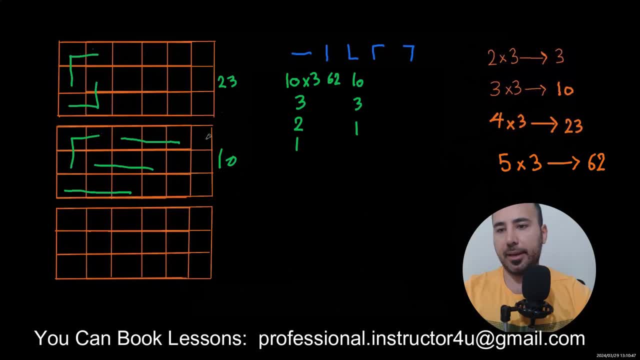 then this one will also be forced. so from here we have to be careful. this one could be tiled in two ways, maybe like that, maybe like this. so it's going to give us an additional two. so 23, a 10 and a 2.. let me go write it: 23, 10 and a 2.. and lastly, this one is easy. 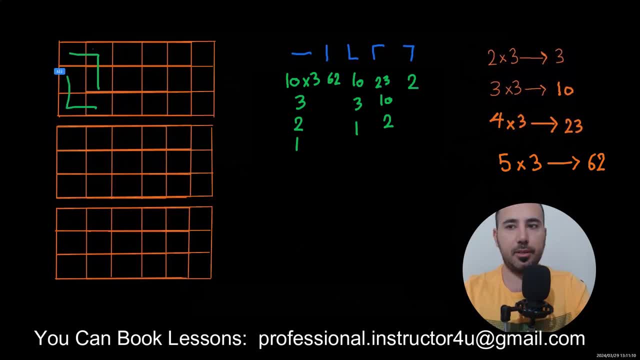 because this one will just be and it's going to give us another 23 and it's going to be all of it. so let's see here. uh, this will help us to see the big picture of how each one is being repeated. again, we're going to have one of the previous ones.